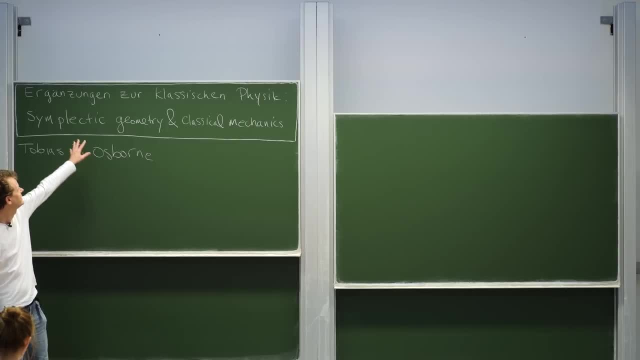 So we'll see, hopefully by the end of this course, that symplectic geometry, that even quantum mechanics can be thought of as a symplectic theory. So that's why we're going on this journey, Because it's the mathematics that underlies so many of our physical theories. 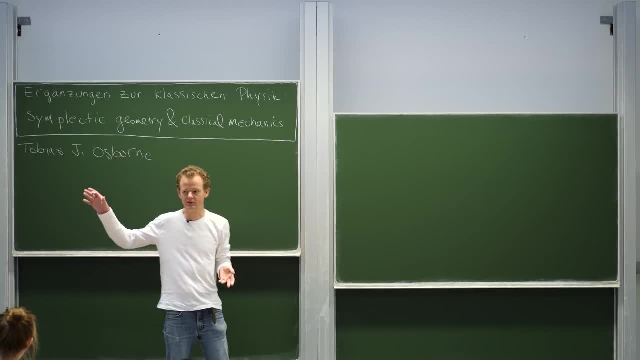 And then when you see this unifying mathematics, then it allows you to transfer ideas from, say, geometrical optics all the way through to quantum mechanics and vice versa. So this is a very powerful toolset that we're going to learn and we're going to gain huge insights into the structure of physics. 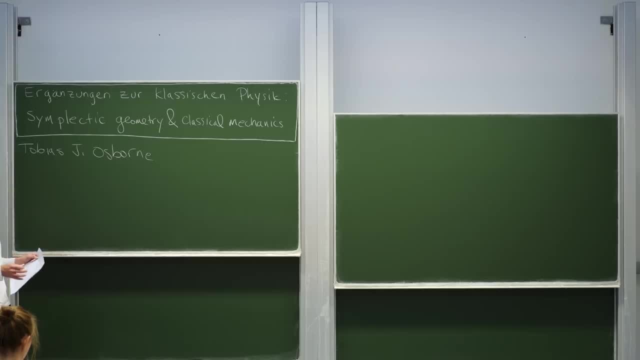 Now I suppose, before I get into any part of the subject material, we'll cover the most important part of the subject material. We'll cover the most important part of the subject material. We'll cover the most important part of the subject material. 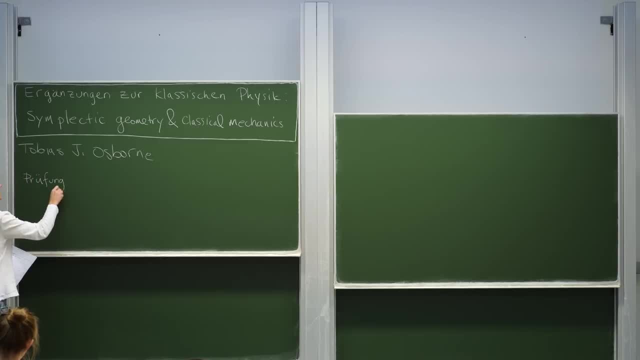 And also we'll cover the most important questions, And so this is a quite a massive team of� question, but we'll still cover the most important questions. j 等, v. If you want the Prüfungsleistung for this course- that will be an oral exam- just contact. 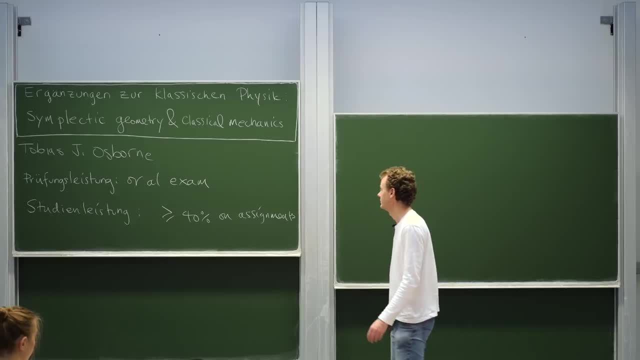 me for an appointment. If you want the Studienleistung for this course, then you need to achieve greater than 40% in the assignments. There will be six weekly assignments- there might be five, but I believe we'll set it at six weekly assignments that count for the Studienleistung. achieve greater than 40% on. 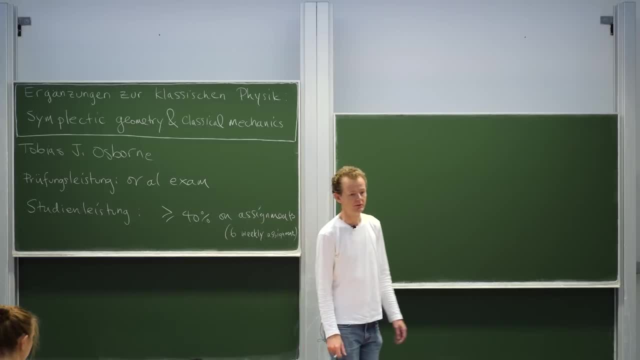 those and you get the Studienleistung for this course. For the viewers who aren't in this course, The problem sheets, I will distribute them on my blog. you can find them on StudIP, but the solutions will not be distributed. 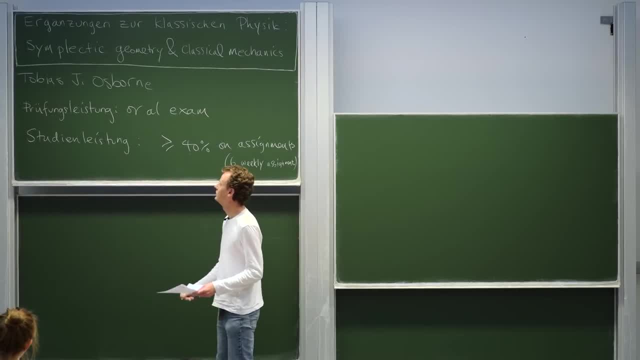 So that's the important stuff. if you want to get the marks for the course Now, when can you even sit in this course? Well, you're welcome to sit in this course whenever you want, but I'm going to assume that you know what you're doing. 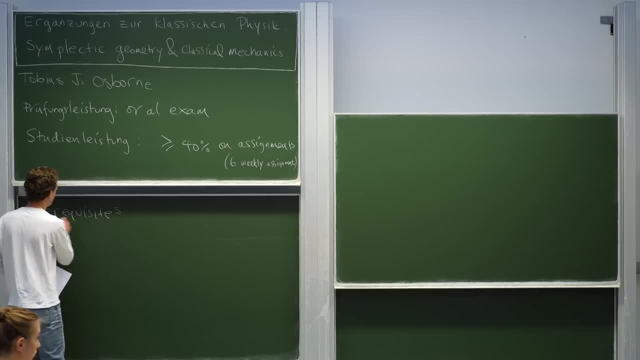 You know some stuff, and if you don't know it, then either please go and learn this stuff pretty quickly or accept that it's going to be a little bit require a little bit of background reading as the lectures go. So we're really, really, really. it's an absolute, fundamental prerequisite for this course that 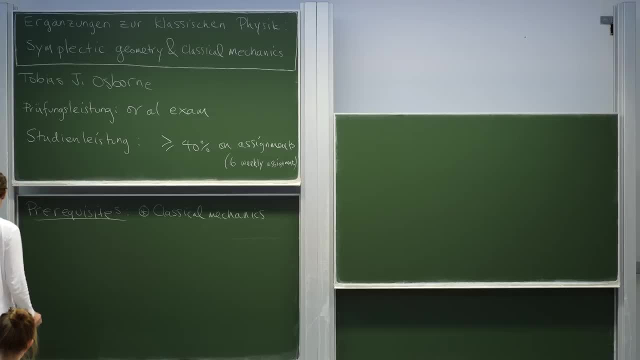 you know classical mechanics. you all do. I know this- And in particular, I want that you know what on earth is a Lagrangian. I want that you know the extremal or variational extremal principles. I want that you know what a Hamiltonian 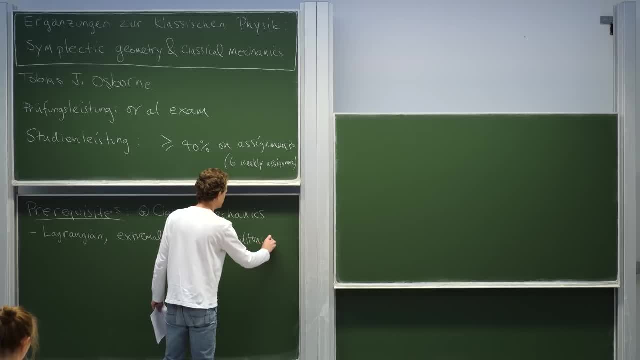 is, and Hamilton's equations And Poisson brackets. So as long as you've seen those words in your classical mechanics studies, then you should be good. There shouldn't be any difficulty in the physical background. There is a little bit of mathematical background in this course and that is I'm going to. 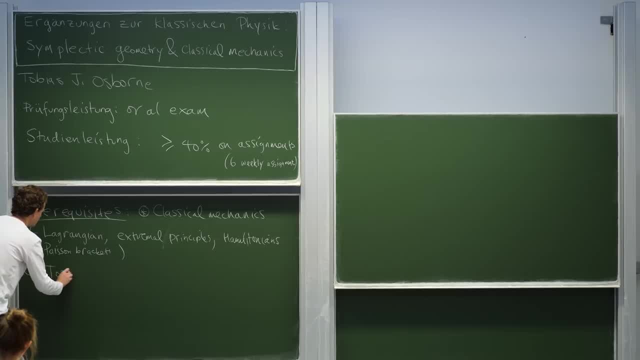 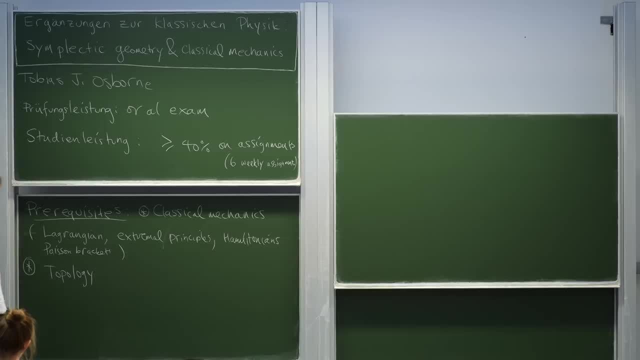 And if you don't, then you're willing to go and look these words up. So, open, closed, compact, continuous and homeomorphism- these are the only words that we'll probably use in this course. so these words will appear and, but don't be too afraid, I 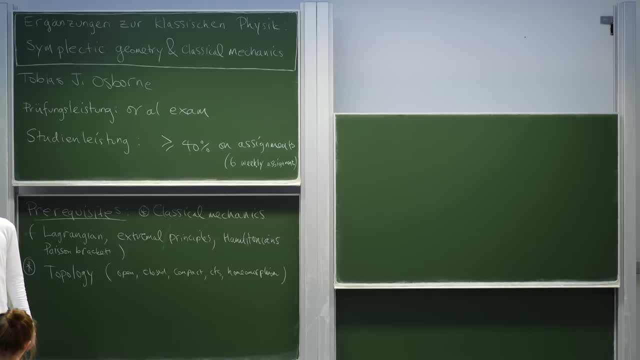 mean the first lecture. this is going to be a real drudge. the first lecture. we're going to have to just toil through some definitions before we can get really started in this course, and that may look a bit off-putting. we're going to use a. 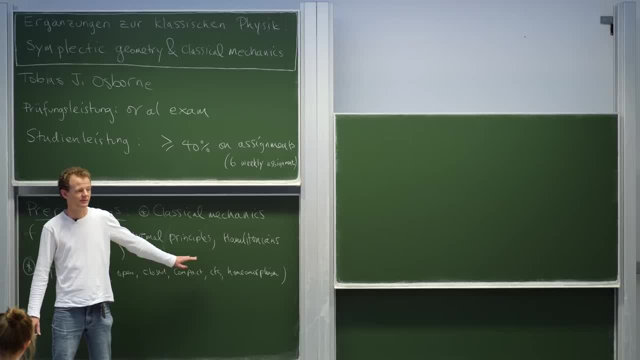 lot of these words in the first lecture, but the beauty of physics is that physics isn't about general mathematical theories, it's about examples, and as the course goes on, we'll focus more and more on examples. I mean wide classes of examples, very important examples, but nonetheless, we, it turns out, we will. 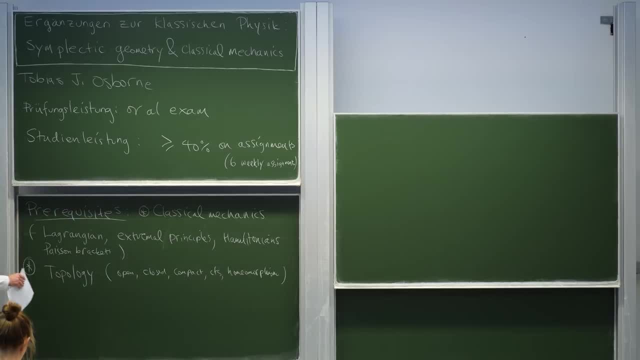 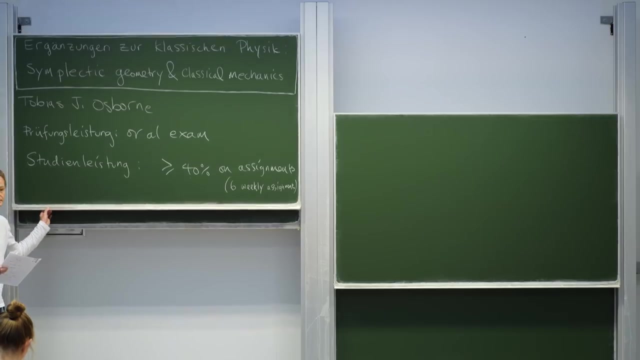 hardly need any of this language as the course goes, goes on. you also need to know a little bit about differential geometry, so hopefully you heard the word manifold. we're going to completely redefine everything in this course, but I'm just. it would help if you've seen this stuff before. 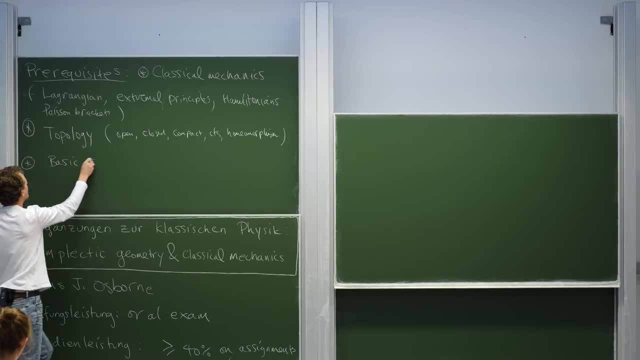 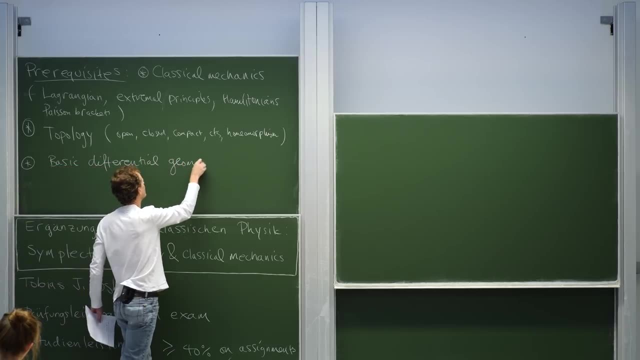 so it would help if you know, if you've heard the word manifold before. maybe tangent vectors, this kind of stuff you've probably met in various ways throughout your studies. but I'm just going to give you a little bit of a quick overview of what it is and then I'll get back to you when I have time. 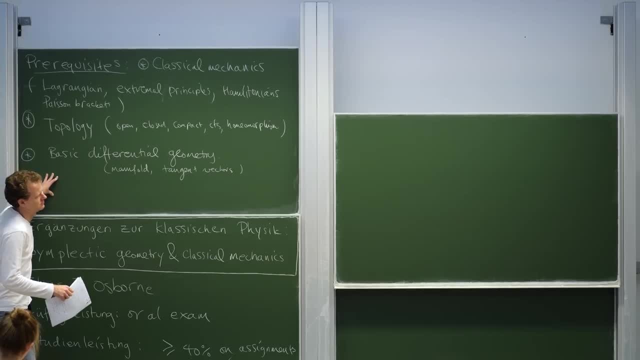 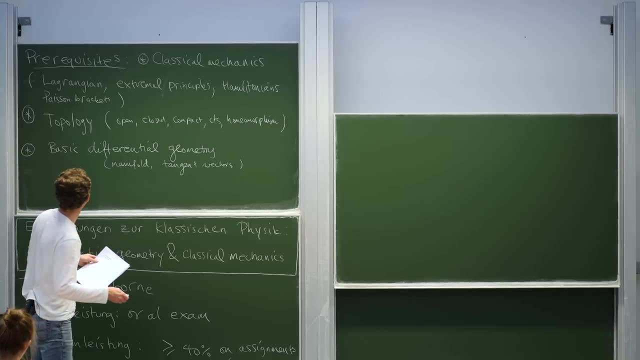 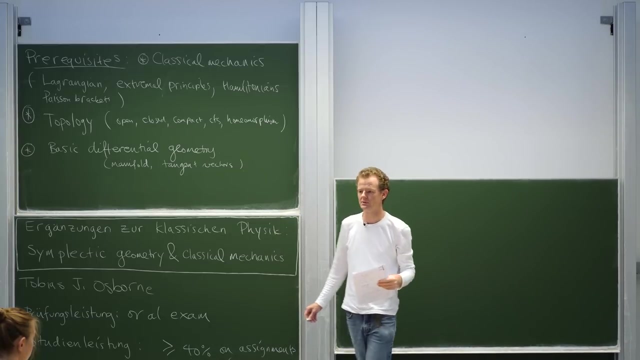 if not again, you'll get actually references to look these things up at your leisure. that's the prerequisites. we got some texts for this course. we do not follow one single textbook. there is no really one good textbook on this, so that's kind of annoying. but that's just life. we are have to put this course. 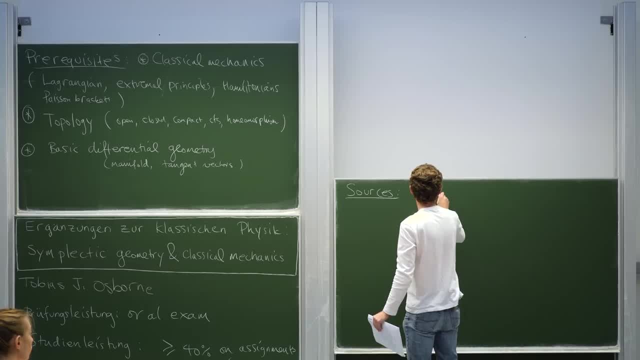 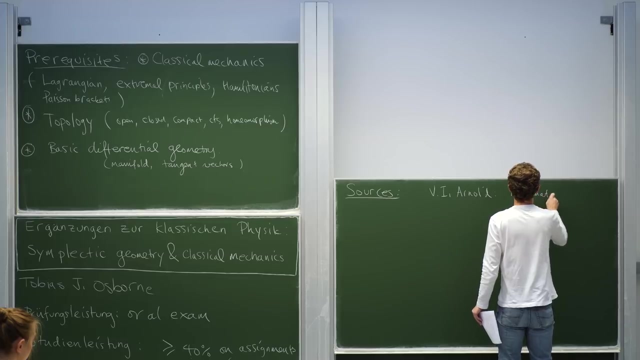 They're from various books. Now, ultimately, the best text to follow is that of Arnold on the mathematical methods of classical mechanics. This is really the canonical reference for this subject matter. It starts out super basic, this book. You learn about Lagrangians and Newtonian mechanics. 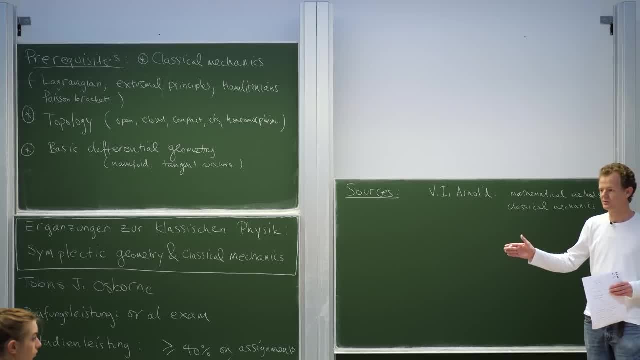 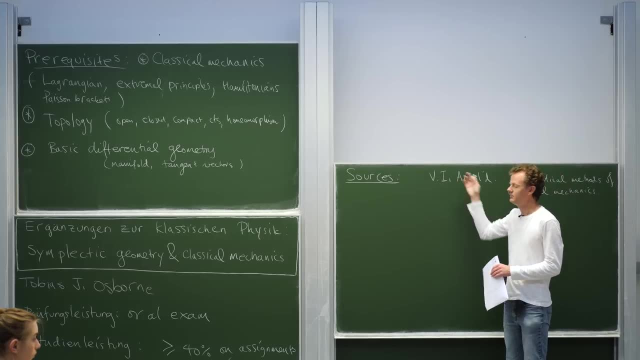 and so on at the beginning of the book. The subject material in this course will be sort of starting out about halfway through the book, so if you're a bit unclear on things. However, the really big shame about this is he uses a slightly different way. 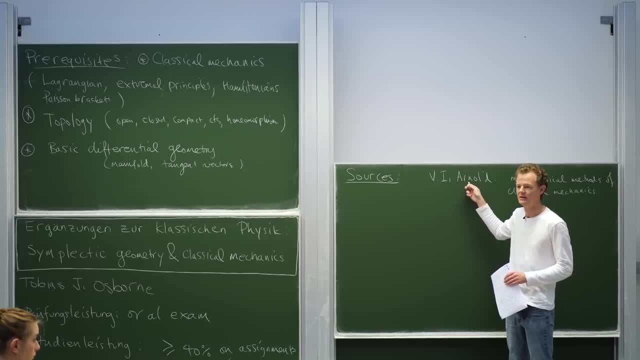 of defining manifolds and charts and so on. that will be incompatible with the rest of this course. So we're actually not going to follow this book directly because all the definitions are just. they don't follow the same standard forms that we'll see in all the other books. 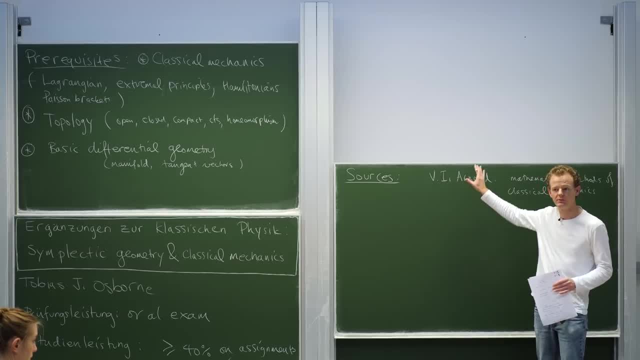 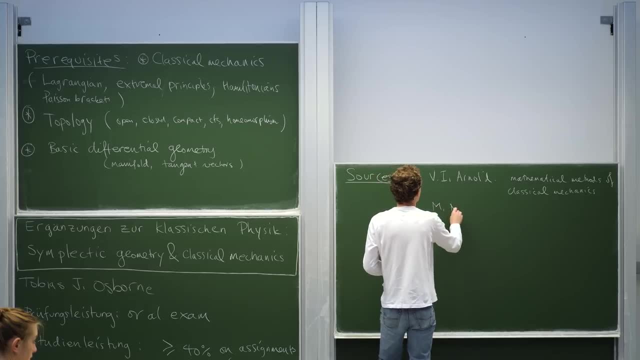 So I've decided not to follow this one directly, But this is the book that really underlies this course. Please do obtain it or take a look at it. For the first part of this course we've got to get through some definitions to get sort of into the subject material. 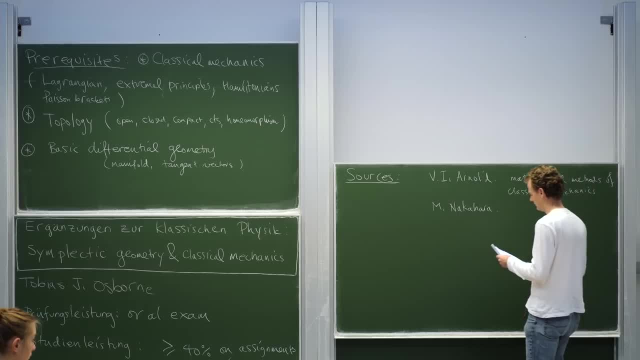 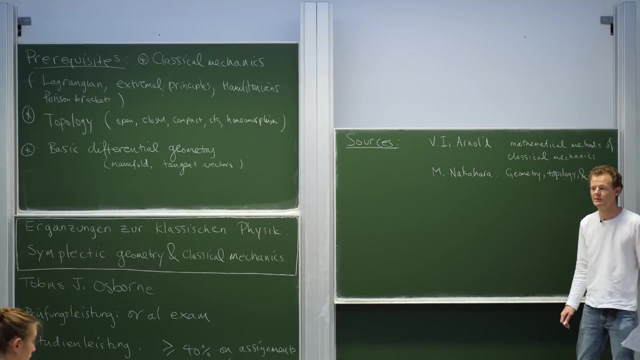 And for that we're going to follow the book of Nakahara. This is Geometry, Topology and Physics. It's a good book to have in your bookshelf if you want to stay anywhere in the subject area of physics or even, to some extent, neighboring areas. 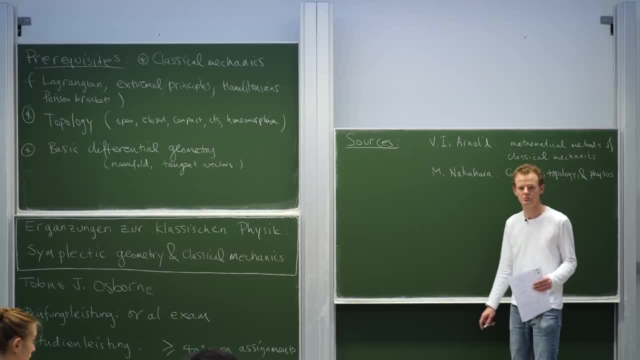 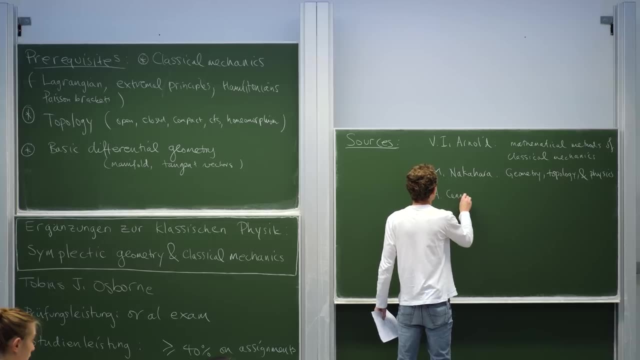 like Chemistry, Biology. This is a useful book to have And for the large part of the second half of this course we're going to use. very briefly, we're going to use a very lovely book of Kanasta Silva, or Kanada Silva. 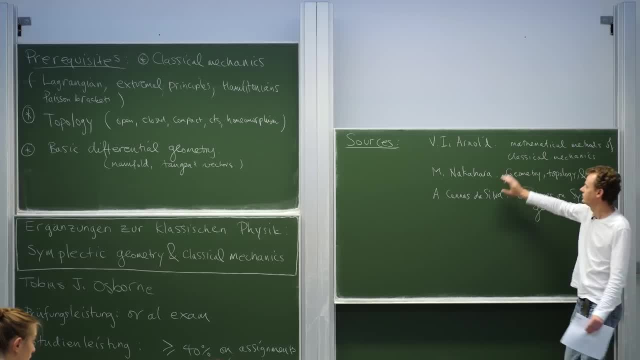 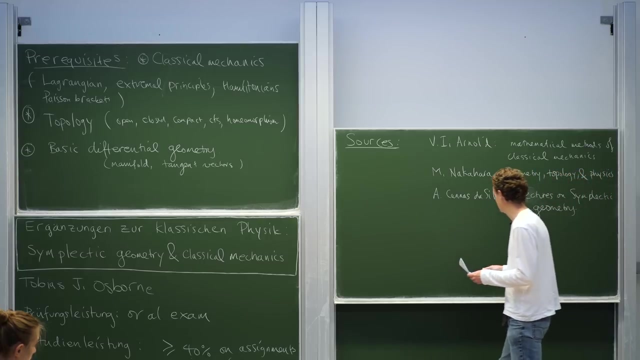 So, if you like, the course is somehow pieces of all these three books pasted together in, hopefully, a coherent fashion, So you would do well to obtain all three books and use them as background reading. There's other books that are somehow indirectly used in this course, which you can look up at your leisure as well. 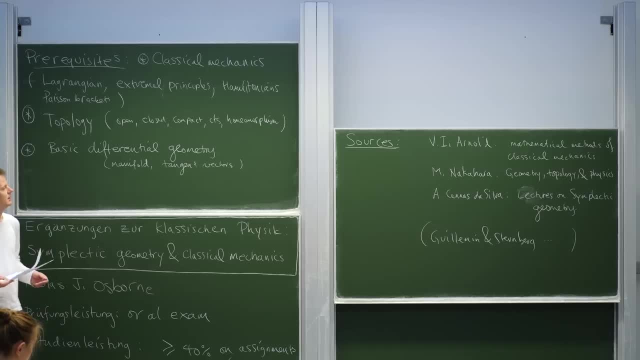 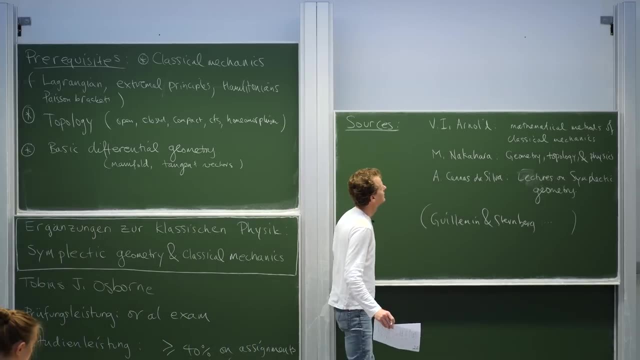 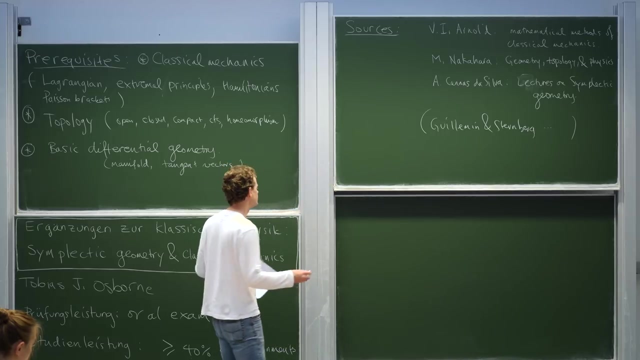 if you're interested to get a little bit more background, All right, That's the sources, the prerequisites, the assessment, all of that kind of stuff. All right, then let's look at the topics we're going to cover in this course. 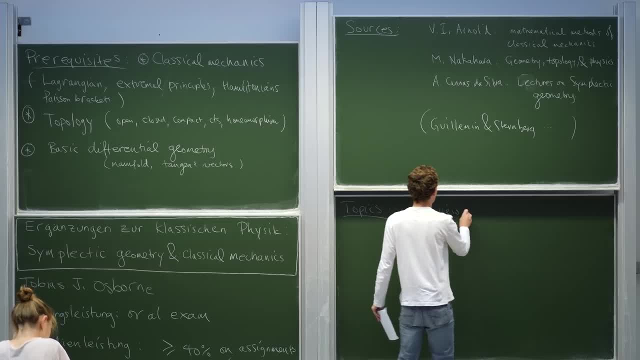 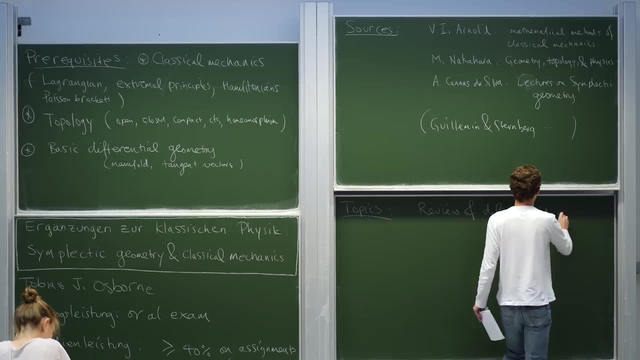 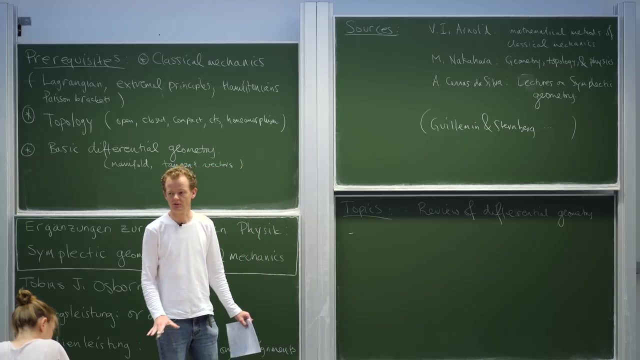 So the first topic that will occupy us for a couple of weeks is a reasonably comprehensive review of physics, A reasonably comprehensive review of differential geometry. We're just going to have to work through those definitions and do some examples and exercises in order to get comfortable with this language. 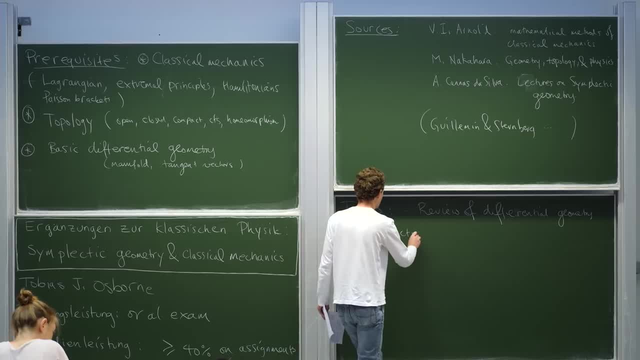 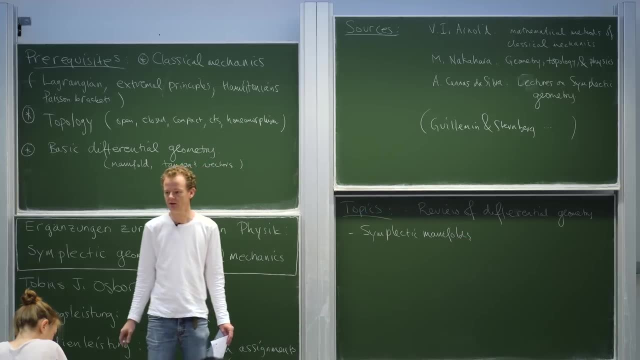 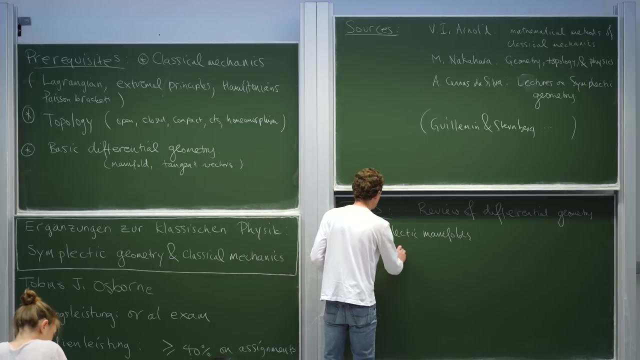 Then we'll get onto the objects that will interest us for the rest of the course, namely symplectic manifolds. We'll be able to talk about those after we've introduced differential geometry, And then, at that point I guess, we'll talk about the Darboux Theorem. 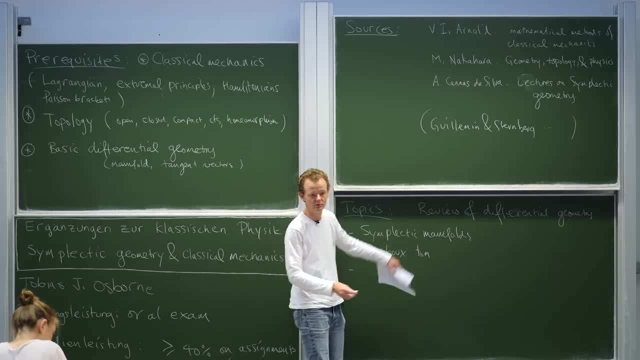 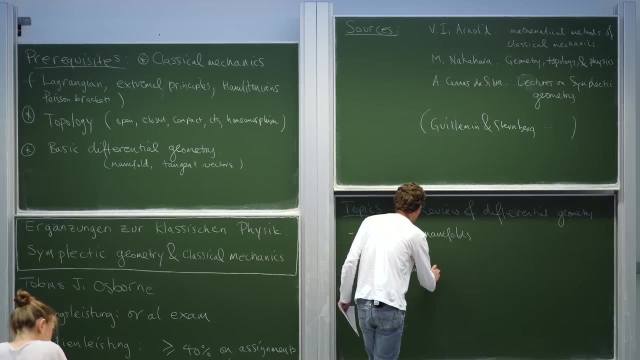 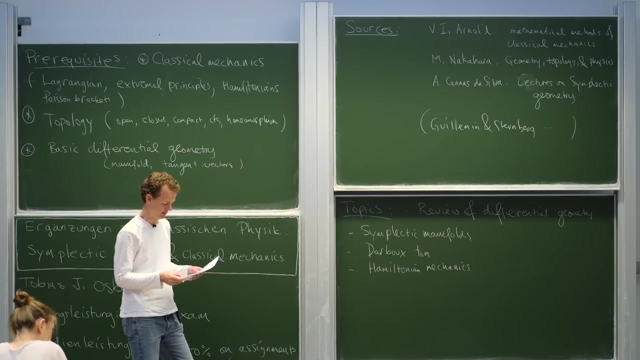 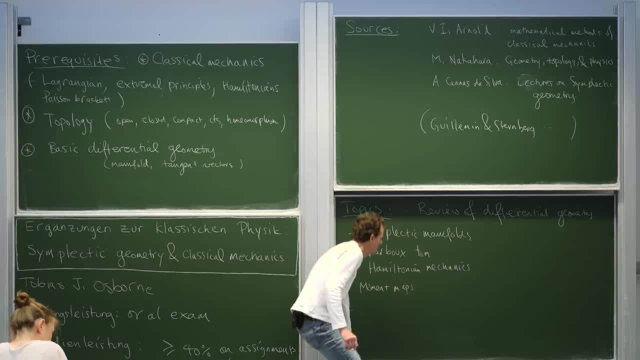 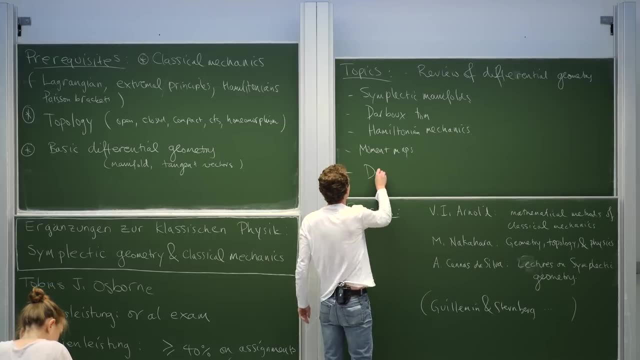 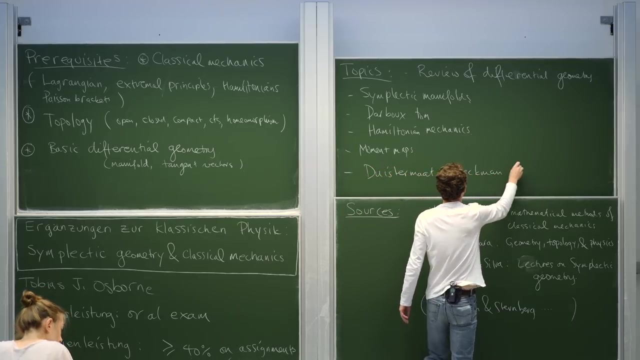 in this field, which is a theorem or a bunch of theorems, You know, I think you could say D'Eustermann and Heckmann. OK, that's the objective for the course: to see these things, to cover these topics throughout this course. 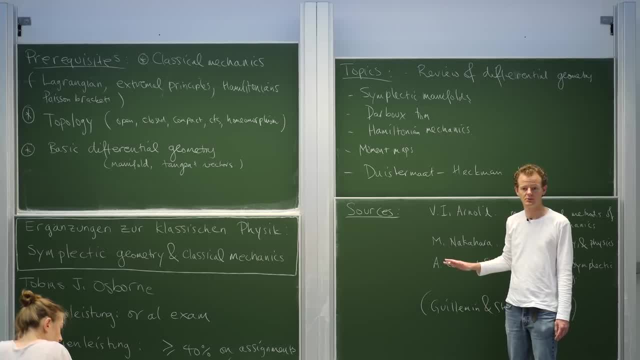 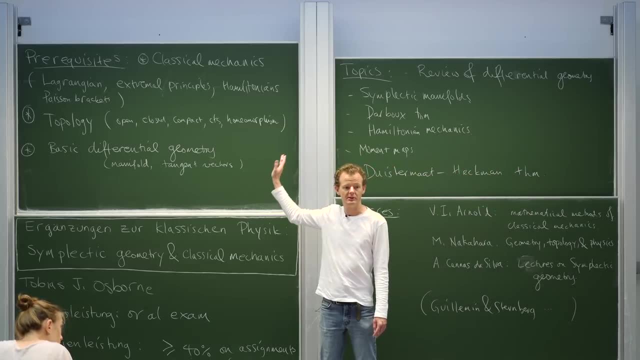 So this is a course in a physics department, not a mathematics course. So what does this mean? It means that we're going to talk. We're, Although this material is completely mathematically rigorous. there's no point in this course where I'm going to wave my hands and say: 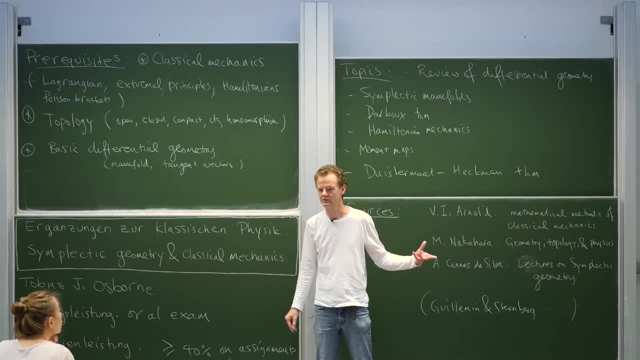 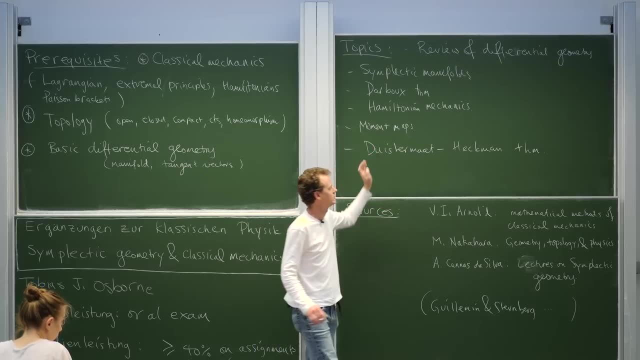 you need to know some physical intuition to get to the next step. Everything here in this course, all this material, can be proved at the level of mathematical rigor. Although all that is true, we're not going to prove things at the level of mathematical rigor. 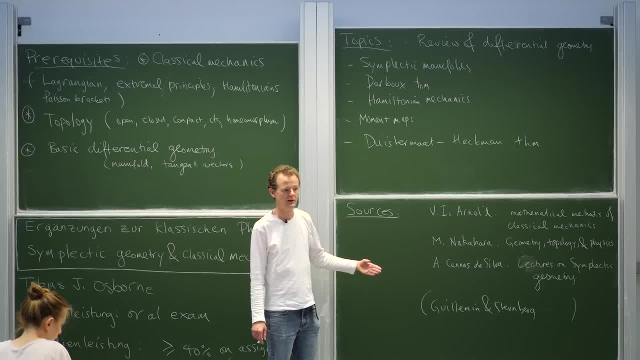 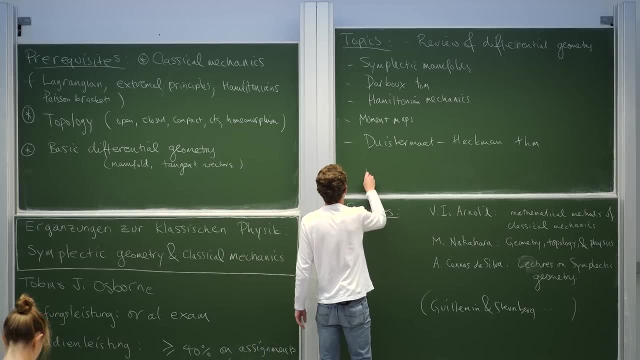 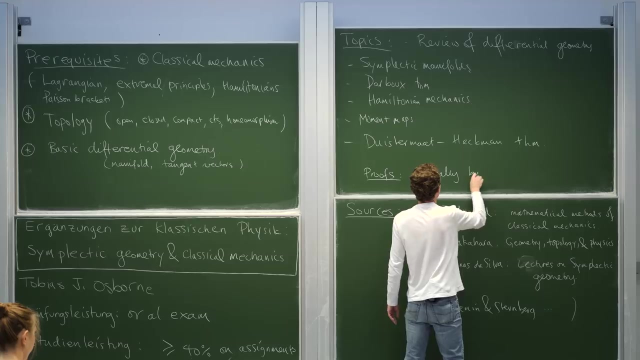 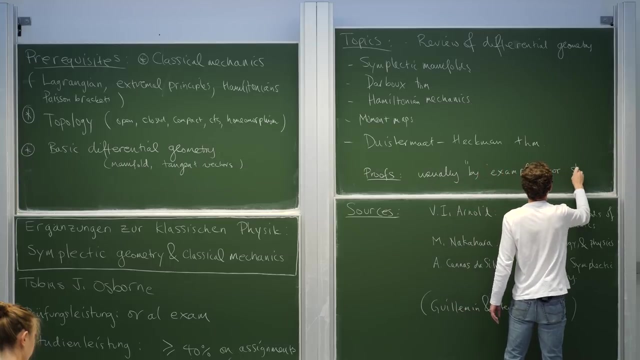 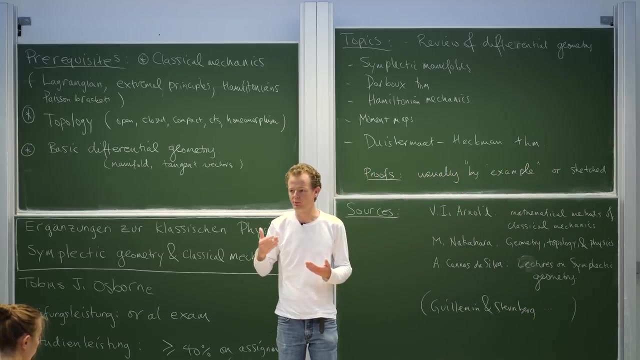 So that'll allow us to get through the material quicker. And I'll appeal to examples often in order to establish results. So the proofs in this course will usually be in the form of a proof by example. So we'll look at an example where we can check everything. 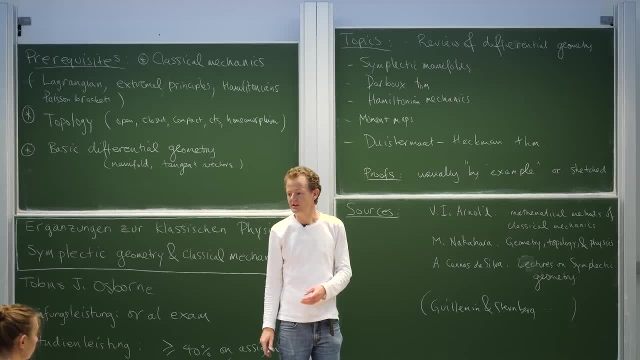 and see how the proof works, And then we just leave the kind of more abstract formulation of the proof either to your background reading- and I'll definitely be able to give you a reference for every proof- Or indeed we might just prove things using more physical sketch arguments. 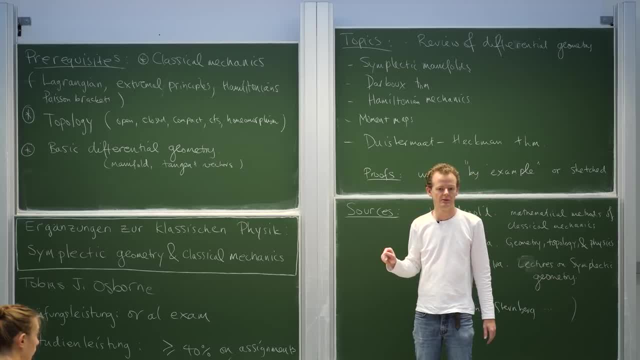 than going through all the little steps of a proof. So that's the kind of level of this course. This stuff is all rigorous, but we're not going to cover it at the level of a mathematics course. If that's what you want, then the Maths Institute does have courses. 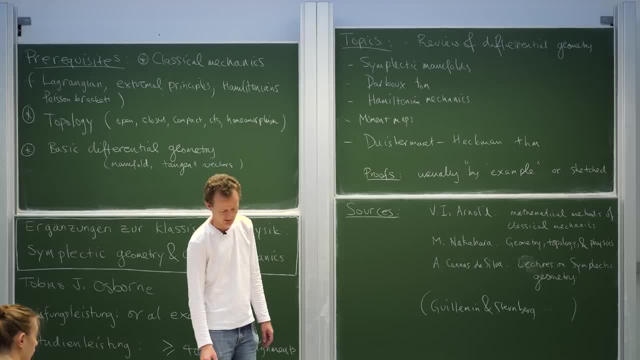 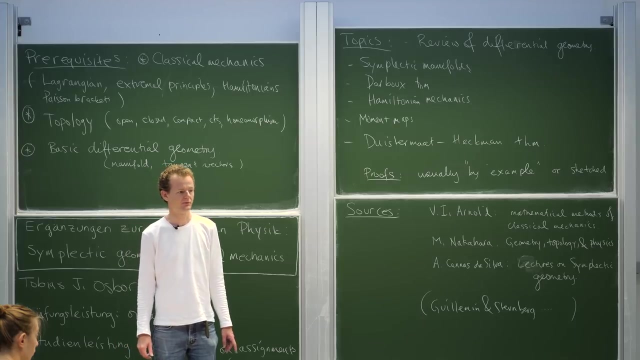 It's at your disposal to learn this stuff more rigorously, And the emphasis here will be on applications to physics, Right? So I think that covers all the sort of boundary conditions background material for this course. Are there any questions? before we proceed, 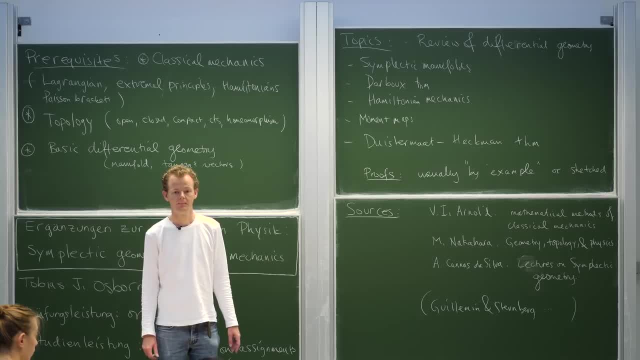 No, Oh yeah, There will be an exercise class. It will occur in the three and one, So we'll have two lectures in one week And then next week we'll have one lecture on Thursday and then the exercise class on Friday. 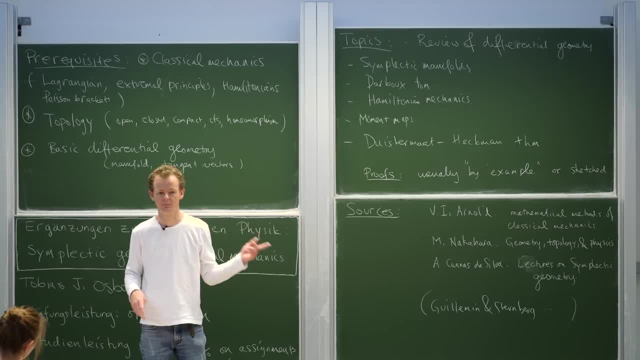 And then again. this periodicity continues: Two lectures, then one lecture and then an exercise class. It might be that we move the exercise class from Thursday to Friday, depending, But at the moment this is the current plan, Yeah. 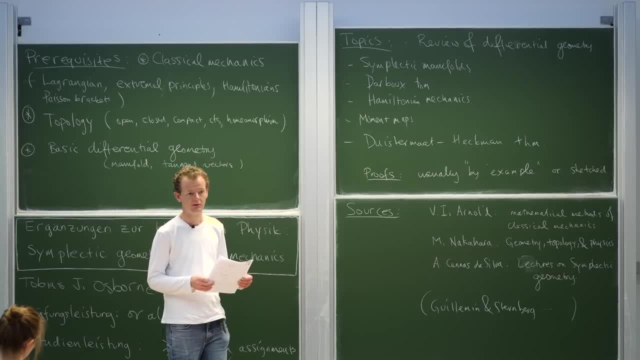 The lecture notes will not be distributed. They will be distributed for this course, That's more, also for people watching. The notes for this course are handwritten, And indeed, as I go along I often change what's written here, And so the canonical notes for this course. 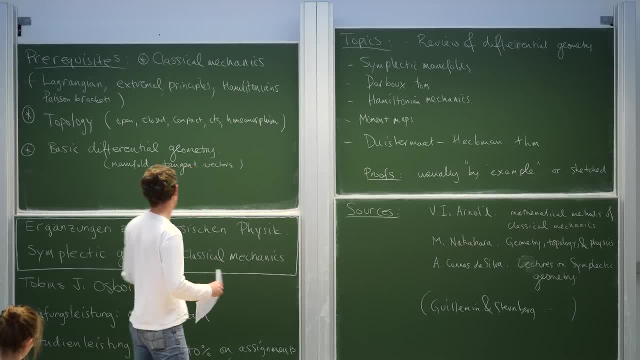 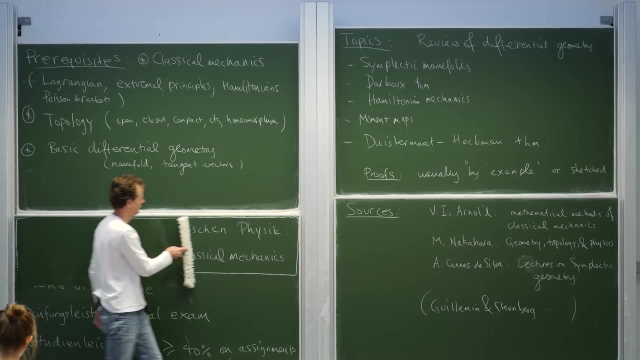 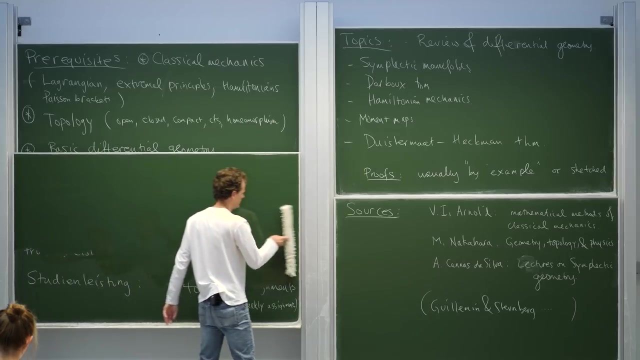 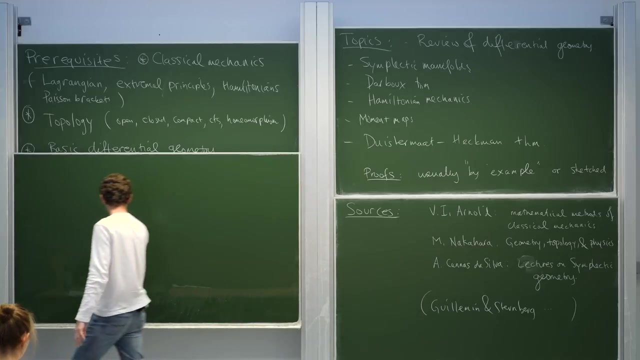 are what's written on the board, So you have to watch the videos or write them down if you want the lecture notes. Yeah, so it's more like a Yeah, Yeah, Yeah, It's good, It's really good, It's really good. 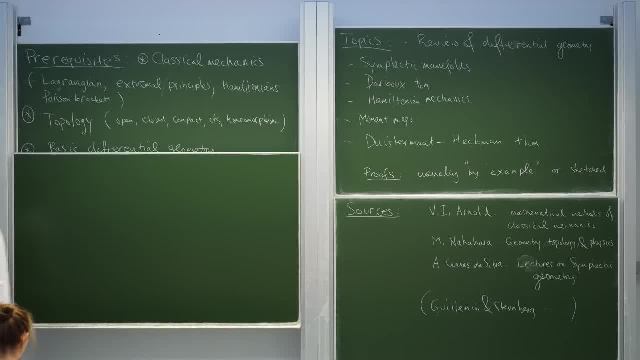 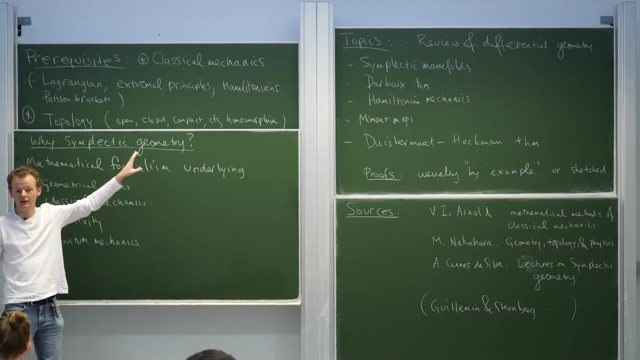 So why symplectic geometry? I mentioned this before. Why symplectic geometry? This is why we care about symplectic geometry, because it's the mathematical formalism underlying all these areas in physics. If you like, it's a unifying formalism. 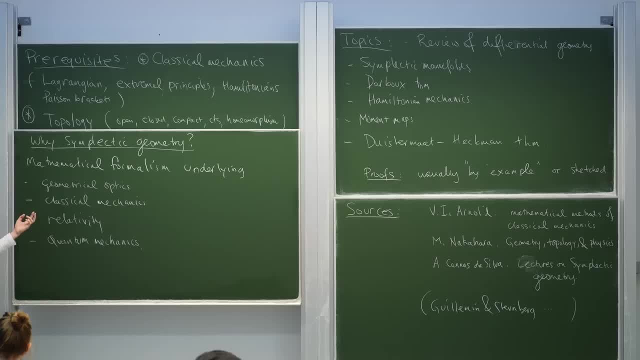 And we like unifying formalism. I mean you shouldn't become obsessed with unifying formalisms, But when you have a good one, then what it will do is it will allow you to take ideas and tricks in one area and apply them to get results in another area. 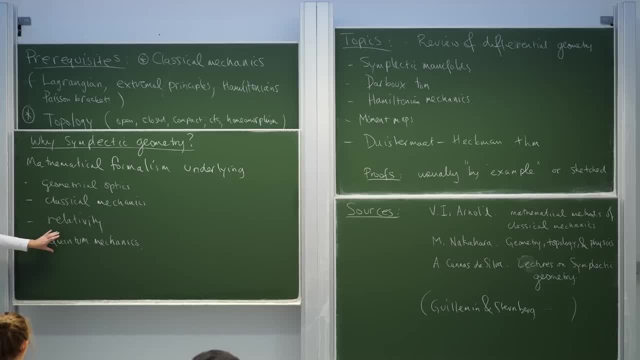 And so that's why we like formalisms, And when they're good, that's what they do. They give us ways to solve problems in one area by using tricks from another. It also simplifies things. When you have a good one, you have a good one. 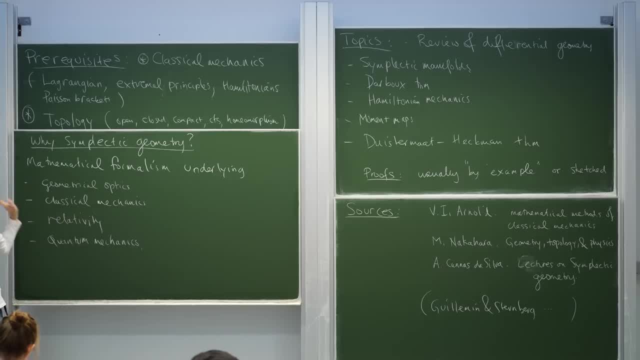 When you have a good one, you have a good one. When you have a good underlying formalism, not a bad one- There's no shortage of formalisms out there- But a good one allows you to compress what you need to learn. 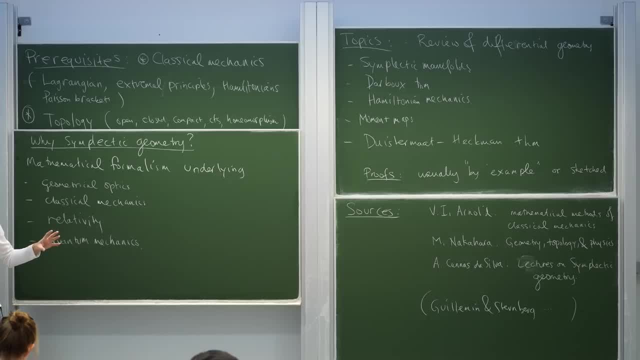 It allows you to reduce the surface area of the stuff you need to remember. So when you learn physics for the first time, it looks like just a vast array of heterogeneous array of different methods, different theories, different techniques and so on. And as you go through your physics training, 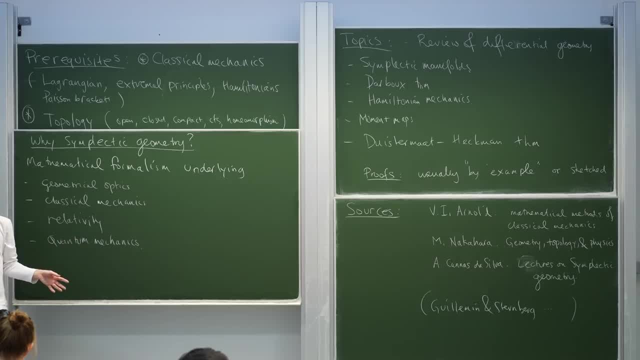 you learn that there are principles underlying this heterogeneous, this collection of ideas and methods and so on, And then, as you go even further along, you start to see sort of the bigger abstract picture of what's underlying everything, And so you could make a pretty good argument that 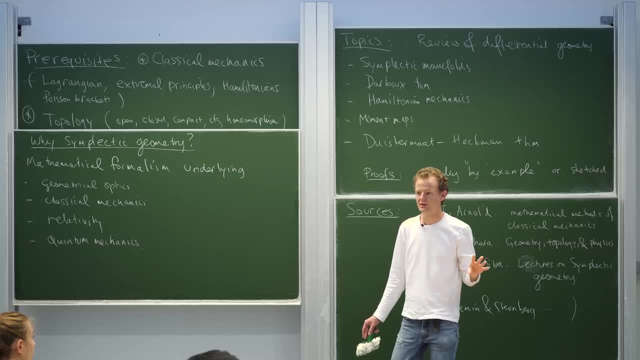 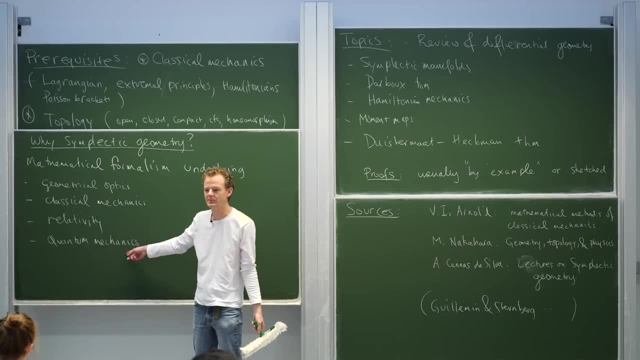 symplectic geometry is one of the bigger abstract structures underlying physics as a whole. Now, there's gaps in this list. right, There's nothing about statistical physics here, although we could put that there. There's a sense. There's a sense in which the symplectic geometry underlies statistical physics and thermodynamics. 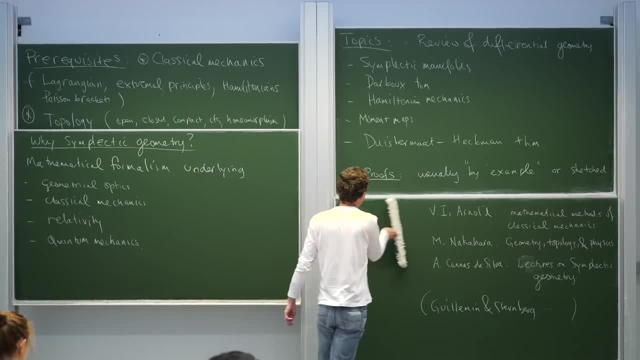 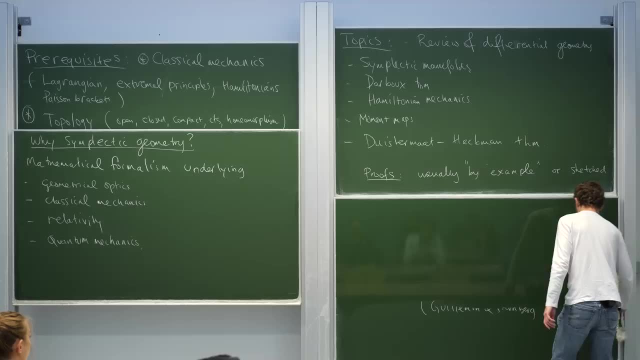 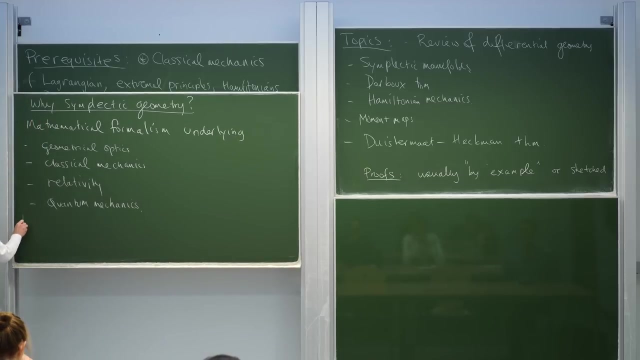 There's places where it doesn't work, at least not very easily. It's usually in systems with dissipation, friction, loss, noise. Well, it's not entirely true. So I should say, where it doesn't work so well, It's not so good for. 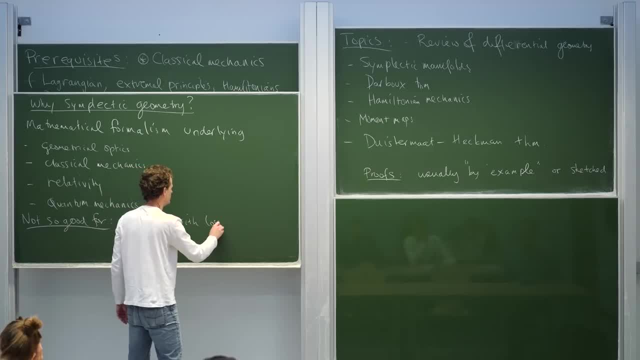 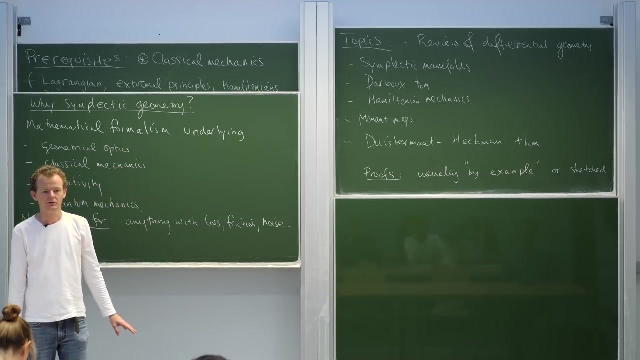 That doesn't mean to say that you can't apply it in these settings. Indeed, sort of recently I was delighted to learn that you can apply symplectic geometry to study systems with quantum noise. So that doesn't mean it doesn't somehow live there. 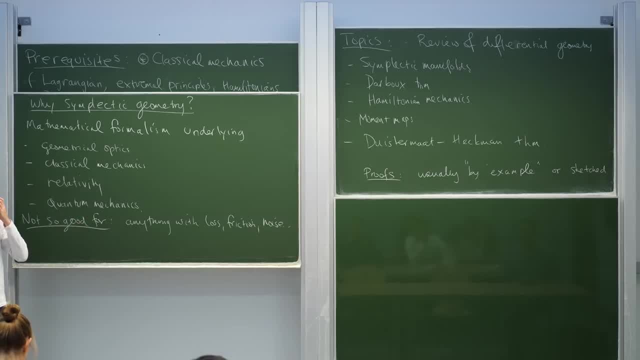 but it's just not as useful for these sort of systems. So if you're interested in physics of very noisy, very lossy systems with loads of friction, then probably symplectic geometry isn't the formalism you'll run to to solve your problem. 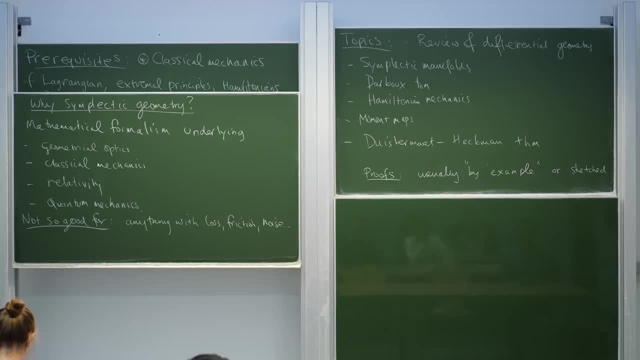 You'll go for a different way of setting up your problems. But if you're interested in in closed systems, then if you take a little bit of extra effort to phrase everything in the language of symplectic geometry, then you might find that if you came up with a result, 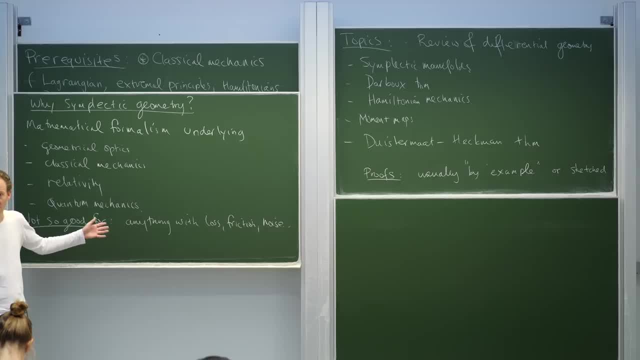 that you could actually generalize it to many, many other places and learn many more things. So we like formalisms because they reduce the surface area of things we have to remember, because once you know the formalism, then every other one of these topics 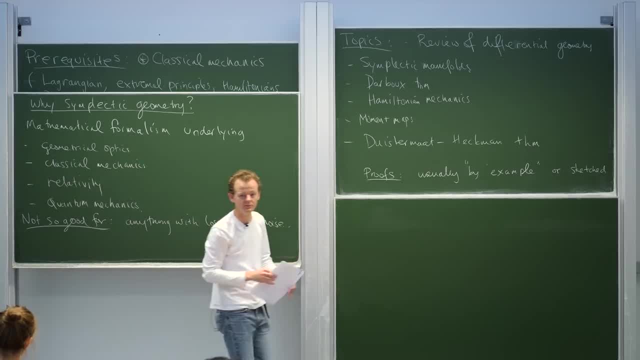 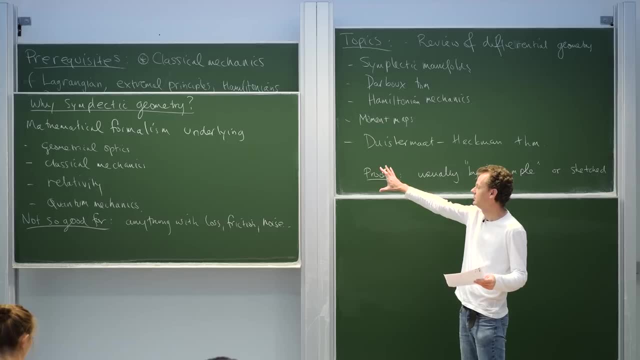 just because just becomes an example or an application of that formalism. They help us to learn things, but it's not always. it's not the like. this is not the silver bullet or the panacea for all problems. All right, the objective for today. 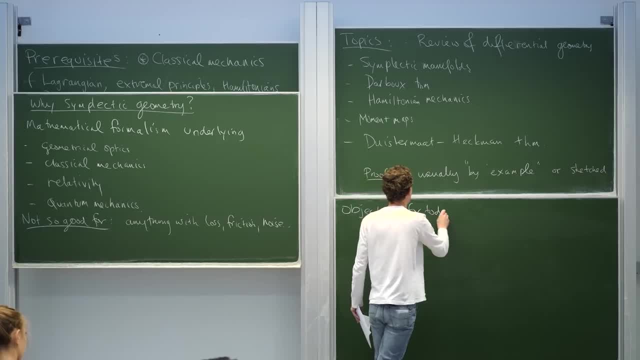 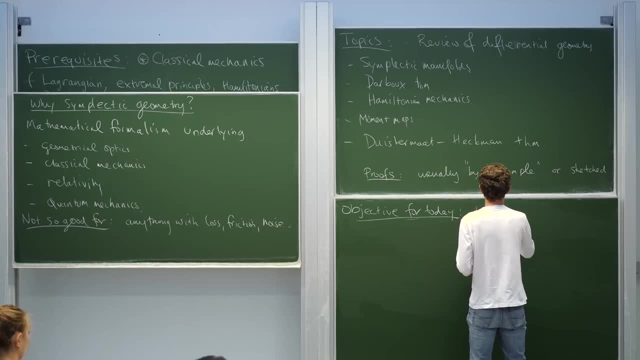 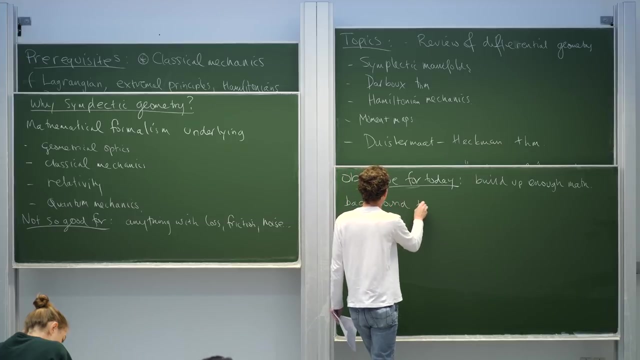 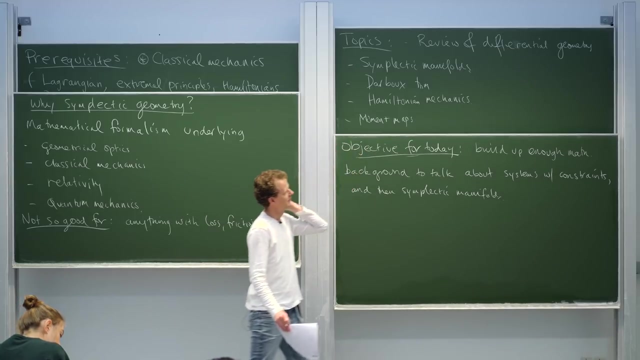 well, the next couple of lectures is to build up enough mathematical background to talk about these things. All right, so brace, brace. The next couple of hours of this course we're going to be writing down definitions. 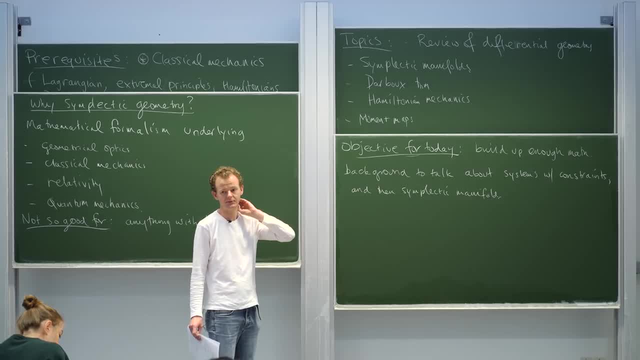 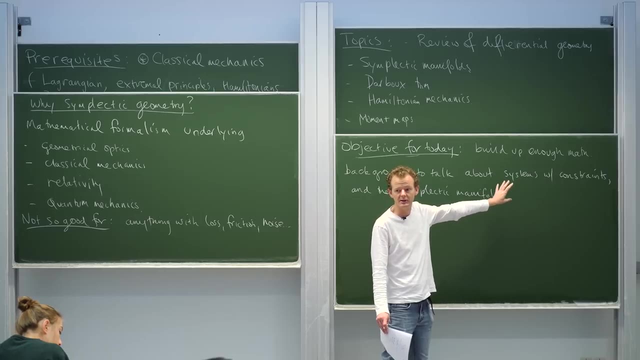 And the reason we're going to do that is to give us enough background to actually start talking about interesting mechanical systems, ones that model these settings here. And then we're going to use this more general mathematical background to introduce the things that really underlie everything, which is symplectic manifolds. 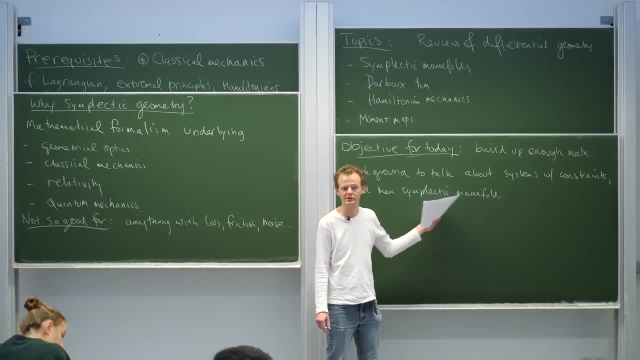 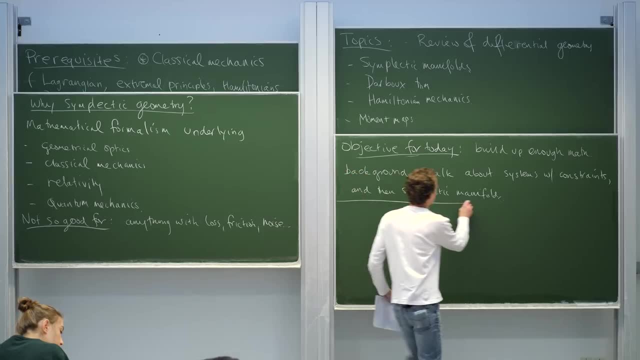 So I estimate sort of by lecture five or six we'll be onto symplectic manifolds And for the next three, four lectures we're going to be talking about simplectic manifolds. Our first definition is by far the worst definition in the entire course. 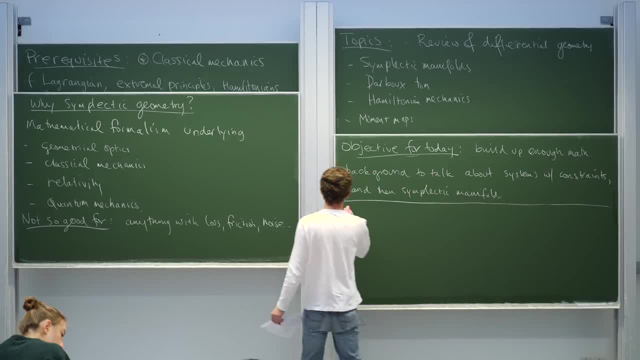 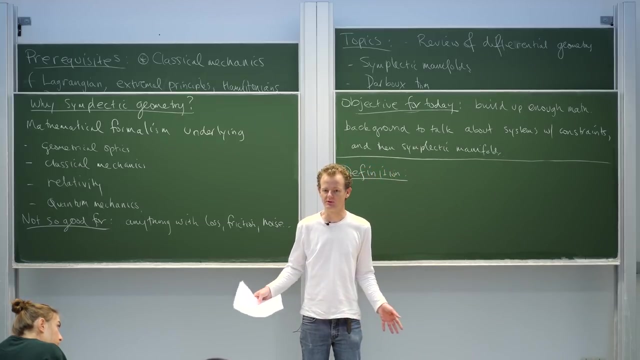 If you can hold on for this, then you'll probably be good. We need some mathematical way of talking about the things we want to talk about. This is the most general way to do it, And we're going to get more and more specific until we really just focus on examples. 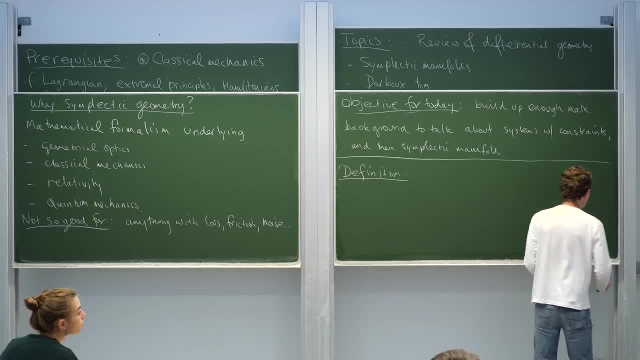 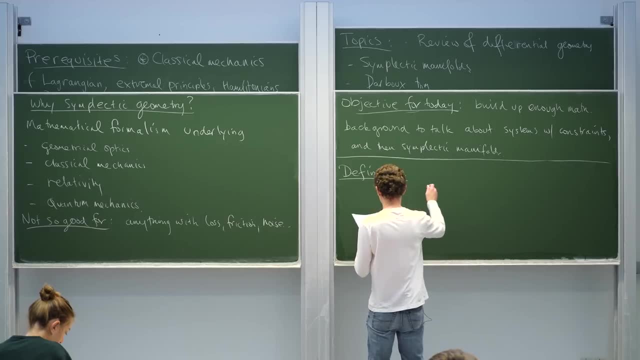 So this is, like you know, looking at Euclidean space and then generalizing that beyond the point of recognition It's not so bad, All right, All right, So the most general things that lie in the background, mathematically, for this entire. 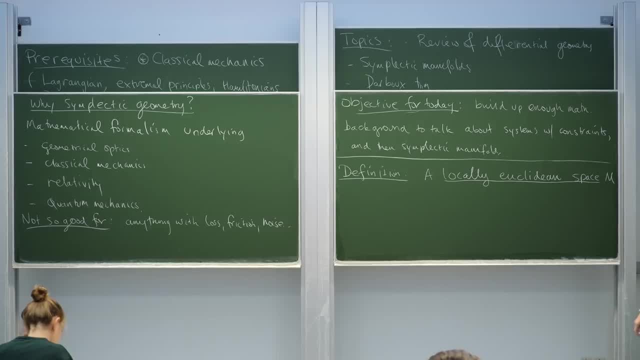 course are things called locally Euclidean spaces. So even before I write the definition down, let me just tell you in words what this is meant to capture. So we understand Euclidean space, n-dimensional Euclidean space. It's a very beautiful place to be. 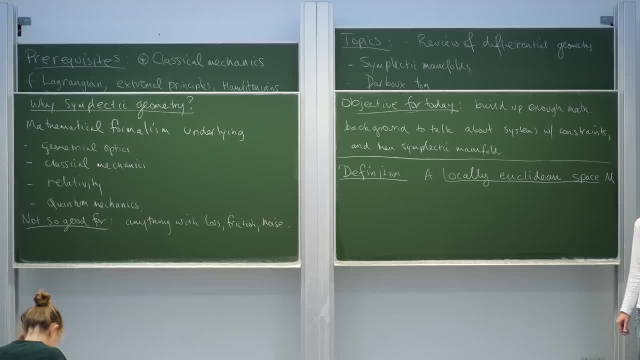 You can do calculus there, You can translate objects there without any kind of weird curvature effects. It's just a nice place to be, But it has lots of extra properties that we use, maybe unconsciously or consciously, And we want to generalize that to the kinds of spaces that we encounter in physics particularly. 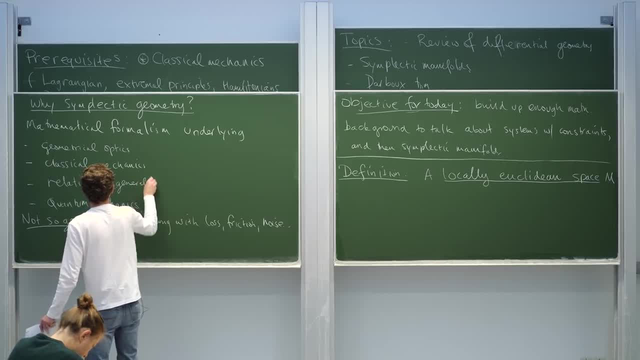 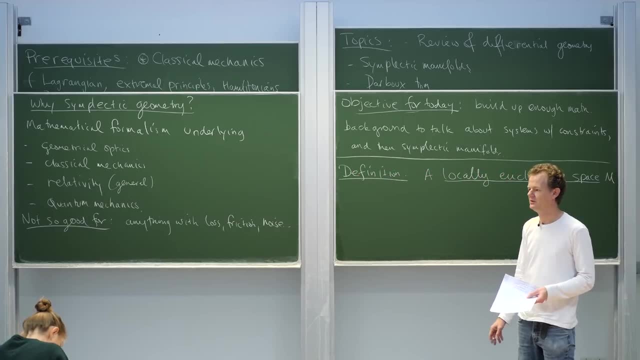 in relativity, general relativity. There we know that space isn't Euclidean. You know there's curvature and indeed it's not even Euclidean: It's Minkowski or Lorentzian. And you want to generalize those spaces. 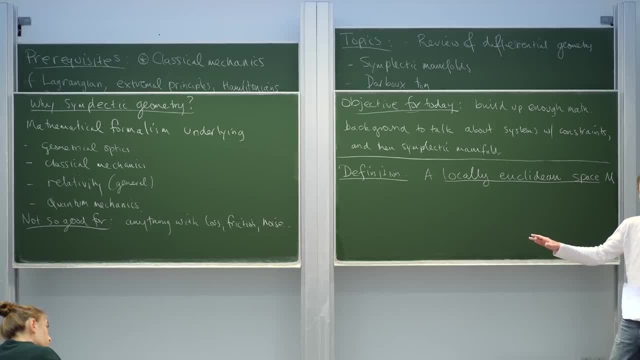 those things that work really well in affine Euclidean space that you know and love so well, to this more general setting. but you don't want to lose too much along the way. So the thing that you try and do is you try and say, okay, I'm going to give up. 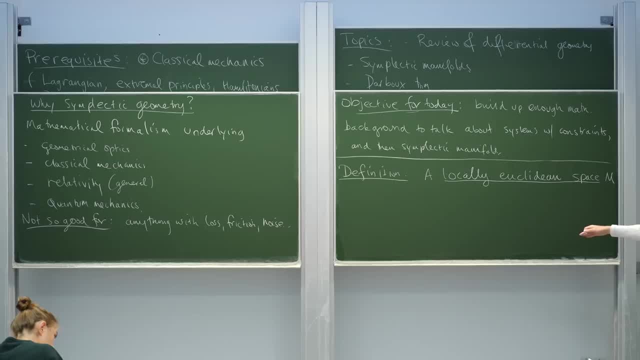 on spaces that are globally Euclidean, globally flat everywhere, with a coordinate system that's nice and rectangular. I'm going to give up on that and instead consider things that are the next best thing, right, Things that look like Euclidean space locally, If you're a little ant. 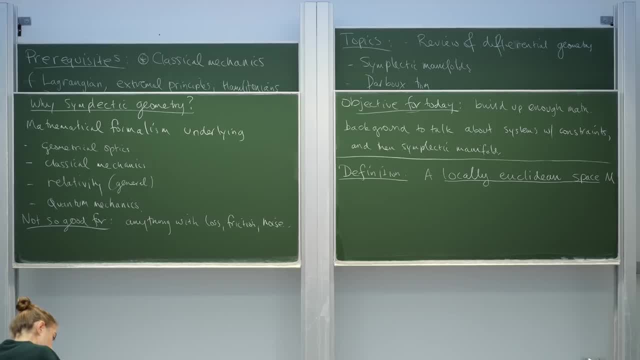 living in this space and you look around, it looks like Euclidean space, but globally things can be different. So that's the most general objects we're going to consider in this course. So in words, a locally Euclidean space is something that locally looks like normal flat. 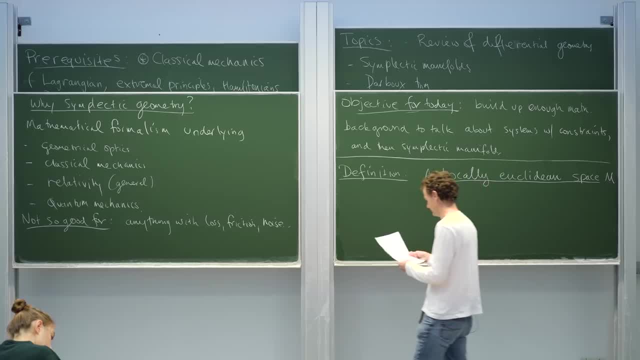 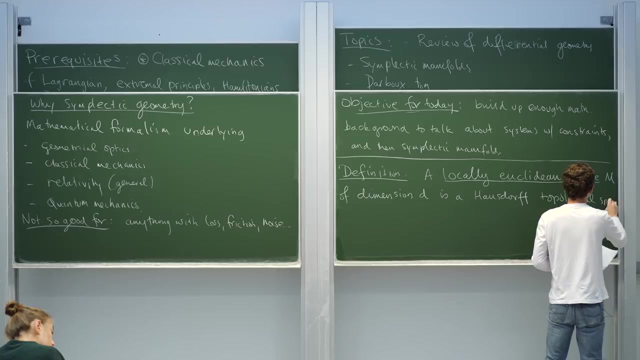 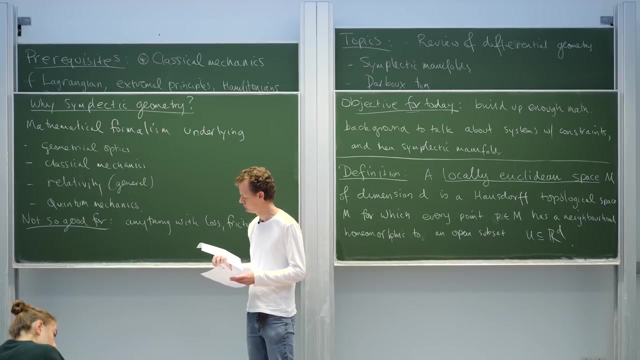 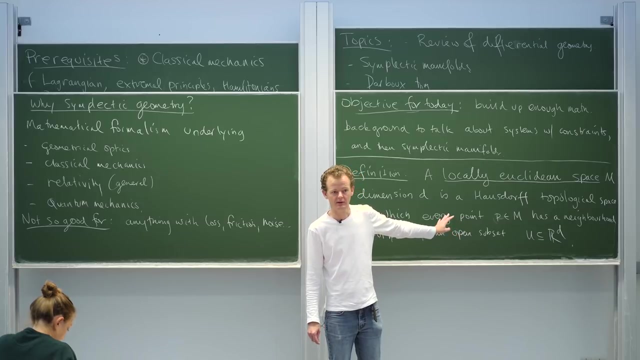 space, but globally not. Thank you, Thank you. Okay, that's the definition here. Locally, Euclidean space of dimension D is a Halstorff topological space. Those words you may or may not have encountered. Now, if you haven't encountered them and you don't want to encounter them, then just think. 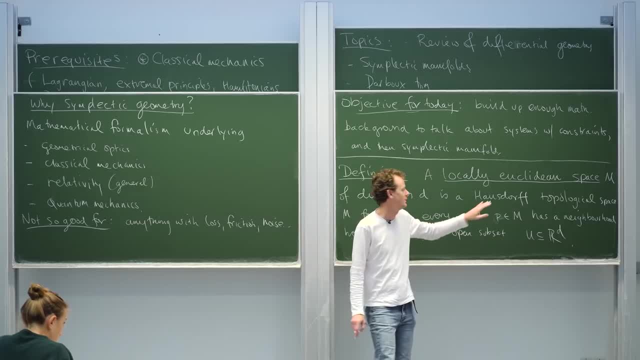 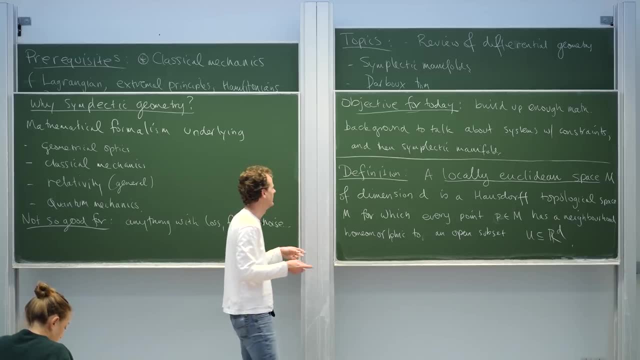 sufficiently. nice is the physicist's way of translating Halstorff: topological space. It means to every two points you can put little circles around them if you like that separate them, For which every point in this space has a neighborhood. that's also a technical. 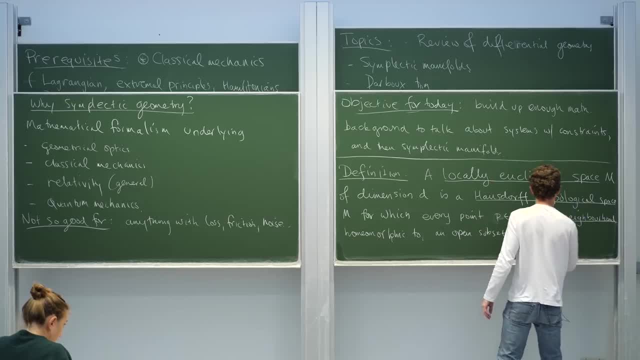 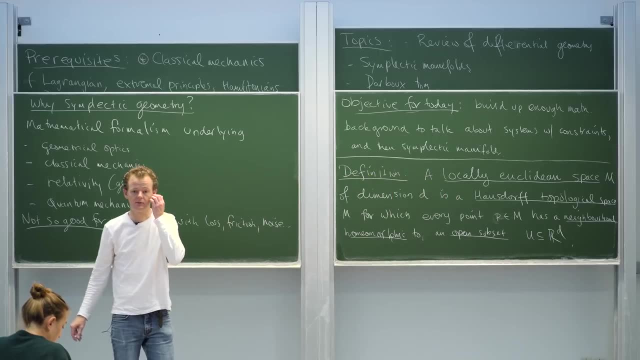 term- I'm going to underline the technical terms: Neighborhood, homeomorphic to an open subset of RD. So that's the way of capturing this physical notion that every point looks kind of like Euclidean space And kind of like here is captured by the word homeomorphic. 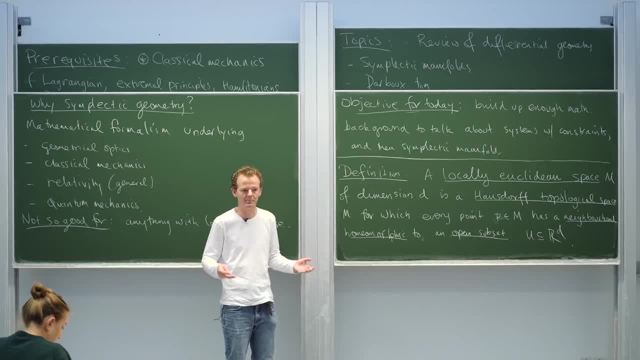 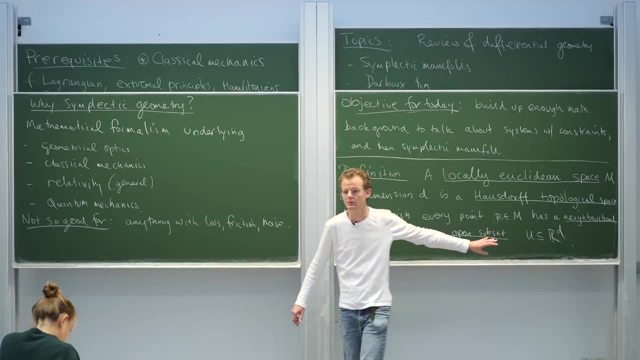 which just means continuously. There's some continuous map from some region around the point to some bit of Euclidean space. Okay, So if you can sort of hold on for that definition, then it gets sort of successively better, I hope, in this course. 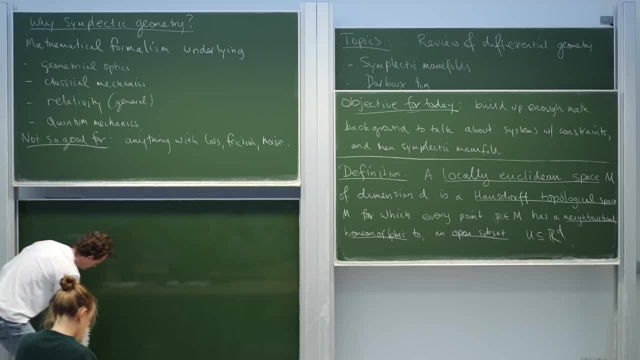 Thank you. Yeah, I guess I'll draw the picture already. This is a locally Euclidean space. What does that mean? It means that every point in this space is a little neighbourhood, where this neighbourhood can be continuously deformed into some nice subset. 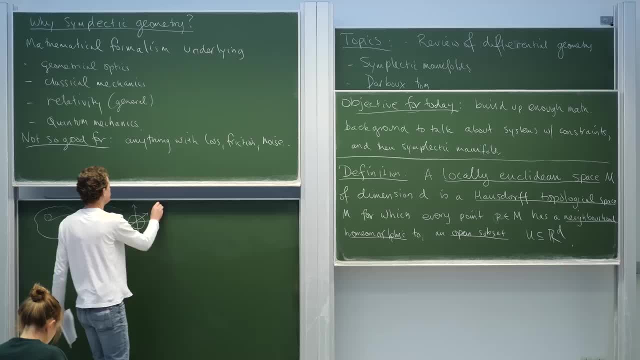 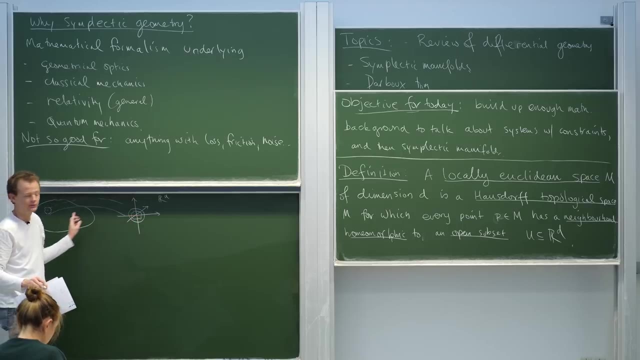 of r to the d. So every point in this neighbourhood has an image here in r to the d, and it's also a continuous map. So the map that connects our locally Euclidean space m, this most general object, to r to the d. 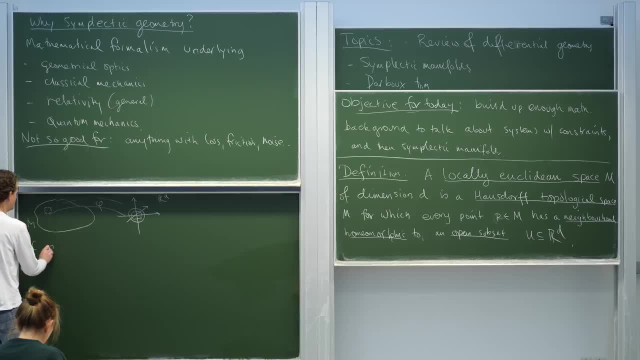 we're going to give that the name phi for the moment, And if phi? Sorry, I'm just going to change the notation slightly. I don't want to name the open subset we end up on. We'll just save pasta. We're going to get some empty pain. 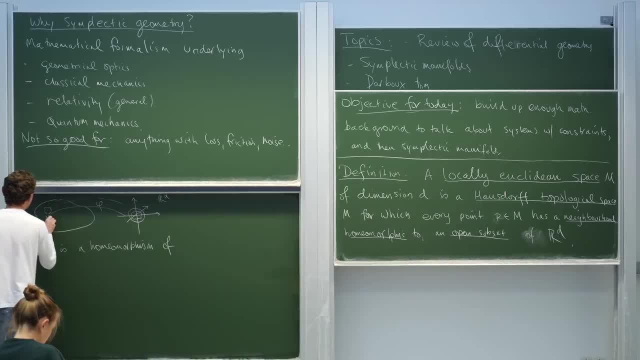 And we'll just say homeomorphic to an open subset of r to the d. I want to name the neighbourhood here, So that's the? u. You can do that on the host pair. So that's what you're gonna do, And for those it's going to be quite a lot faster. 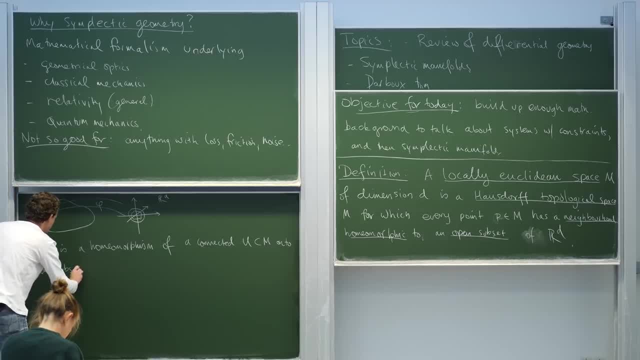 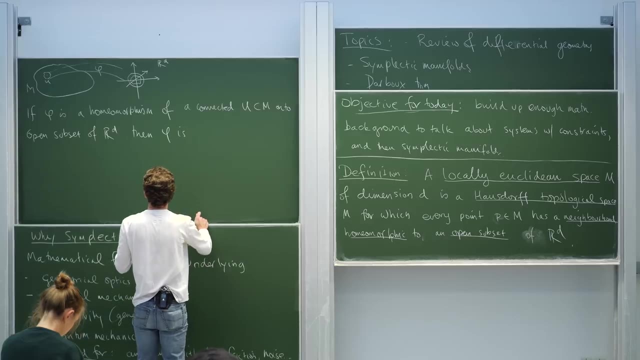 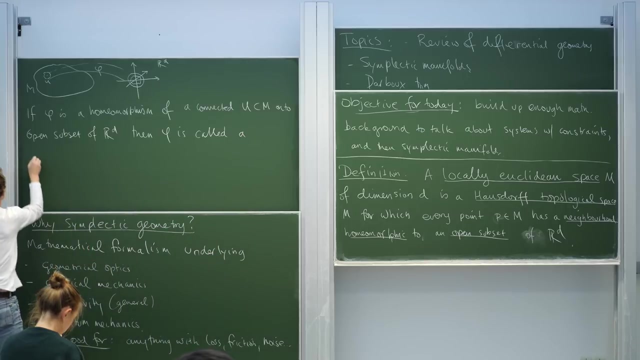 So, consequently, we want to have more els than us. You'll just have 90% percent of r to the d and we're just gonna shampoo the rest of it. So if we have this map that takes this region around, this point p to r to the d, then that map is going. 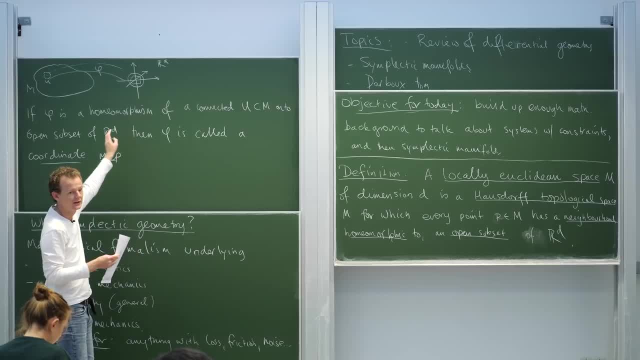 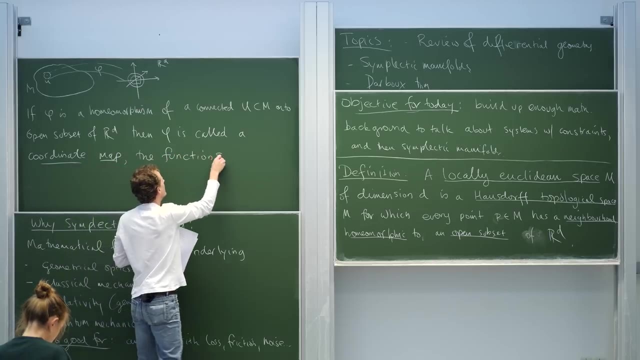 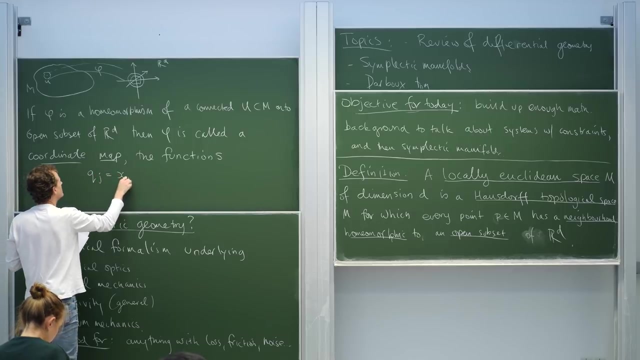 to be a thing called a homeomorphism. It's a continuous map with a continuous inverse And it's called a coordinate map. That's how we call these things. And this map is pretty cool because it gives us some functions on our locally Euclidean space. 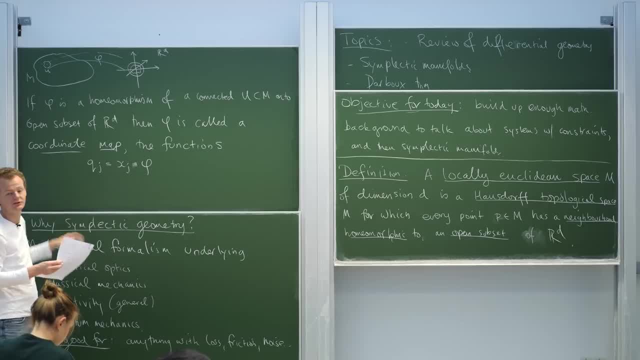 And those functions are what we would call the coordinates. How does it work? Well, you first go from your locally Euclidean space to r to the d And then you've got some real, really well-defined functions on r to the d, namely the coordinate functions. 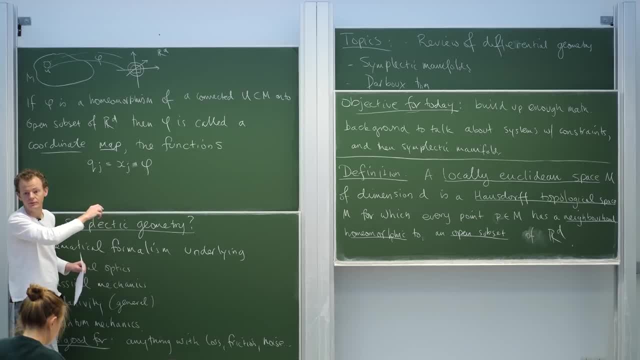 They tell me the j-th coordinate of this point. That's what that means. And so this map goes from m to r, And this map goes from r to the d, And this map goes from r to the d, And this map goes from r to the d to r. 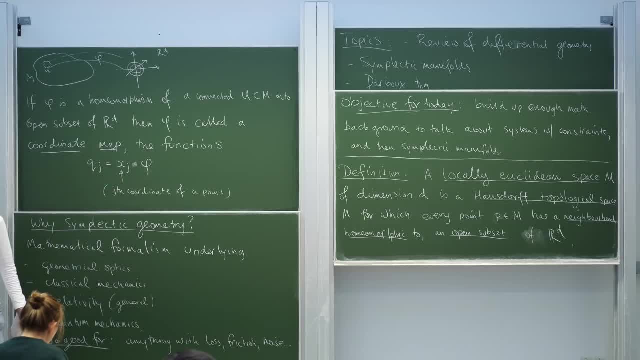 So we've got a map q which goes from m to r. It's easy to get lost in differential geometry. Maps are going this way and that way, and inside and outside, And so it's always worth just thinking through where does it go and where does it come from? 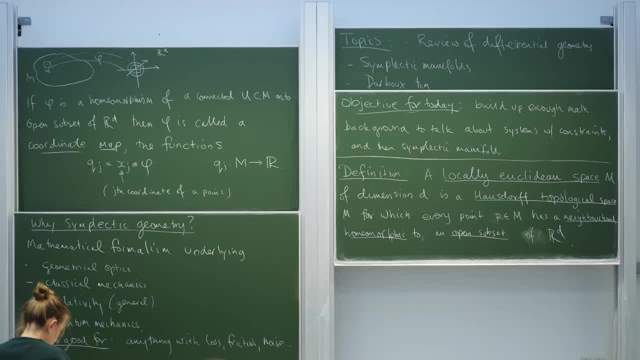 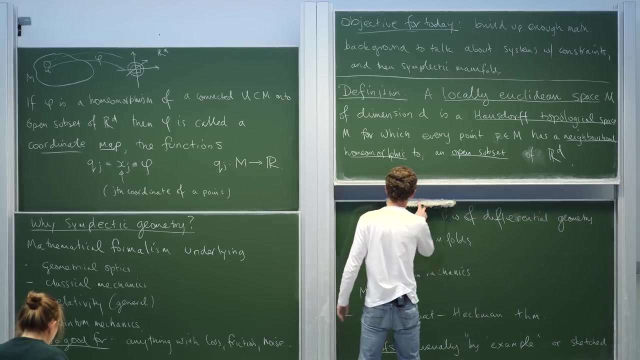 Where is it going to? So why don't we just go back to the original geometry? We've got the original geometry of the model And we're going to say hey到了. we're going to say hey, hh, hh, hh. 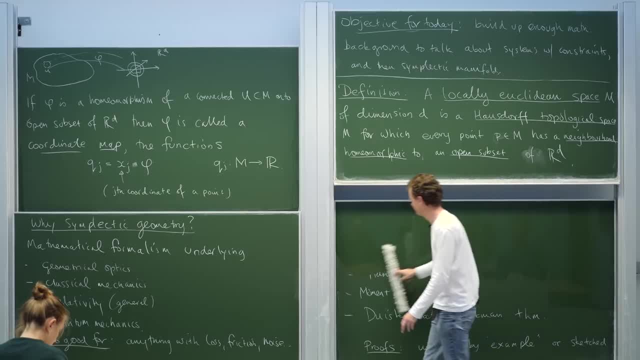 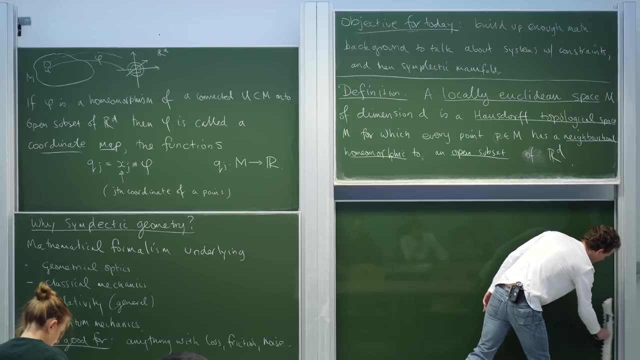 What's happening? It's not us, It's an angle. It's not us, It's me, It's the angle. Now we're going to move this calendula around, So this is the ellipse, And we're going to say, ah, our angle. 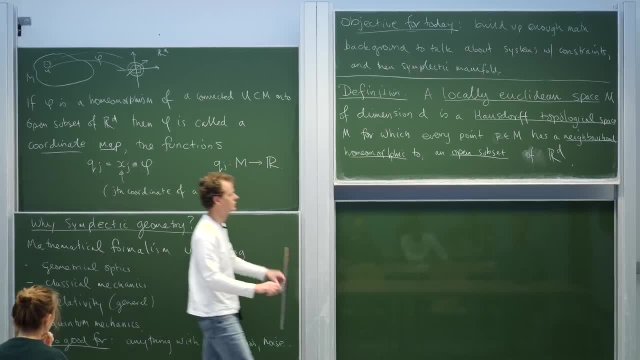 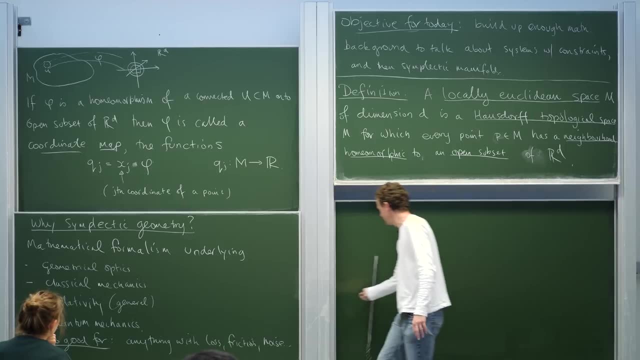 And then we're going to say: you know what? So, given these Q's, you can draw a grid or a coordinate system on M. You just define them to be the surfaces of constant Q, just like you would use the coordinates in Euclidean space to draw a grid on flat space. 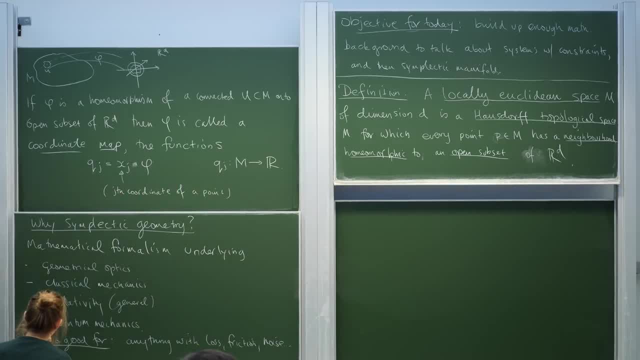 The grid is defined by surfaces of constant X, Y and Z and so on. So that allows us to build up a coordinate system on our locally Euclidean space. So I'll draw the picture again. Here's the locally Euclidean space. 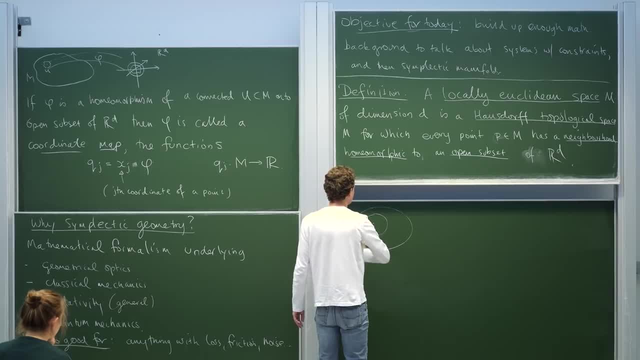 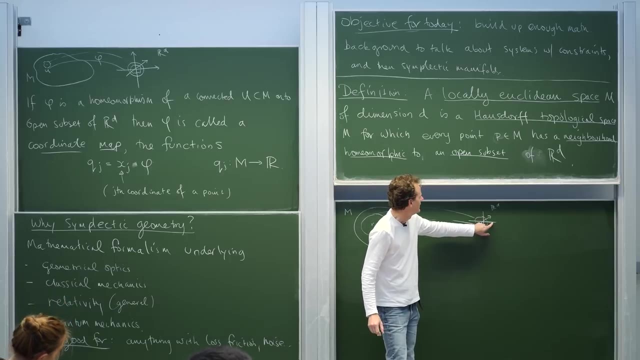 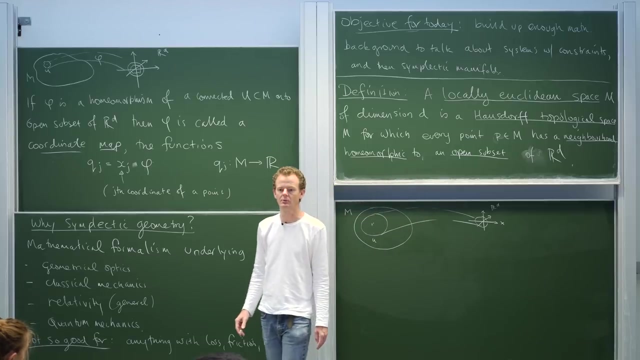 M. here's a point P, Here's some region U around it. Here's R to the D over here. Here's the map phi. And now this line here, which is the line of the X-axis, say the line of 0Y and 0Z. that has a pre-image right up here. 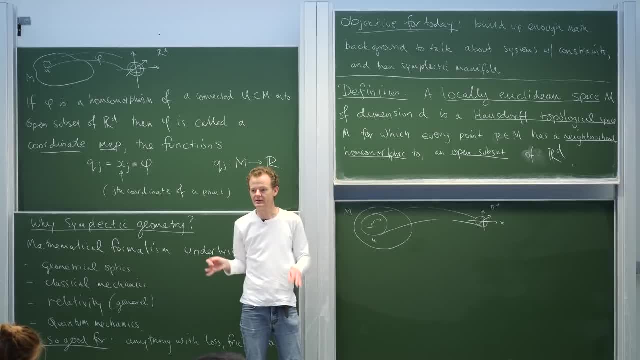 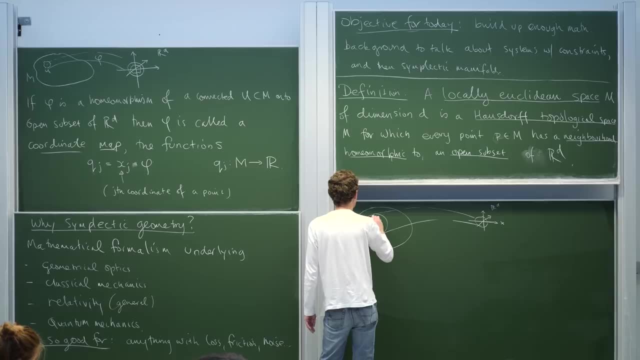 So maybe it looks like that It gets a bit distorted by this map, And then the other axis here gets also distorted, And so you can find something that looks very much like a coordinate system here, but it's a curvy coordinate system. 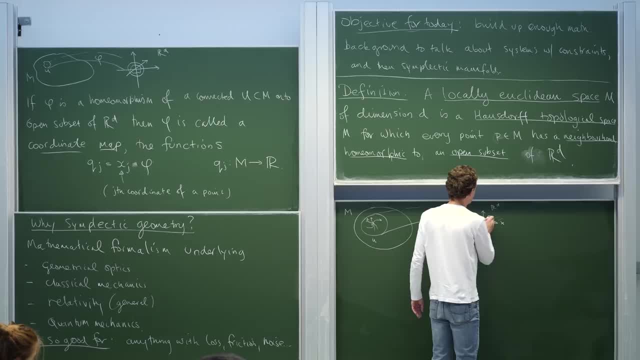 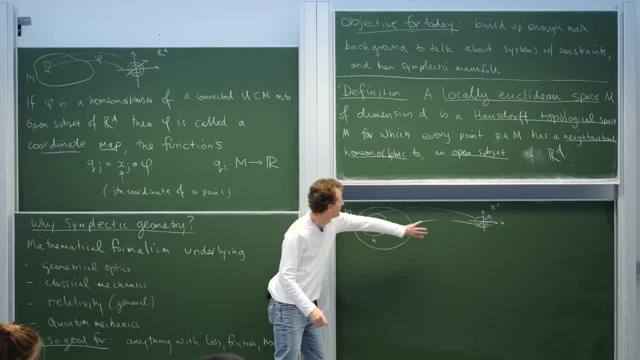 And furthermore you know you can. if you had a nice grid subdividing Rd into a lattice, then that lattice would have some curvy pre-image here in this locally Euclidean space. So that's like almost as good as Euclidean space. 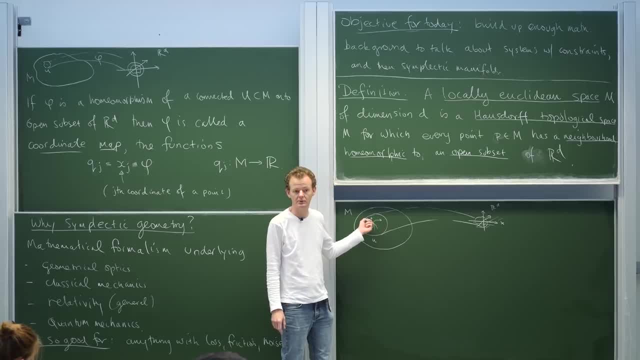 Every point here has like a coordinate which is a list of numbers. It's a list of D numbers, in particular these every point in M sufficiently close to P. So that's a good idea, But of course there's a problem. 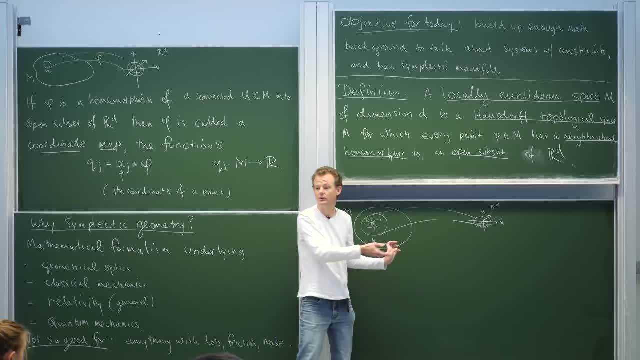 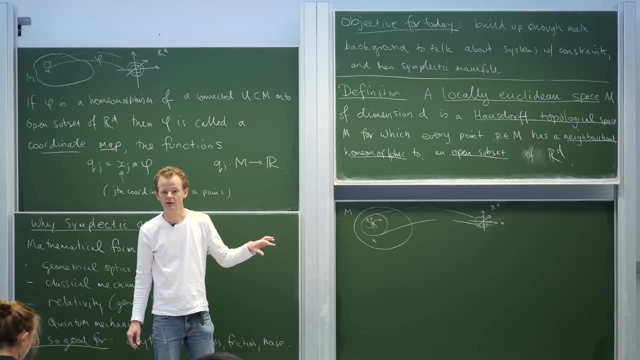 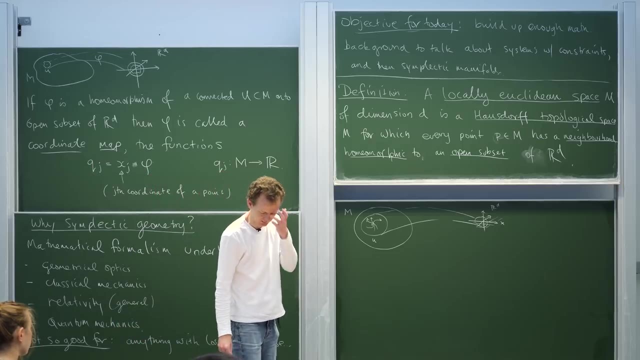 This coordinate system doesn't necessarily extend to the whole of the Euclidean space, of the locally Euclidean space. So it's a good coordinate system locally, but if you try and extend it all the way around then you might encounter problems. Now there's an example. you know your classical example. 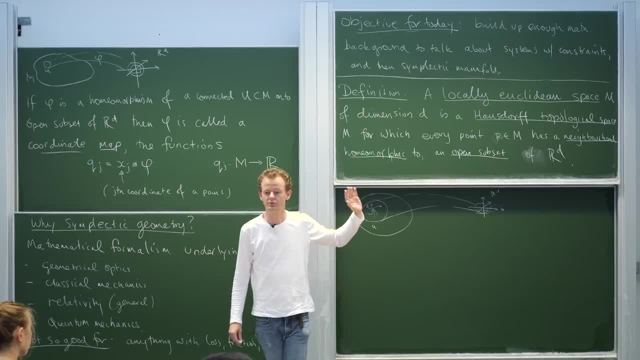 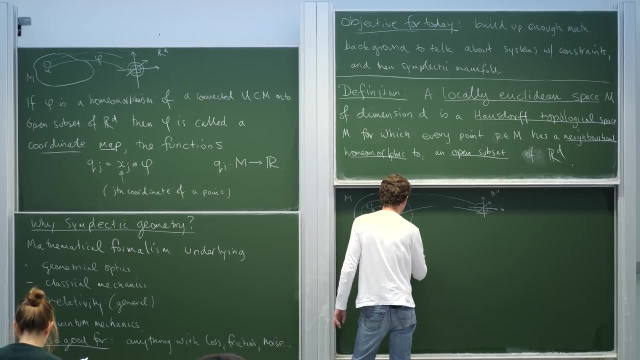 that we're going to return to throughout this course is the circle, or the sphere. This is a great example of a locally Euclidean space. Let's just take the circle. We're going to come back to it anyway. This is a locally Euclidean space. 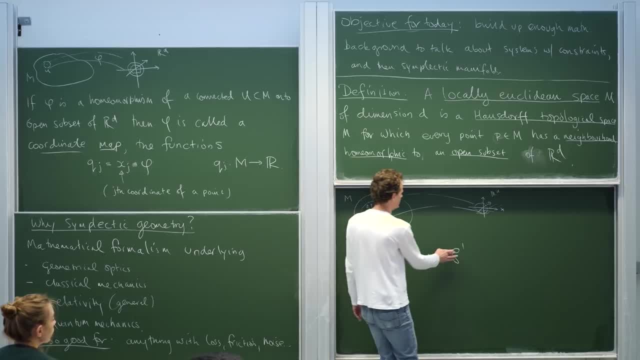 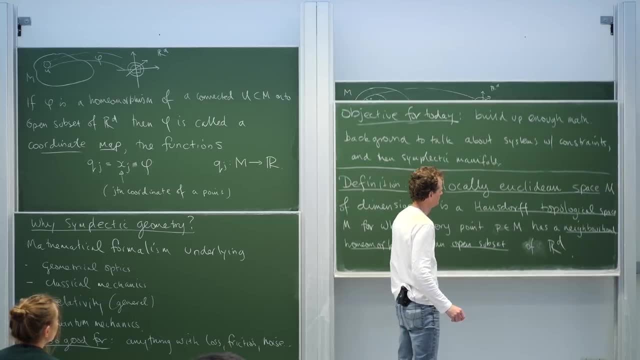 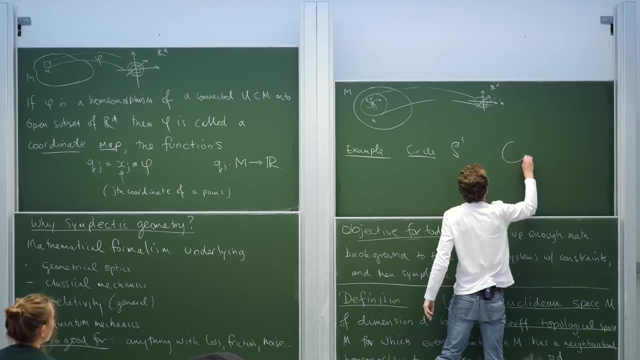 I think this is part of your first exercise sheet to do this properly. So I'm just going to do a really vague, hand-wavy argument here. Circle: is it a locally Euclidean space? The answer is yes, of course. So here is the circle. 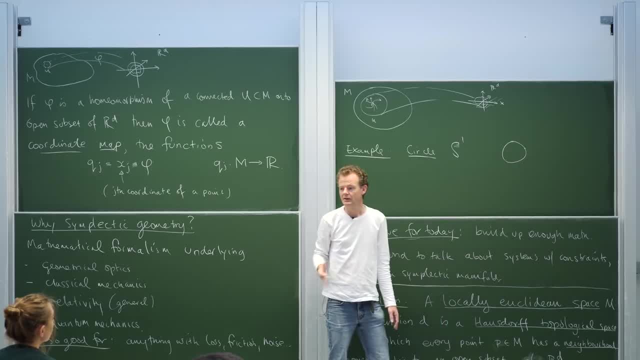 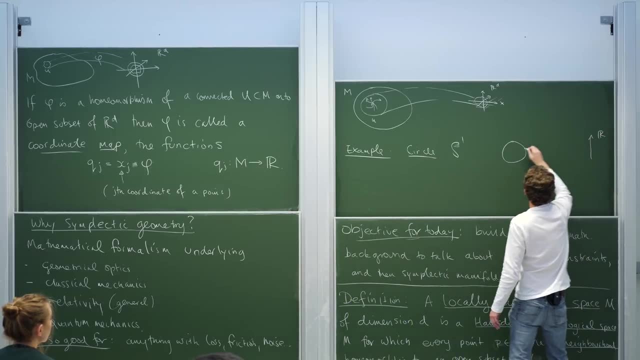 Let's just pick a point on the circle, say here, Is it homeomorphic to an open subset of R? Well, yeah, indeedy, All right, just take some interval around your favorite point. There is a map phi That identifies each point on the circle. 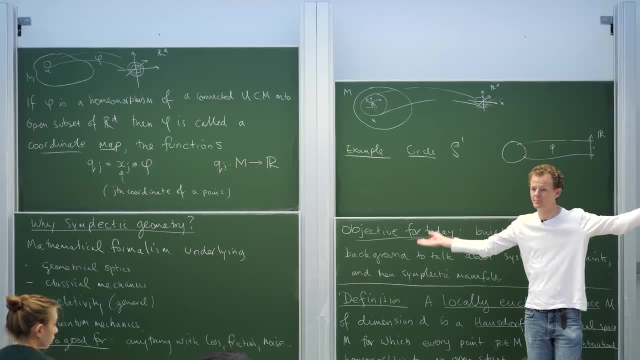 with the point n R like this: Can we extend this map all the way around the circle? Well, almost right, You can get it all the way. You can extend this interval all the way up to like just before these endpoints. 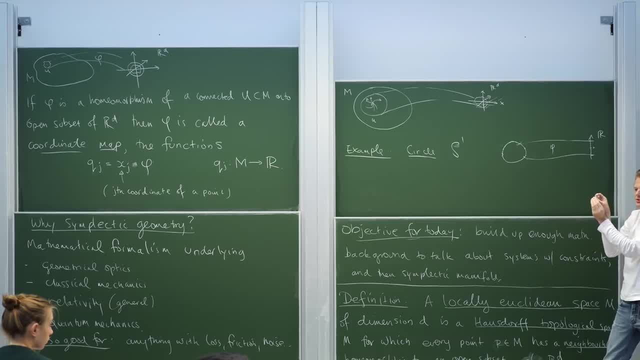 of the interval meet. What happens then You know: pop, they join, And that map becomes not invertible if you try and cover the whole circle. So the circle is locally Euclidean but not globally, globally Euclidean. The minute you try and extend this identification with a real line, 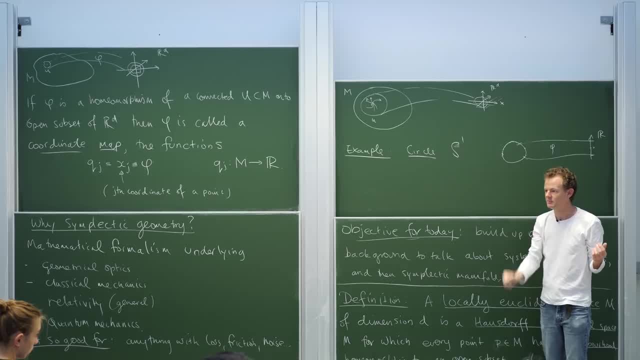 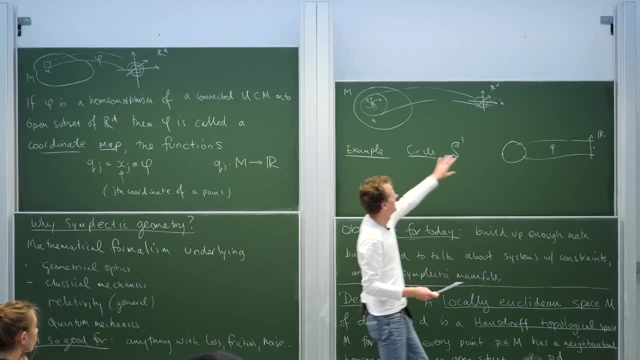 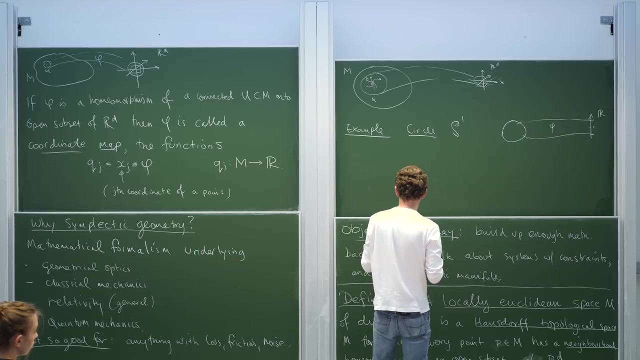 to include the last point on the circle, the map does not become invertible and is no longer a homeomorphism. So that's my. that's the example. You have to think about these things a bit more carefully in the homework sheets. but there's the moral Alright, so those functions. 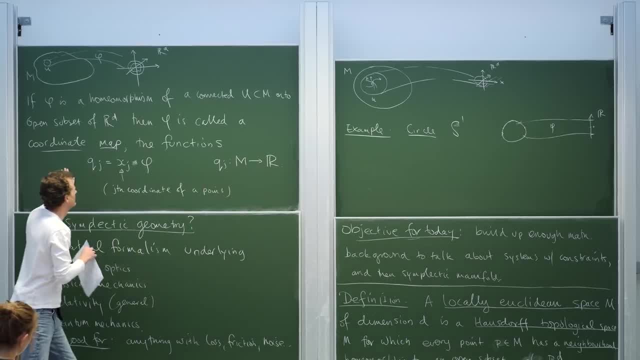 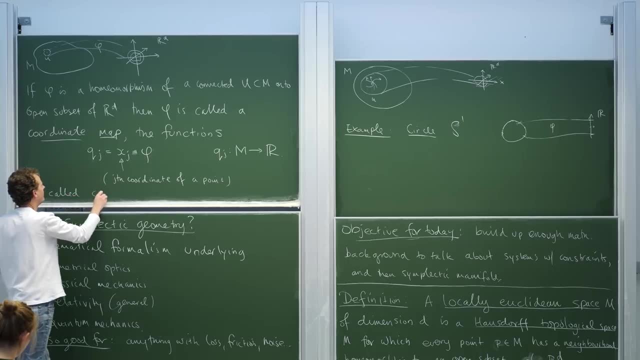 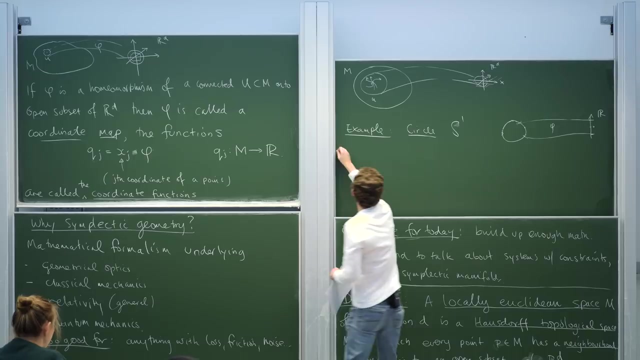 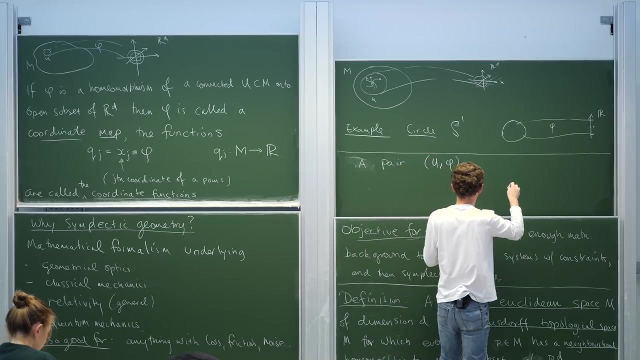 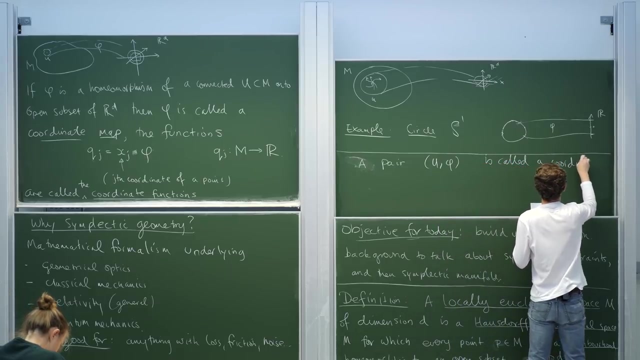 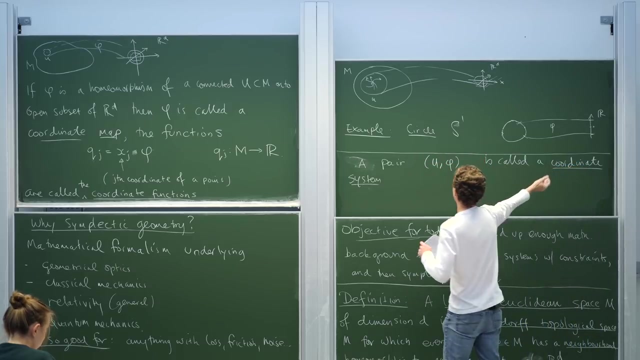 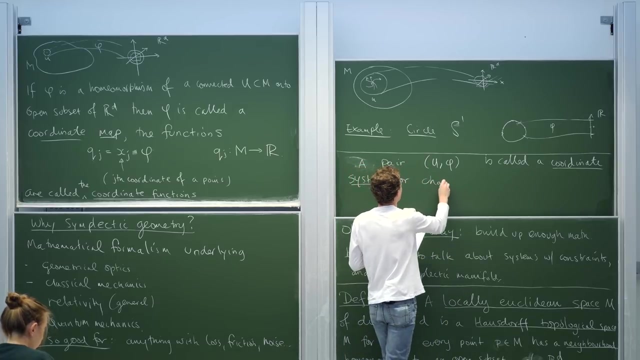 are called the coordinate functions- I got a bit distracted- Or say a pair, So such a pair of a neighbourhood in M and a map to the D. that's called a coordinate system Or, if you're a mathematician, a coordinate system. 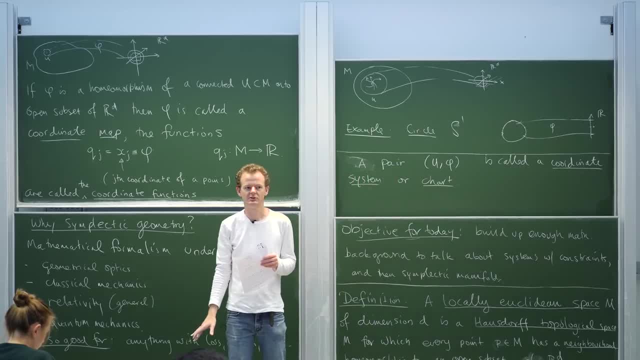 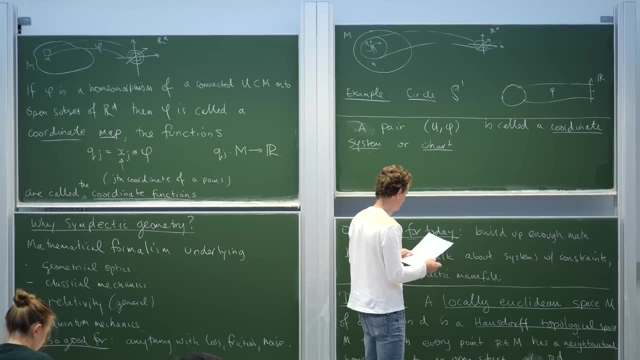 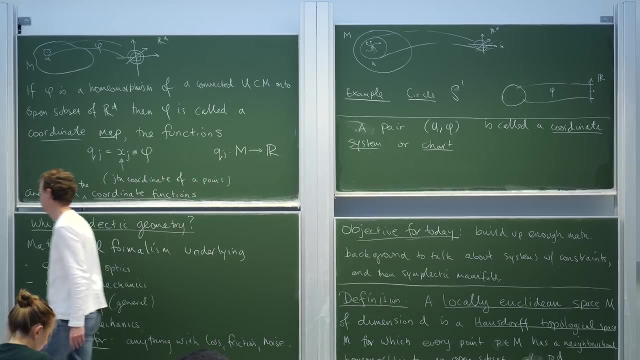 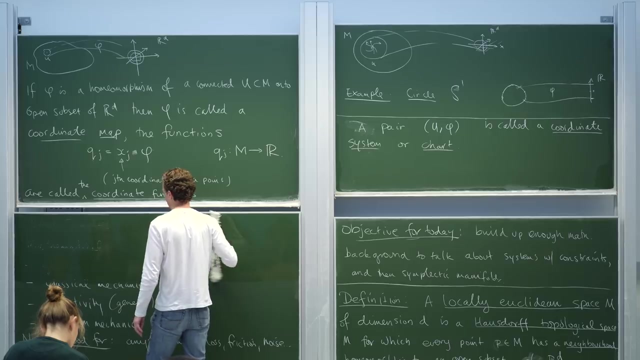 or a chart. Sorry, if you're a mathematician it's a chart, but if you're a physicist it's a coordinate system. Good Well, we got through that. It's not so bad. So Richard Feynman had many tricks to looking clever. 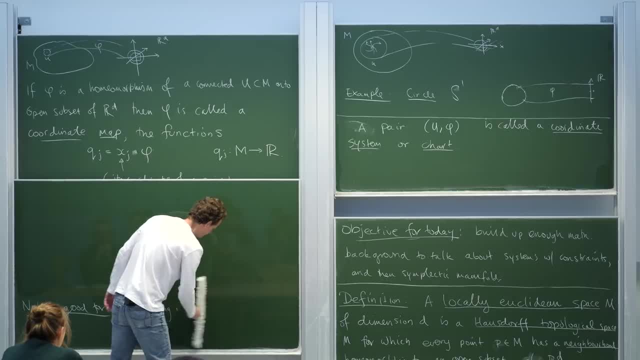 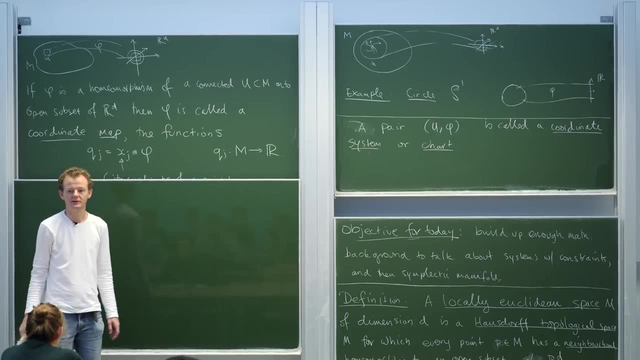 One trick was, in any talk or any lecture he would keep a very simple example in mind and test everything the speaker was saying on that very, very simple example as the talk proceeded. And then at some point in the lecture he might notice an incompatibility with what the speaker was saying in this extremely trivial example. And then 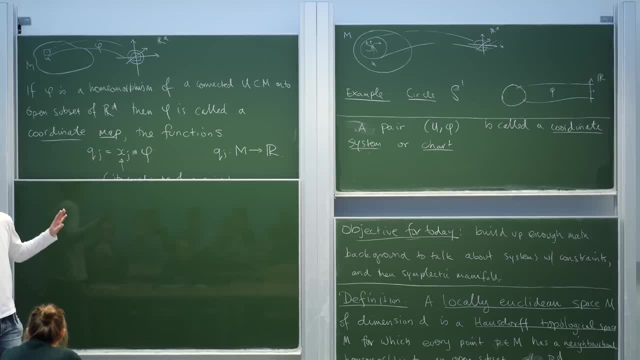 he'd ask some question that would seem extremely deep, as though he understood the entire material of the lecture. Of course, what he had noticed was an incompatibility with a simple example and what the speaker was saying, So I highly recommend that for the rest of this course. 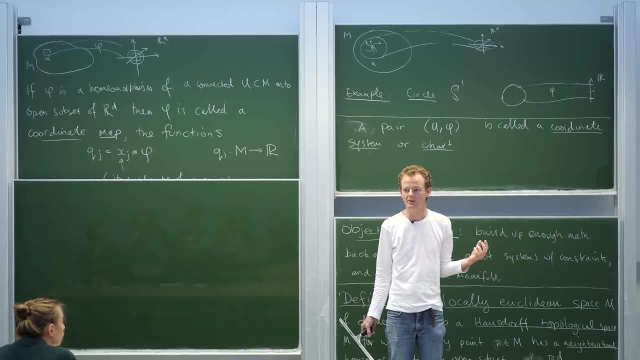 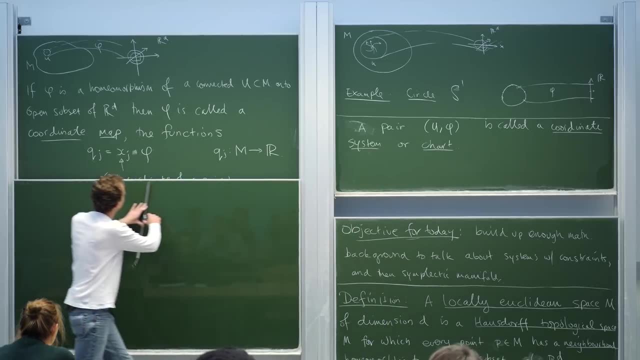 you keep the simplest example of a circle in mind, and that will give you the power to ask difficult questions when we get to more general theory. Certainly it's the example I always keep in mind when hearing about anything to do with differential geometry. Turns out, the circle is not really quite the best example. 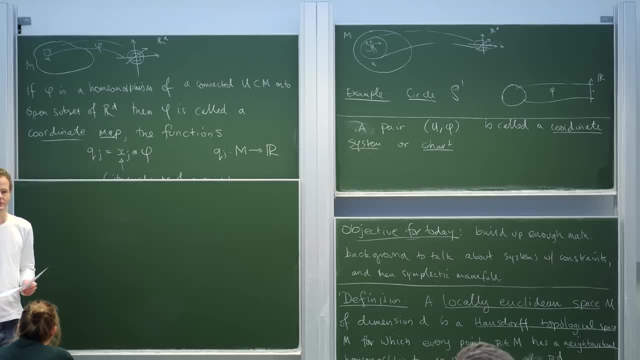 for symplectic geometry, as we'll see, There's a kind of a natural one, the cylinder. We'll get to that For this part of the course. the circle is a really good Feynman example, if you like. Now, up to this point, these maps, phi's, are just homeomorphisms. 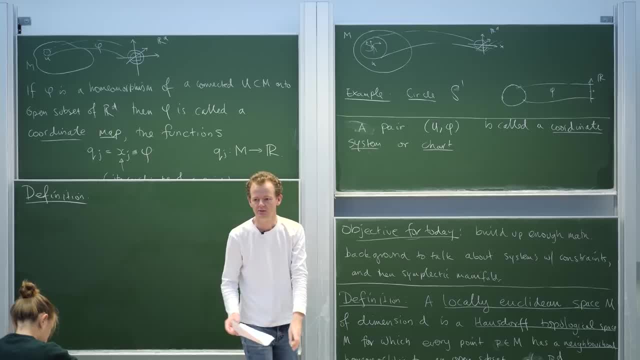 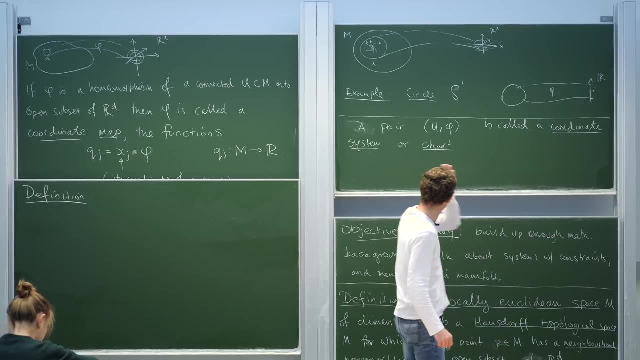 That means they're just continuous. Continuous maps are ghastly things. You don't want to live in the category of where the morphisms are continuous maps. These are vile, vile things. All kinds of horrible maps can be continuous. Cantor's staircase functions and blah. 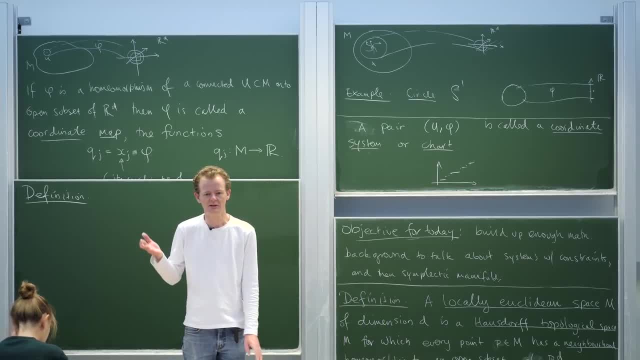 So continuous is not the place we want to be in physics. Nothing in physics leads us to think that it's continuous but not differentiable. Usually you can make a small change and it responds in a way to the small change. So we're going to get as quickly as possible away from 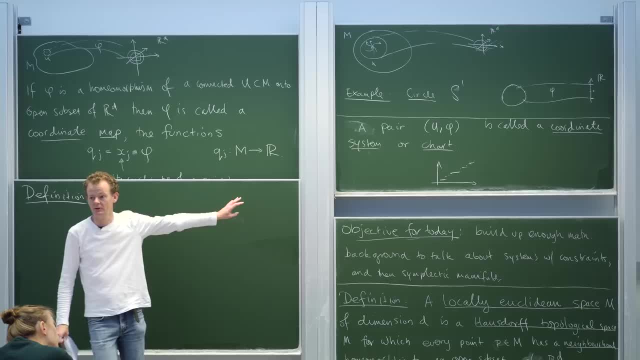 a category where we need to talk about continuous maps. I mean it doesn't mean that the maths isn't interesting. It's a super-duper interesting part of maths to study locally, including space, where you only have continuous maps and all kinds of crazy fractal stuff can happen. 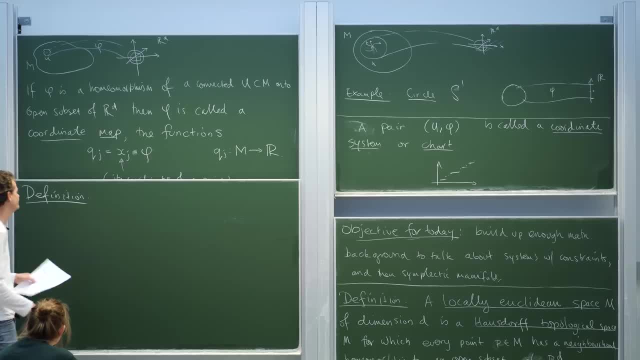 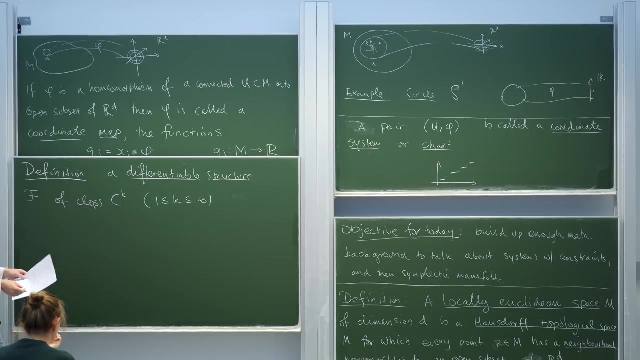 It's pretty nice, but it's not really relevant for physics. So let's throw away all those pathological examples And demand that everything starts to be differentiable so that we can take derivatives and not have them explode in our face. So a differentiable structure f of class c to the k. 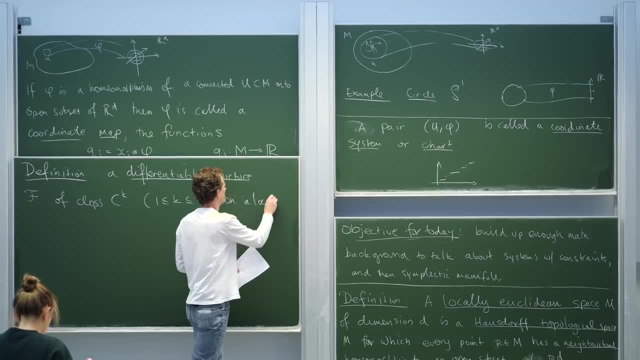 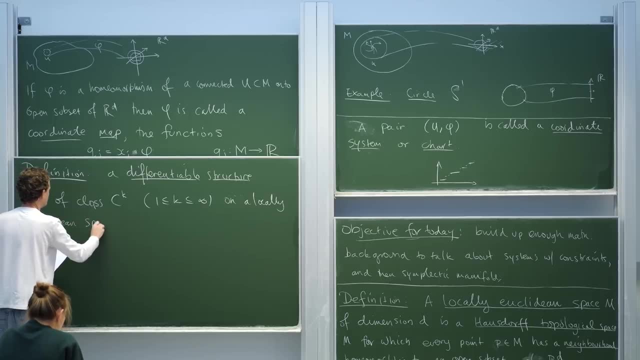 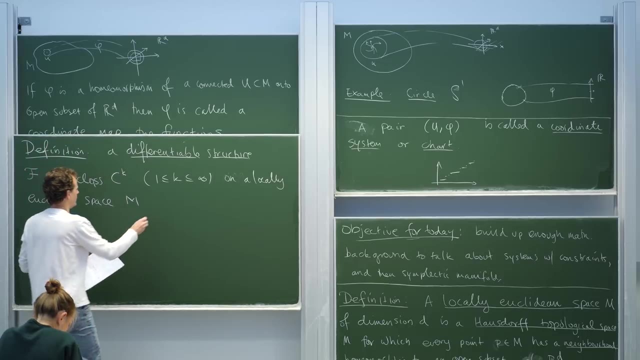 on a locally Euclidean space, some extra structure that we're going to put on top. What is it? It's a collection, It's a bunch of charts. 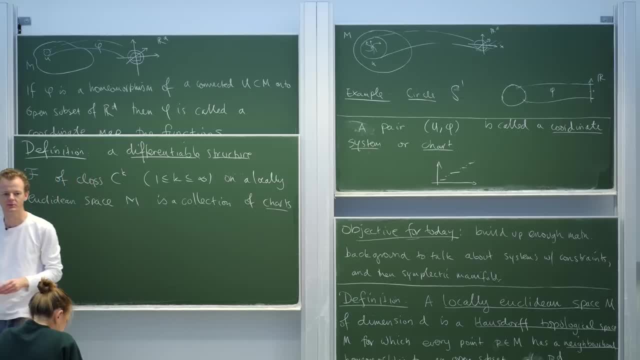 I just write charts instead of coordinate systems, because it's sort of shorter to write the word chart than coordinate system. every time Of charts it's a bunch of charts now, Not just one anymore, but lots U alpha, phi, alpha and these alphas. 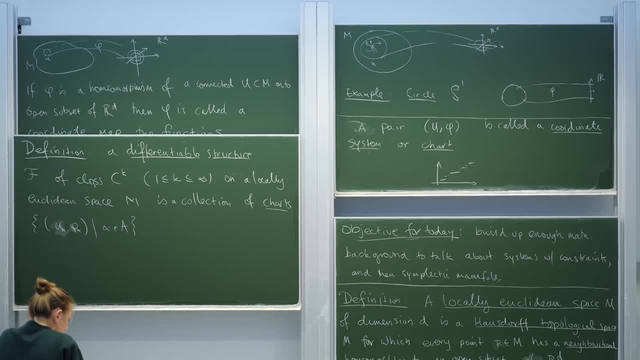 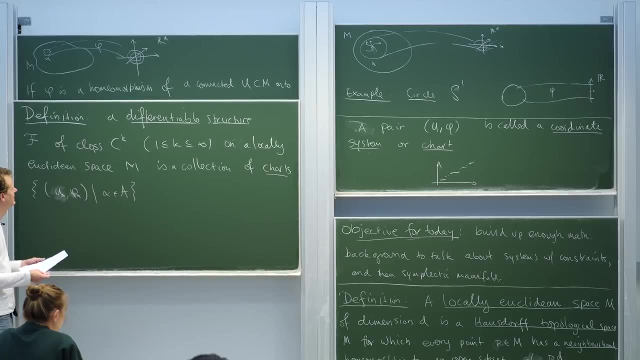 are running in some indexing set A. It might be a finite set, It might be an infinite set, It might be an uncountably infinite set of charts. So it's a bunch of charts satisfying some extra conditions. So condition one: well, nothing's missed out. 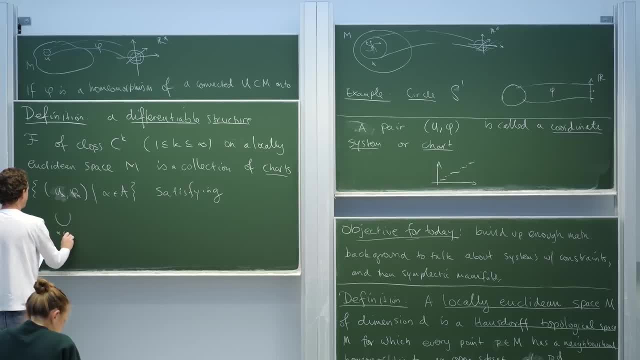 This is the simplest possible requirement we could have of a bunch of charts. Every point in M appears in at least one chart, So we're not going to miss out any points. That's a really mild thing to require of a bunch of charts. 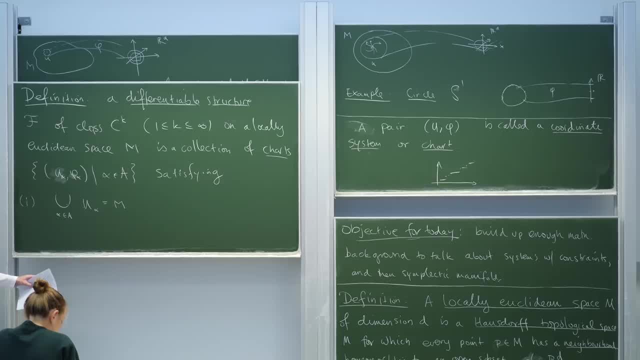 OK, It's a bunch of coordinate systems. At least we can assign coordinates to every point, Maybe not in every coordinate system, but at least in one coordinate system. And here's the more important one, That is that these charts, these coordinate systems, 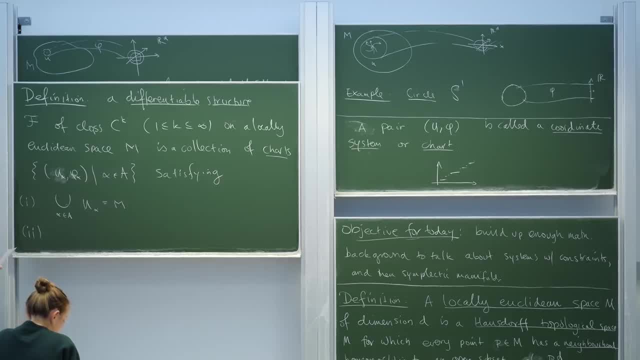 are in some sense smooth enough that we can take derivatives. And that's what this next condition tells us: that phi A alpha composed with phi beta inverse Is k times differentiable. Ck means k times differentiable. It doesn't mean the constant c to the power k. 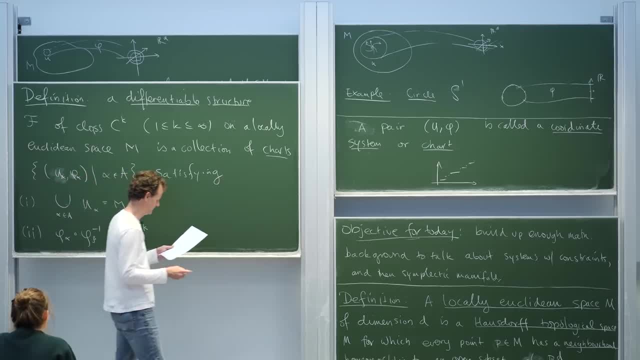 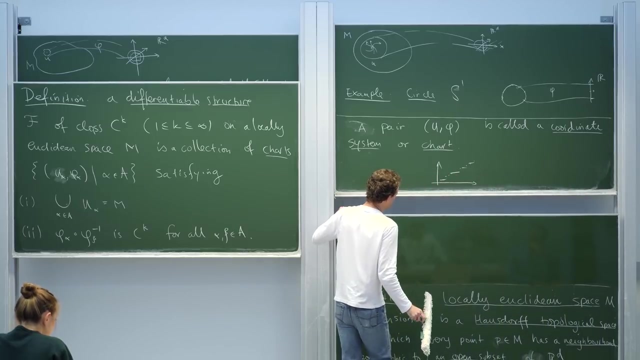 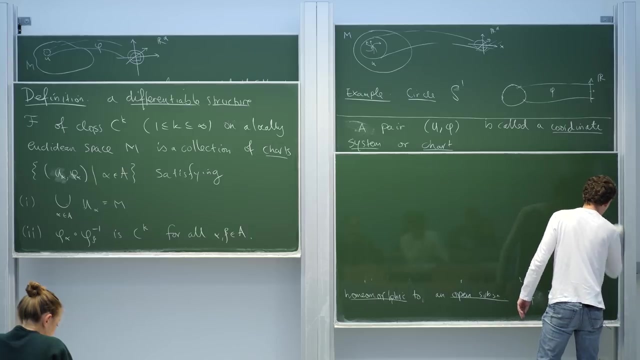 It really means k times differentiable, And there is going to be one extra condition. that will look completely bizarre, but I'll try and explain why that's there. Oh, I always start at kanske, And it's always going to be positive. 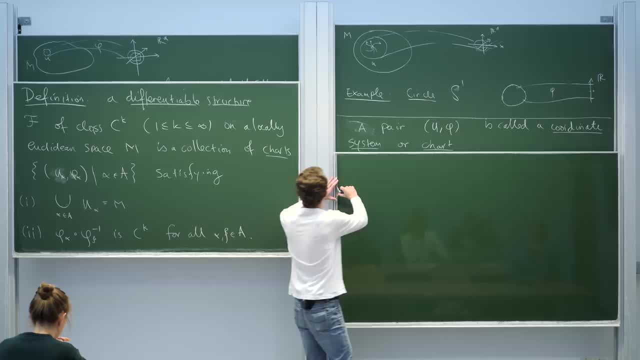 And I'm also going to most likely So think iniend games, where you have this thing that always goes up but it's also going to like go up, And that's where you've got a fastestаемся Mm-hmm. Look like. 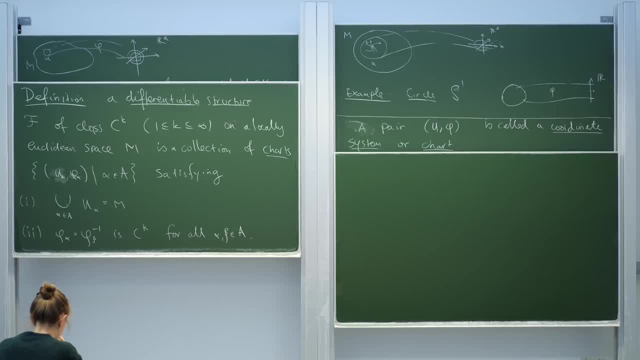 OK, Yeah, Yeah, Alright. third condition: Alright, this collection of charts is maximal. You can't add in another one. So this is not the way we usually do differential geometry in physics. Usually in physics you just get enough coordinate systems to cover your space. 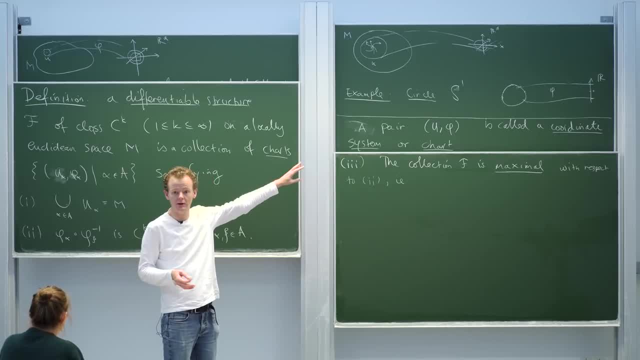 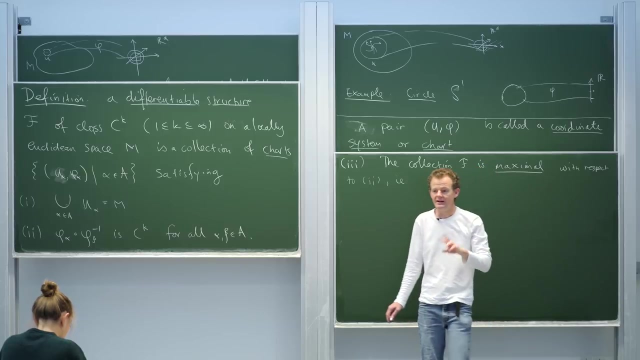 Like the circle. you only need two coordinate systems, as it happens, To cover the whole circle, And then you just do maths and calculations with respect to these two charts, But a differentiable structure. what is it? Well, it's not only those two, but any other one that's compatible with those two. 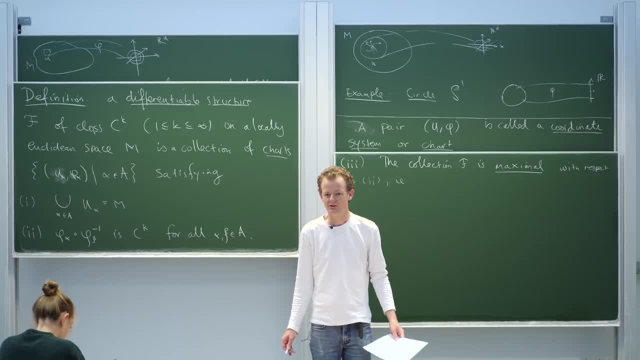 You have to add them in. It seems like unnecessary baggage, but it's there so that you get a unique object out at the end. Otherwise you don't have a unique way of talking about the differentiable properties of this. So this is like nitpicking. 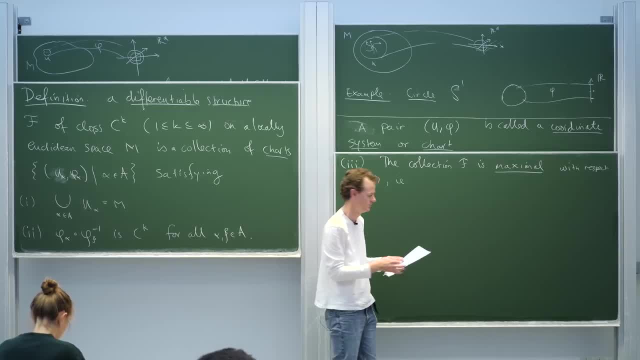 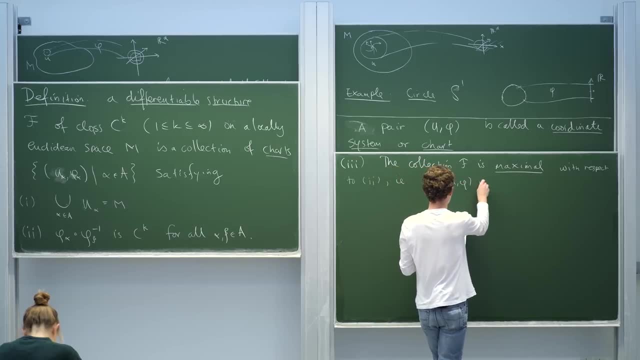 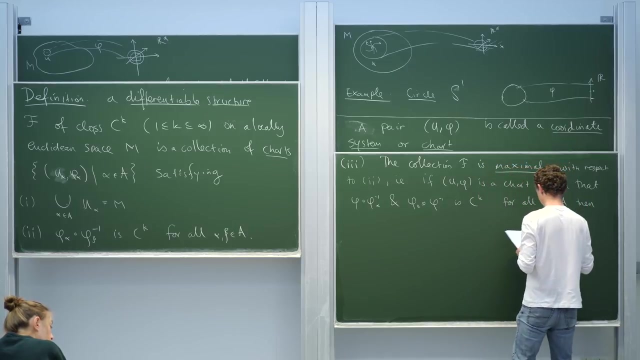 We're never going to use this third condition but we're going to write it down So it's maximal with respect to the property that if a chart has that these functions are c to the k, it's maximal. It's maximal Namely. these charts are sort of compatible with all the other charts that are there. 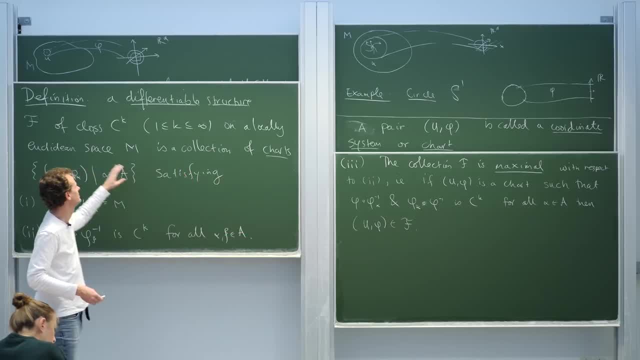 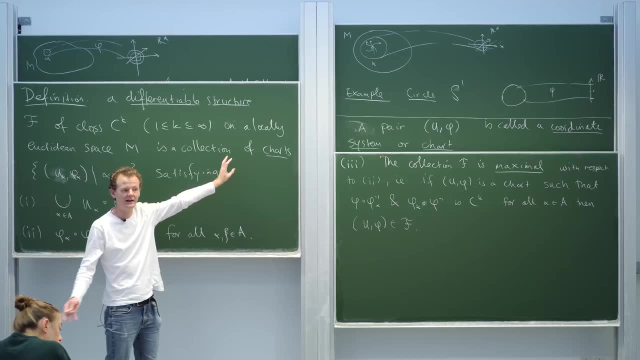 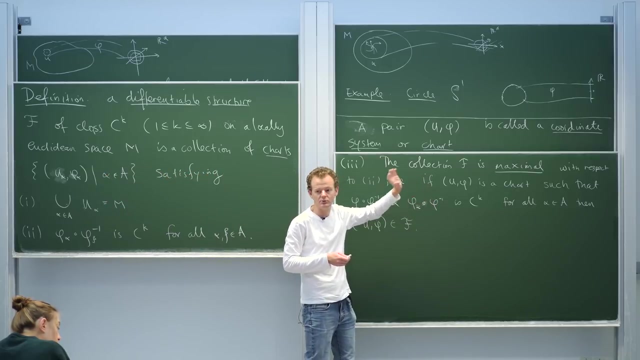 Then you have to add it in to this differentiable structure. So remember, a differentiable structure is a bunch of charts And it's a bunch of charts that's so big that you can't add in an additional chart, because it already contains all charts that are compatible to the level of k derivatives. 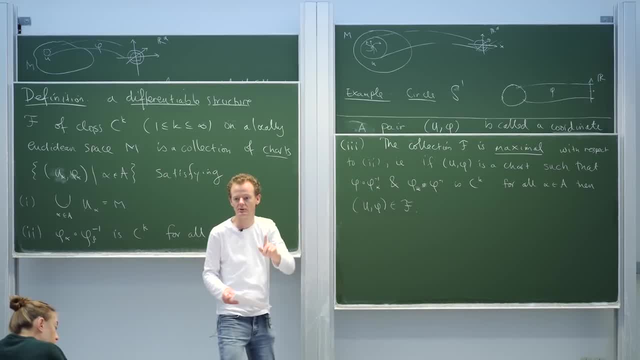 Now we're going to instantly forget this third condition. You have a question. So the question is: is it possible to have two differentiable structures? It sure is. Manifolds can have Locally Euclidean spaces can have different differentiable structures. 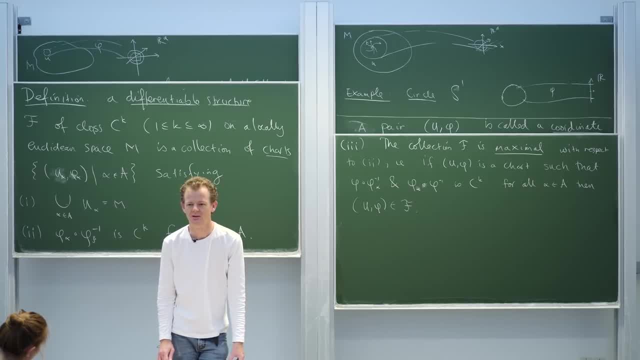 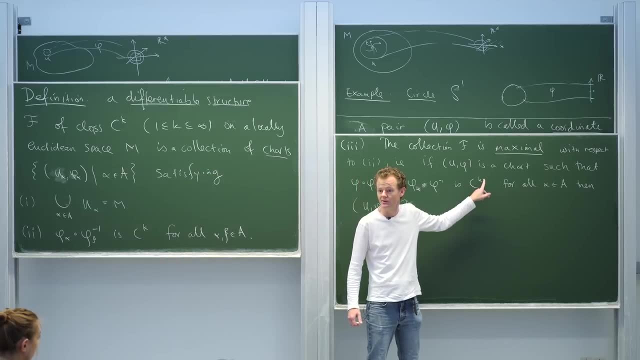 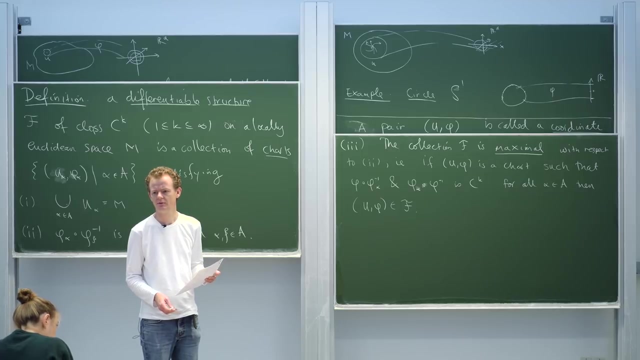 That's sort of Particularly when k is low, When k is like 1 and 2, you can get different structures. I will leave that as a very challenging exercise. This is not trivial, I think phi cubed- I think the real line- can have, if I remember it correctly. 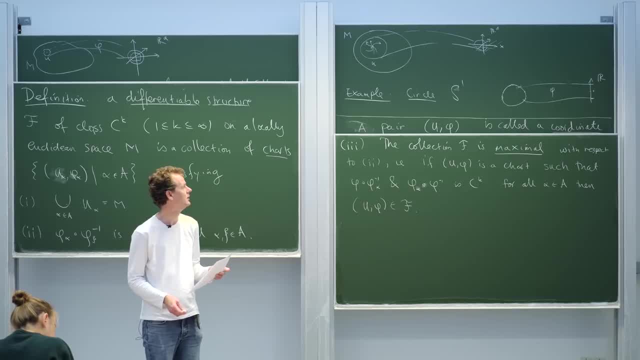 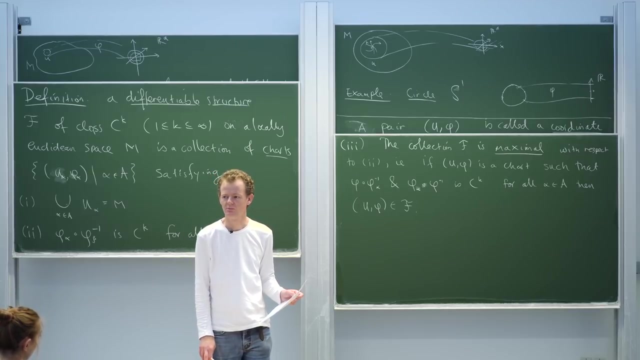 the real line has more than one differentiable structure and the map is like phi x cubed or something that gets you from one differentiable structure to another, But that's what I have in my memory as being the example. I see people nodding. 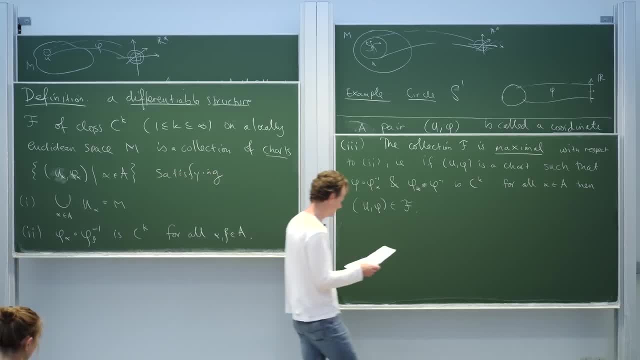 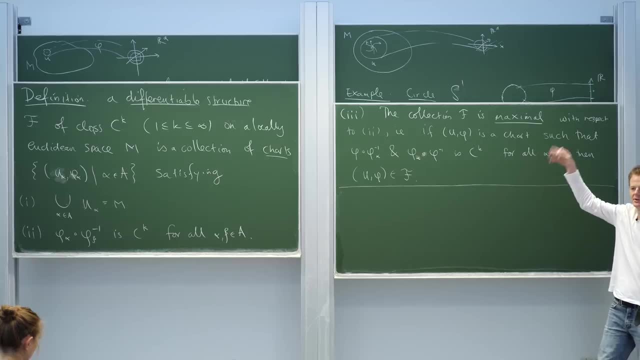 So people obviously more familiar with this material than me seem to agree That's good. Now, as I said, we're going to make this condition, then we're going to throw it away. We're not going to think, Because we're always going to work with just one or two charts. And why does that work? Well, once you've got a couple of charts, then you just keep adding in until you can't add in anymore. So you more or less specify the differentiable structure once you've specified charts that cover a manifold. 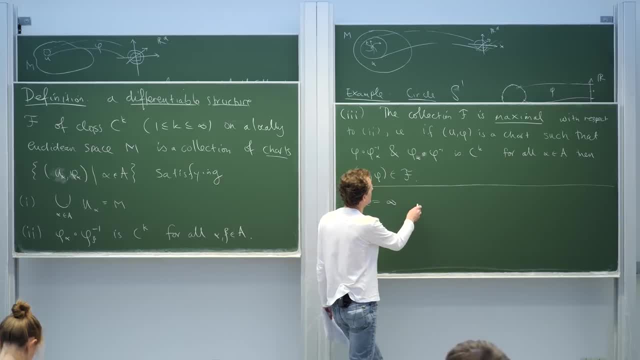 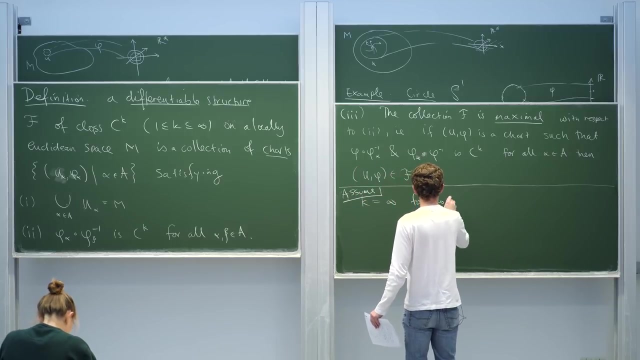 Oh yeah, And what else are we going to assume? Well, we're going to assume that k is infinity pretty much throughout the entire course. But- and I want to stress this- in physics our equations of motion are usually second order or lower. 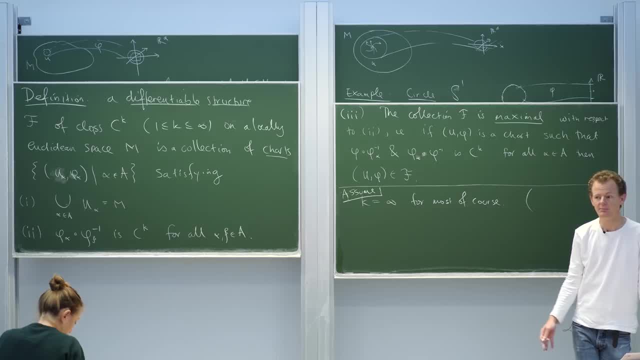 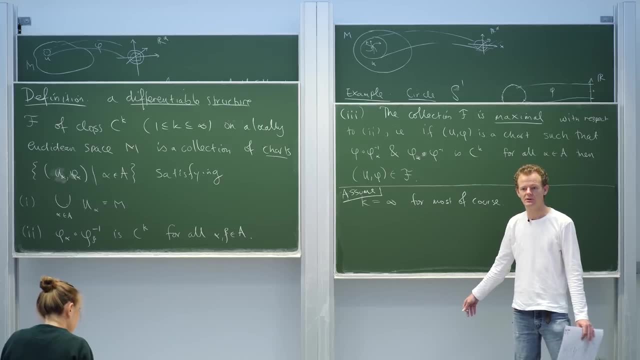 So actually everything we can say could be maybe true at the level of second order differential equations or even first order. If you go to weak forms and fluid mechanics and stuff, you might be able to specify all your equations of motion using only one-time differentiable functions. 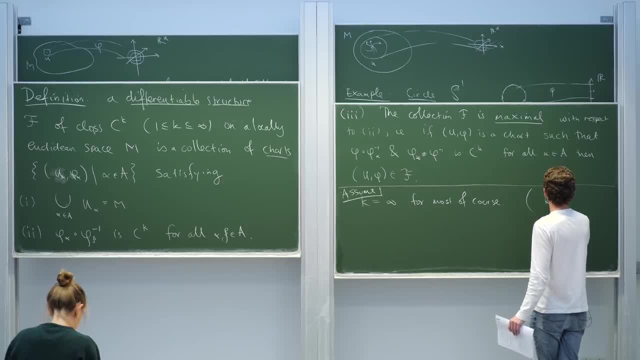 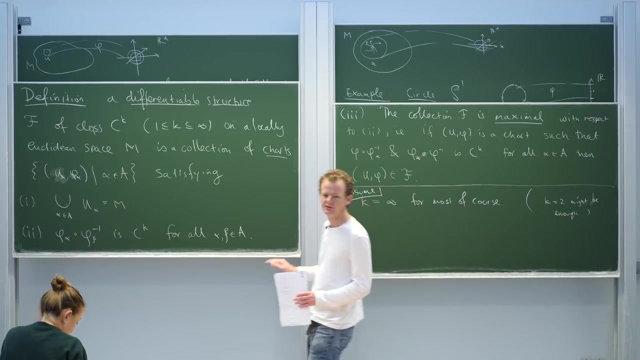 Life gets very complicated around there, And boy do things get interesting when k is one in two. So when k is like three and above, stuff starts to get pretty boring. But around k is one in two, where you have continuous functions and just one-time differentiable functions. 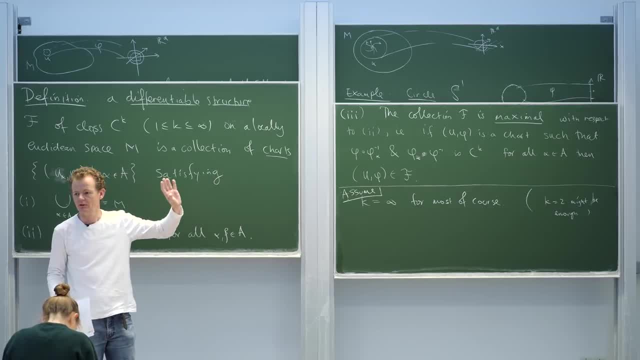 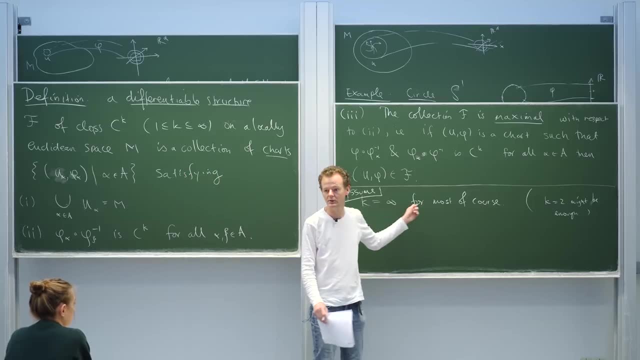 then you can get all kinds of different structures. But I'm just quoting that as an interesting thing to keep in your mind that nowhere in physics does it really say things have to be infinitely differentiable. That's us wanting to make our lives simpler. 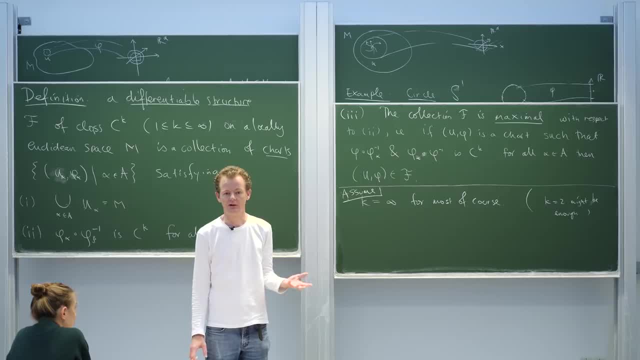 And indeed, certainly if you think in terms of fundamental physics, it's not even clear that things should be differentiable at all If you take seriously the idea that the holographic principle, for example, that space-time itself should be comprised of a finite collection of degrees of freedom. 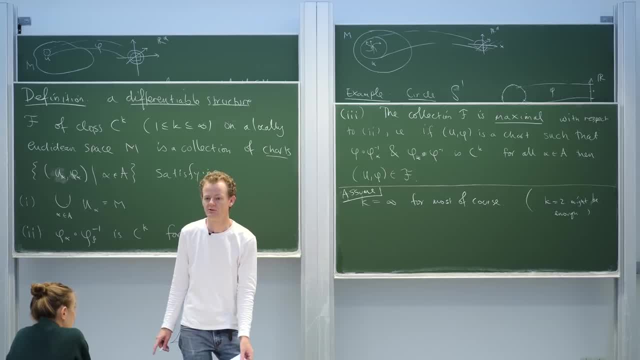 and that's not even continuous differentiable. I mean these concepts completely break down at the Planckian level. So this is all an approximation to perhaps discrete things lying under the surface. But as I said, for this course we're assuming k is infinity. 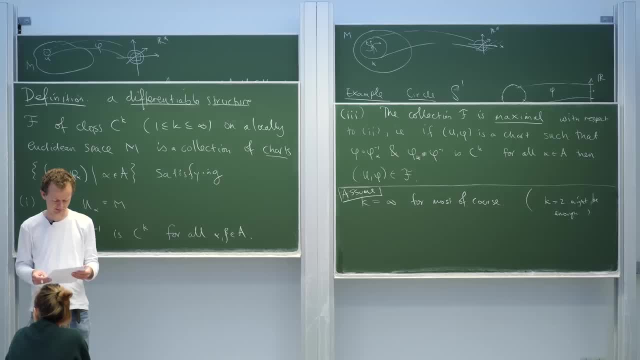 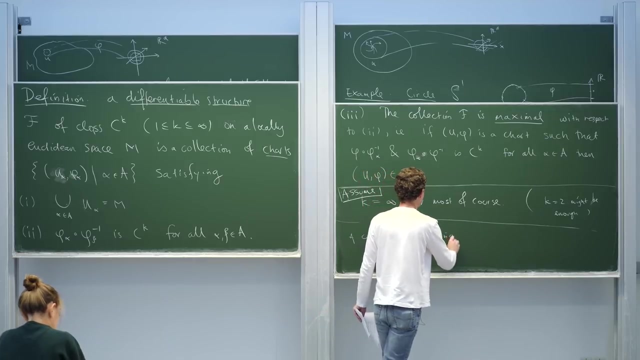 Maybe it's important that k is only two in some parts, but I don't think so. All right, another piece of terminology: A collection of charts obeying one and two. That's right, isn't it? Yeah, yeah, it's called an atlas. 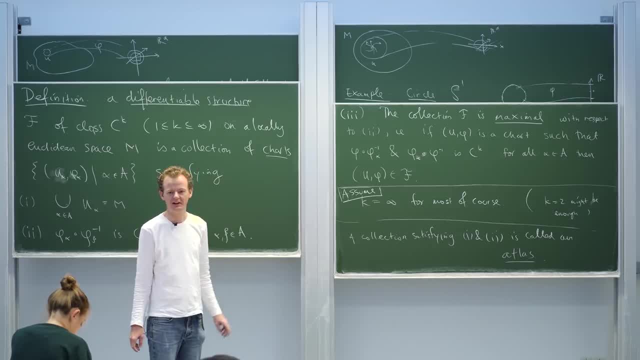 And the reason it's called an atlas is because that's actually what you see in an atlas. When you open up an atlas of the Earth, then on every page you see a piece of the Earth. right, That's a coordinate chart of the Earth. 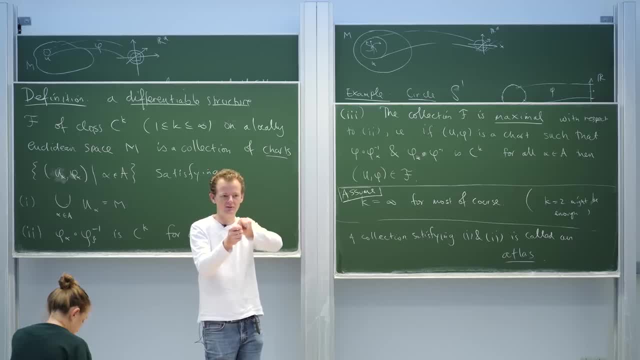 And these coordinate charts, they smoothly depend on each other. You turn the page and see another part of the Earth, And then, if you turn the page backwards and forwards quickly, you can sort of see how one point on the next coordinate chart is mapped continuously or even differentially. 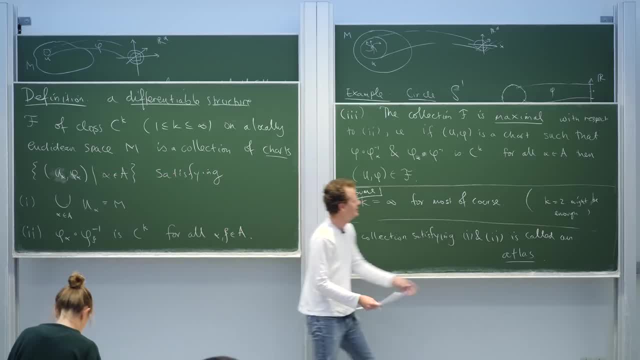 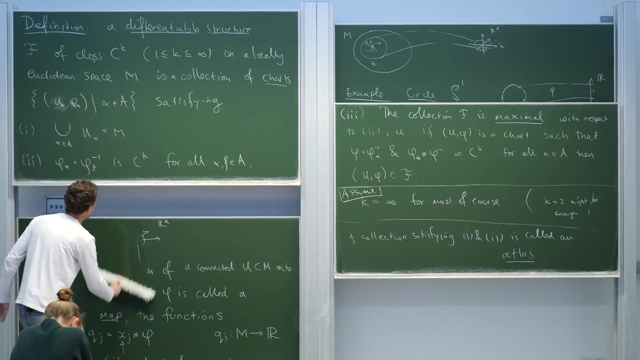 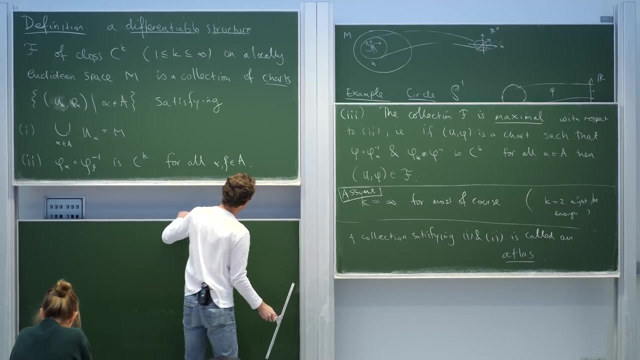 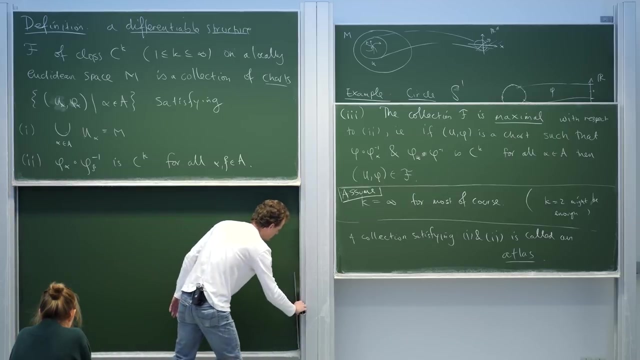 with a point on the previous chart. So you know that's a really nice definition, because the word here evokes exactly the content of the definition. So I'd certainly be remiss if I did not draw that picture of underlying this definition. 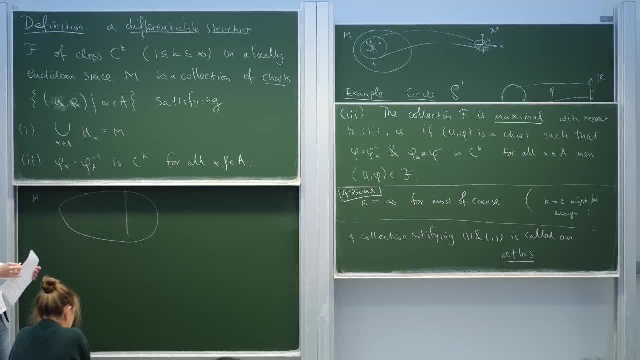 Here's M, our locally Euclidean space, with a differentiable structure F, And the pieces in this definition are usually illustrated, in any book that you care to obtain, in the following way: So we have a U alpha, We have a U beta. 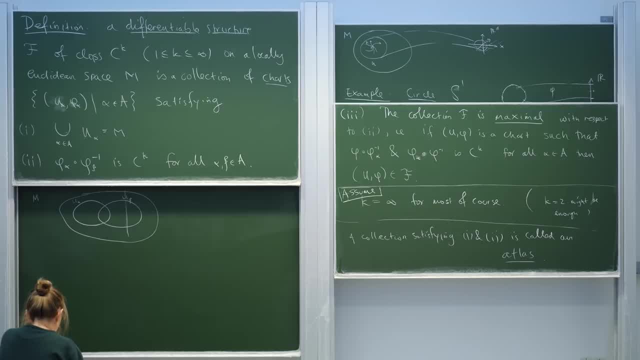 These two neighbourhoods intersect. They have a nontrivial intersection. Now, what is a coordinate chart? Well, it's a map phi alpha, from the neighbourhood to some nice Euclidean space, And I'm going to colour in this bit that's common to these two charts. 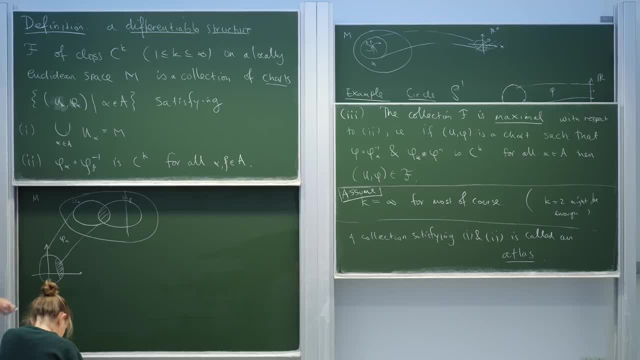 And so that bit looks like this in this coordinate system, this chart here And then this chart here is also mapped onto another Euclidean space, another copy, if you like, by phi beta. And now let's look at this thing here. 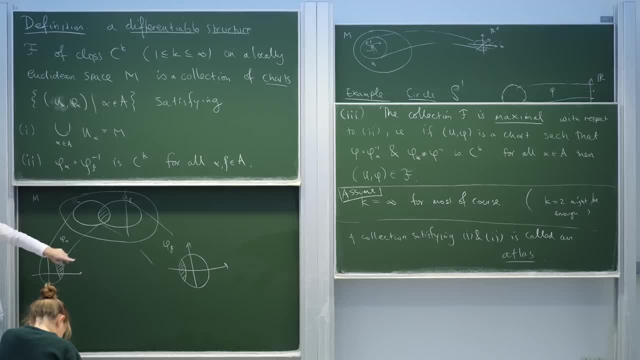 Phi beta inverse composed with phi alpha. What's this thing doing? Well, that's a map. Well, what is it? a map from and to right. This is very easy to get confused in differential geometry, so we do this slowly and carefully every time. 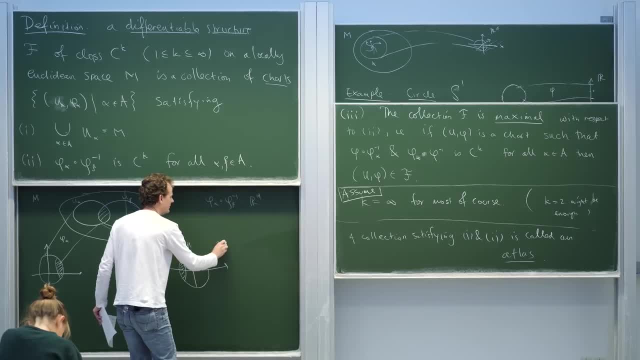 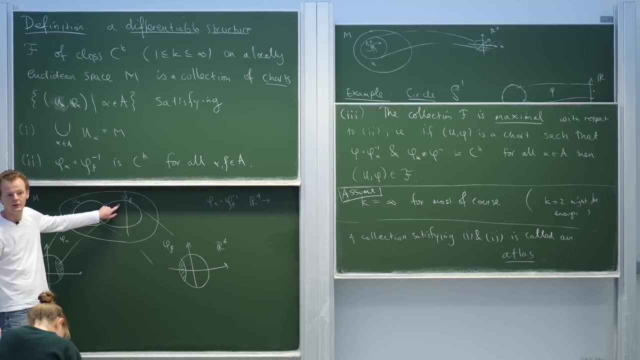 That's a map from R to the D, in particular this R to the D. Well, phi beta inverse goes from R to the D to M And then well, where it's defined. I mean it's not defined here. 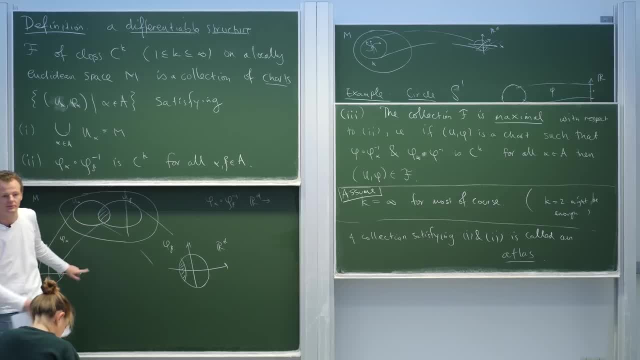 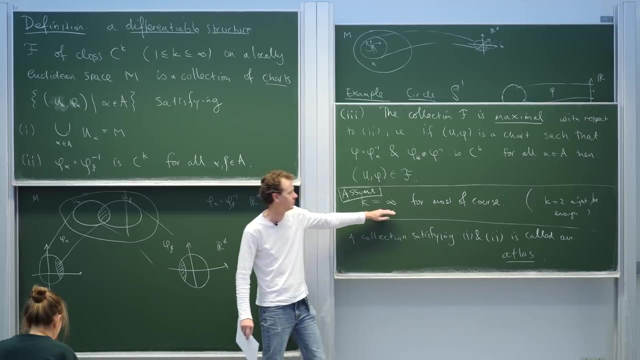 it goes then back to R to the D again. So this is a map from R to the D to R to the D, And we're demanding that this map is k times differentiable, or, since we're making this assumption, infinitely differentiable wherever it's defined. 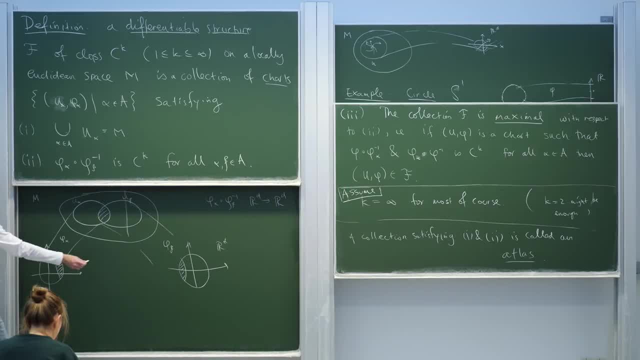 That's what we're demanding. So in this little coloured chart, this little coloured in patch here. so on this coloured in patch here to here. oops, there's got to be an inverse. It really doesn't work. That's got to be a super smooth, differentiable map. 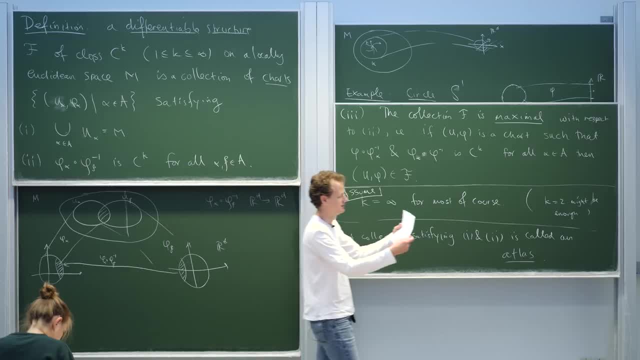 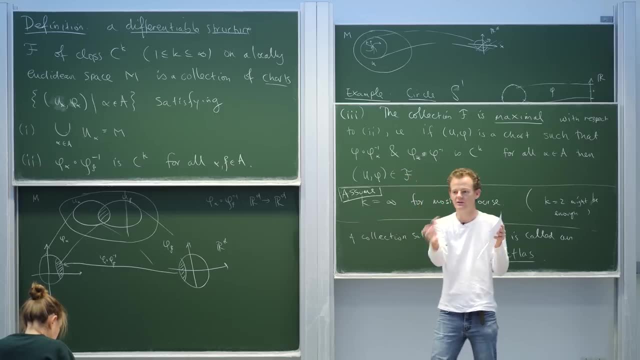 And, as I said, you look in the atlas, you open it up and you see Germany in the middle of the page and then it sort of the page ends around France, and then you turn the page. now you see France. 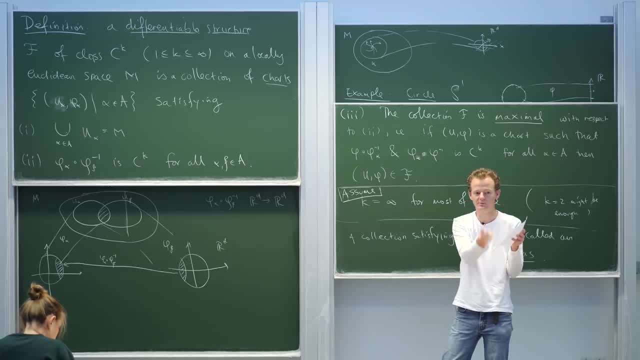 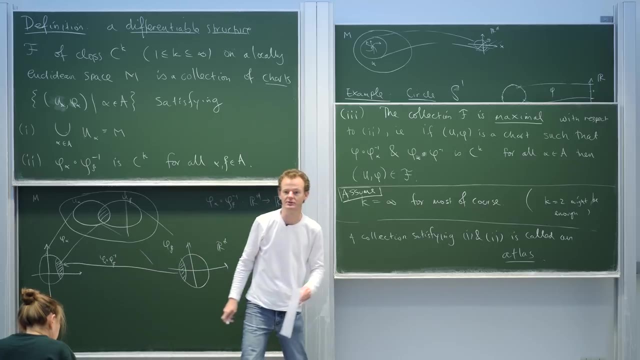 and you see a little bit of Germany. right, There's this overlap between that page and the previous page And it's a good atlas, because the bit where it overlaps is mapped nice and smoothly between the pages, That's these overlap or transition functions. 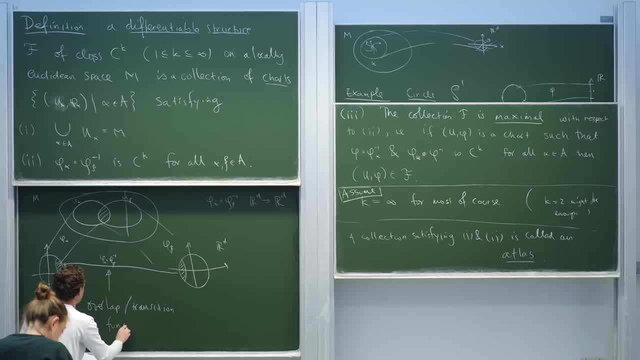 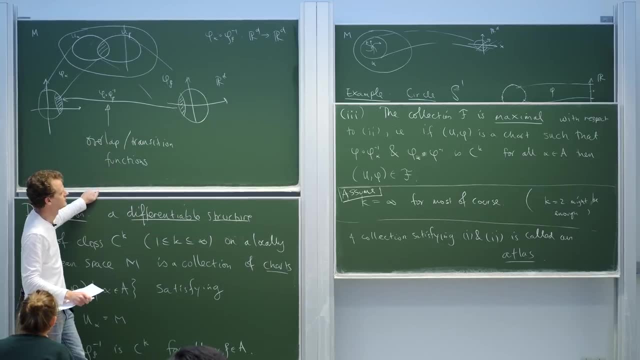 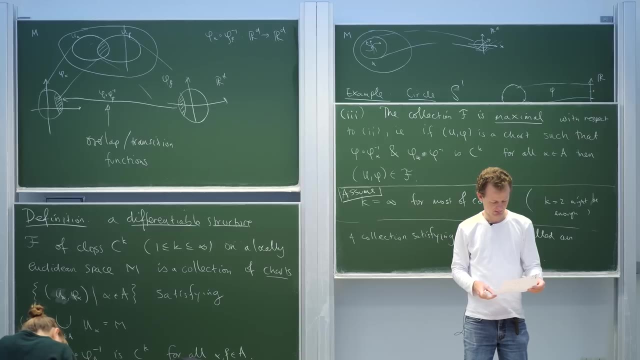 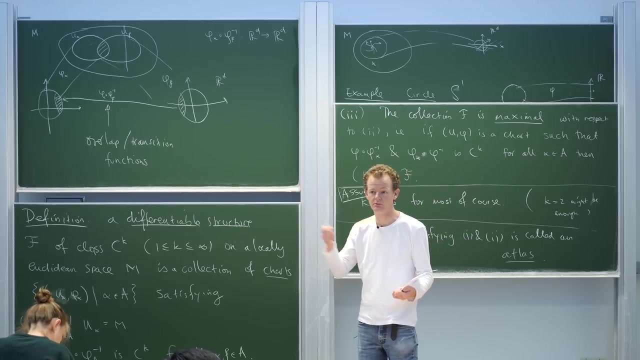 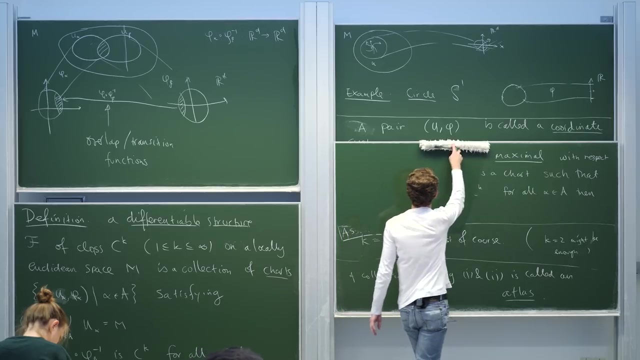 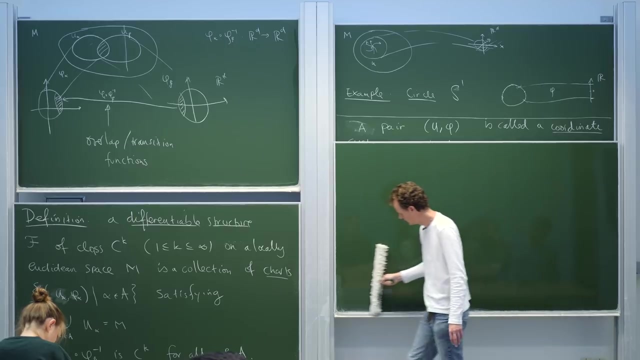 And I think we're going to end the lecture over the next half an hour with just a list of examples. Thank you very much. So a definition is a good definition if it captures all the examples you want it to capture, and maybe a couple more. 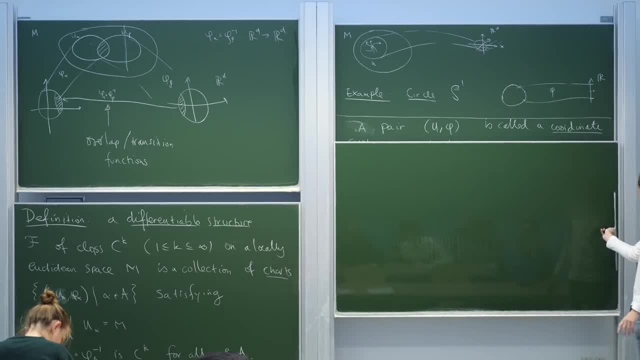 It's a bad definition if it doesn't capture all the examples you want it to capture or if it's so general that anything can satisfy the definition. So mathematical definitions is a kind of a Goldilocks zone: not too cold, not too hot. 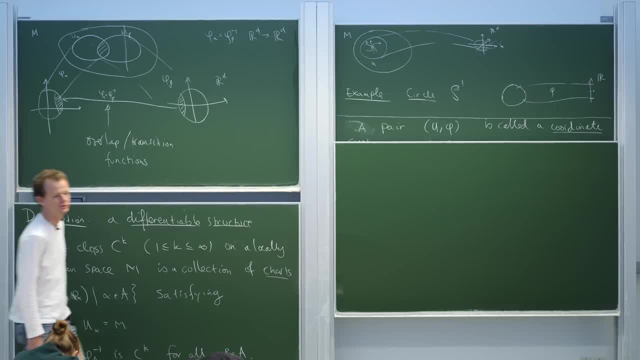 They just capture enough of the examples, but not too many, not too few. So to prove to you that this definition captures the examples we want in this course- and well, it's difficult to show that it doesn't capture too many, but it's certainly that it captures enough- 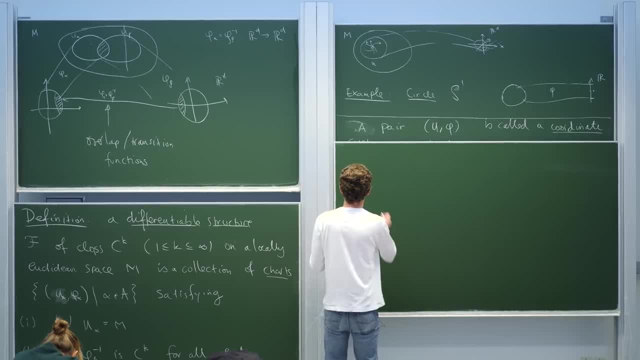 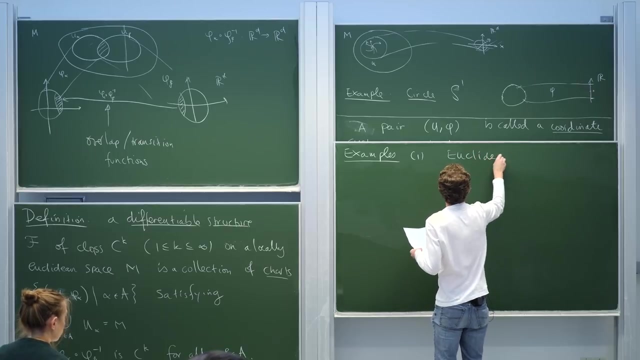 I'm going to go through some examples, And these are the most important examples for this course. Yeah, I guess I'm missing out on one example that's really important, but that's about it. So what is all this stuff meant? to generalize, 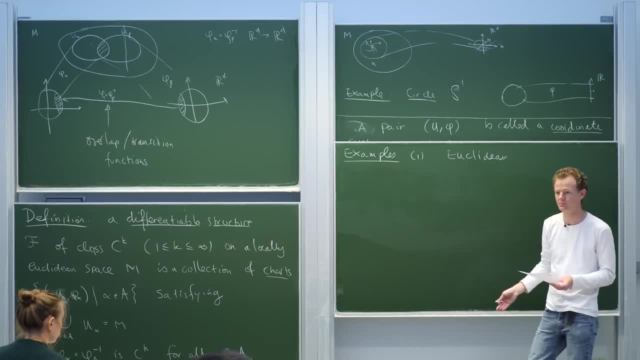 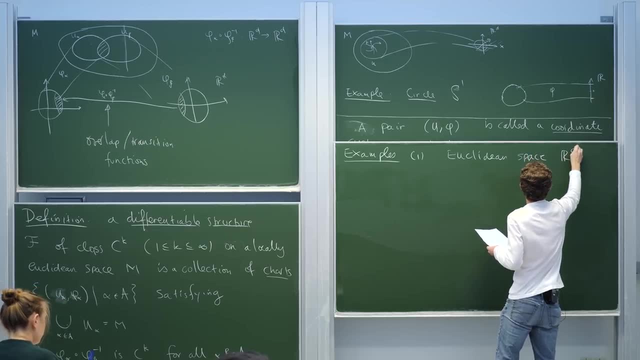 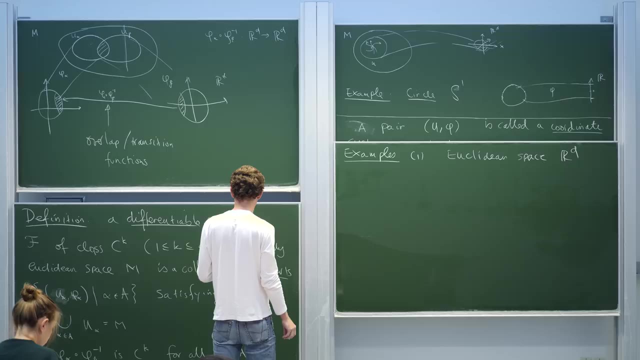 Well, Euclidean space. so it better be the case that Euclidean space itself is an example? If not, then wow, that was a really bad definition. Okay, well, yeah, it's a. Ah, sorry, I forgot to write down. 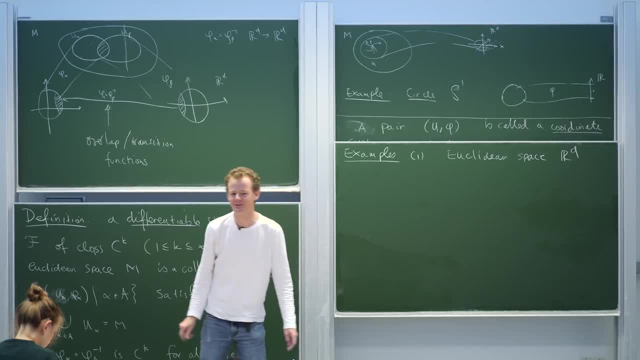 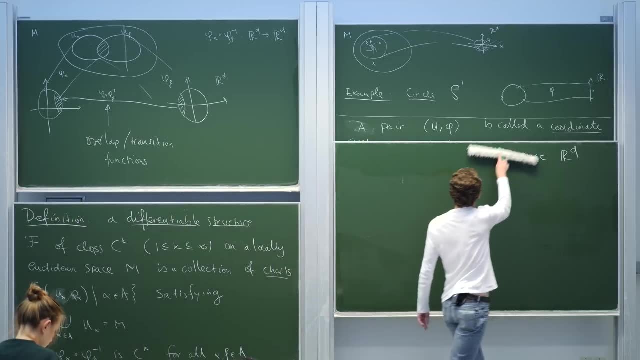 the main definition of a manifold. So before we can write down the examples, I got to tell you what a manifold actually is, And it's kind of clear right. We have this locally Euclidean space. we have differentiable structures, so a manifold is presumably something. 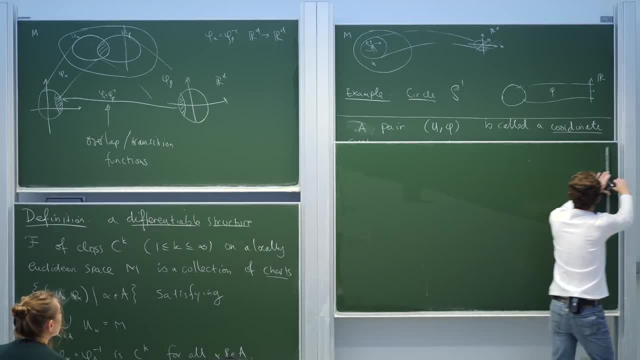 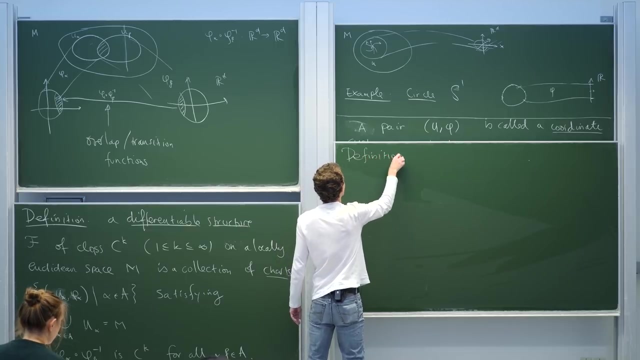 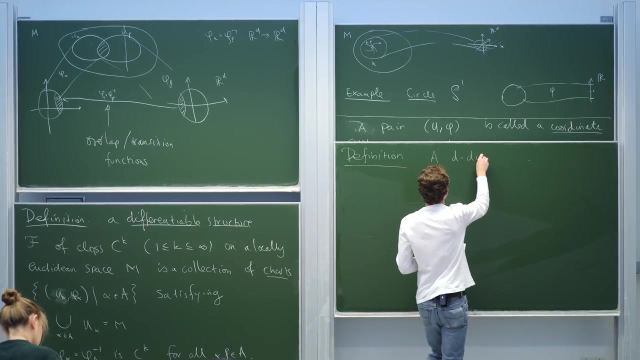 that's got both All right here. it is So a d-dimensional manifold. What is a d-dimensional manifold of class C to the k? Well, it's got to be a locally Euclidean space with a differentiable structure of class C to the k. 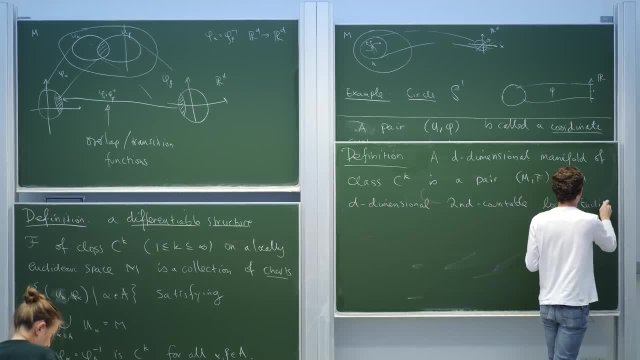 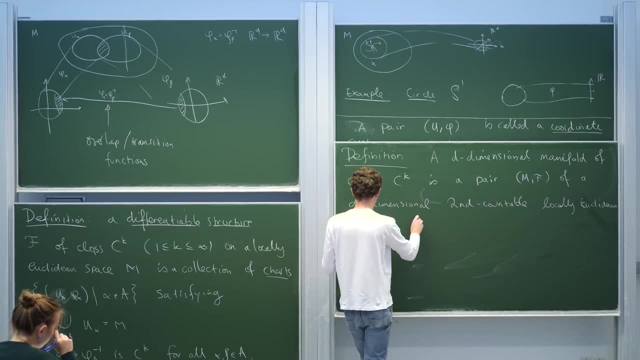 We have to note that within this one, there is a matrix which is represented here, and this matrix is the one that's always there, So the matrix is that's the matrix that's always found at the top of the circle- Now on the bottom of the circle. 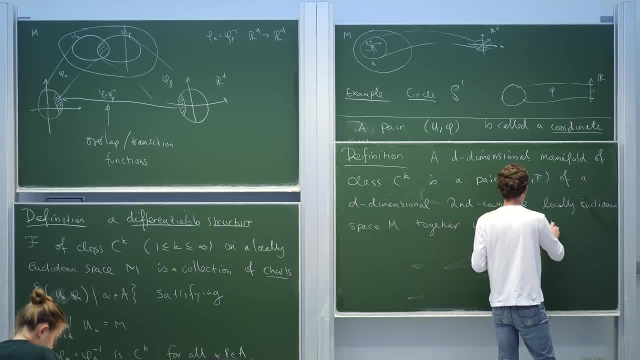 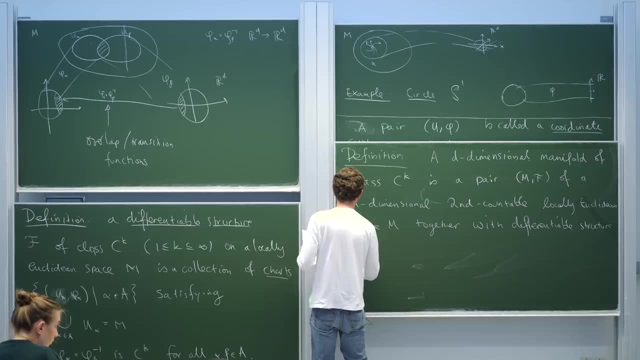 over there there is a matrix, And the matrix is the one that's always there, always trying to be, and means everything. Basically, when you have a matrix, it's the matrix that's always standing in a neutral room, And that's a very good definition. 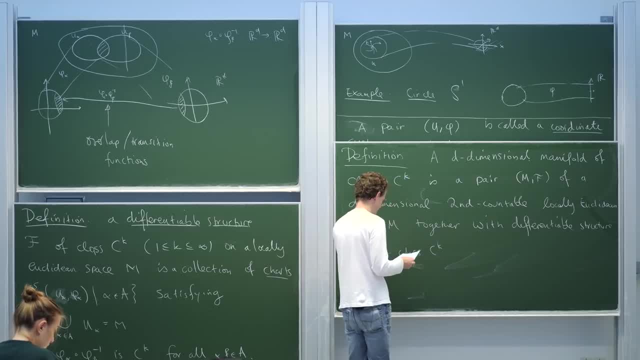 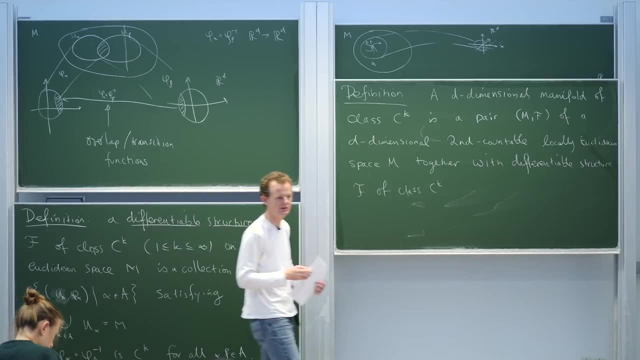 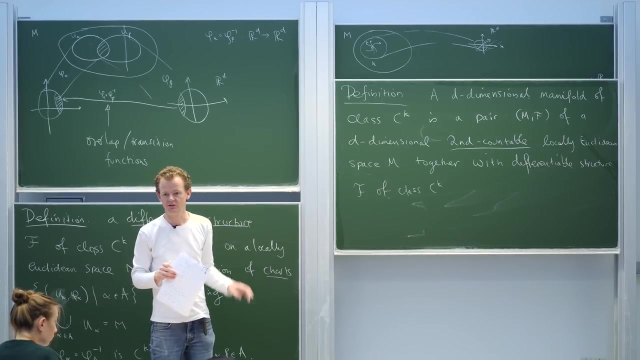 of a manifold. And then All right, there's one technical term that's sneaked in there in this definition: second countable. No examples we consider will get anywhere near not second countable. Second countable is like a technical condition that allows us to do integration on these. 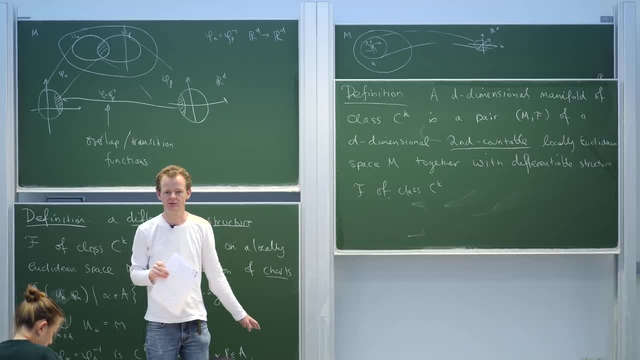 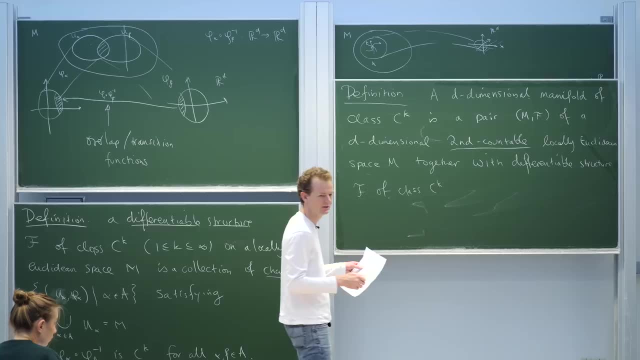 manifolds. It's really difficult to think of not second countable examples. but if you want to knock yourself out, there's a book called Counterexamples in Topology that'll show you no shortage of examples of not second countable, locally Euclidean spaces. 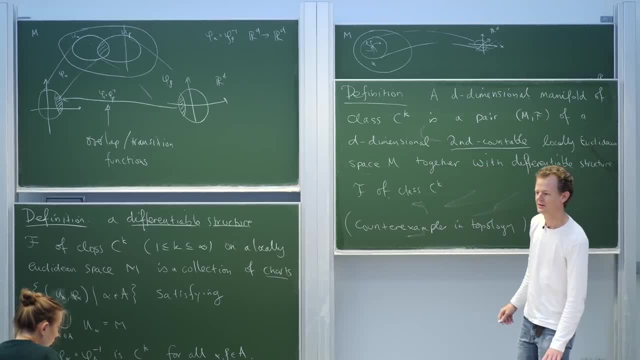 And I think this is like sort of required reading, a book like this in your scientific career. I think it's really vital that at some point you look at a book with the title Counterexamples in X, because it just shows you what happens if you're not careful with your definitions. 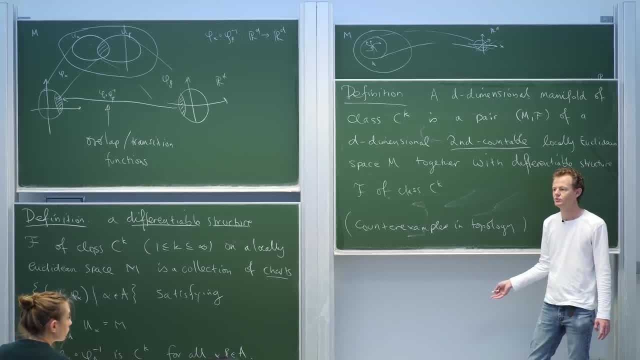 So if you make a definition and you think that you can draw conclusions from that definition- because this definition captures all the examples you know- right, and you know how these examples work- then you can be led to dangerously down the dangerous path of making wrong conjectures or even not being able to prove things. 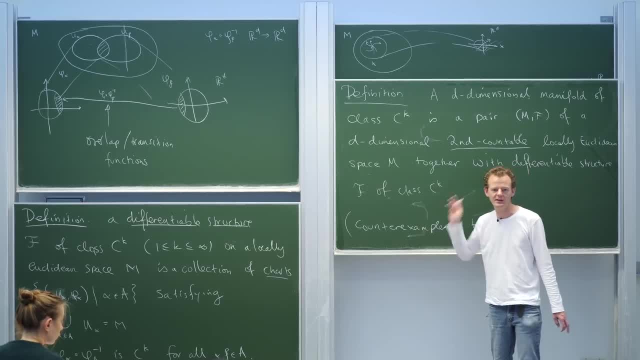 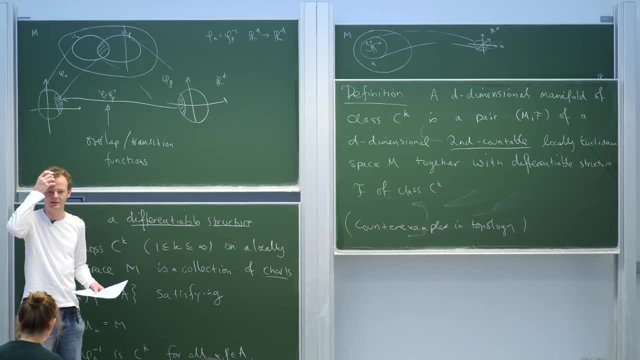 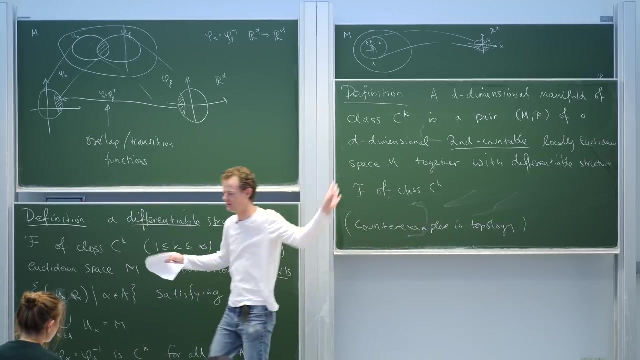 And so these books they present like the most pathological evil, things that satisfy various definitions. And you know, you think you might have a good imagination, right, because you can think up, like Harry Potter or something, But you know the people who write these books, they just live on another dimension. 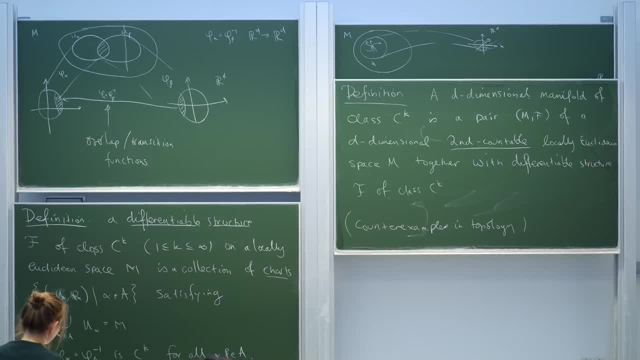 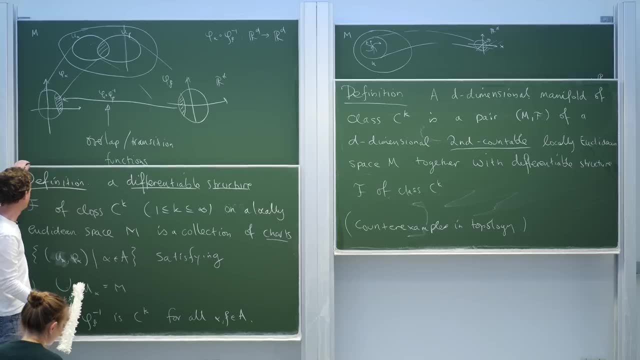 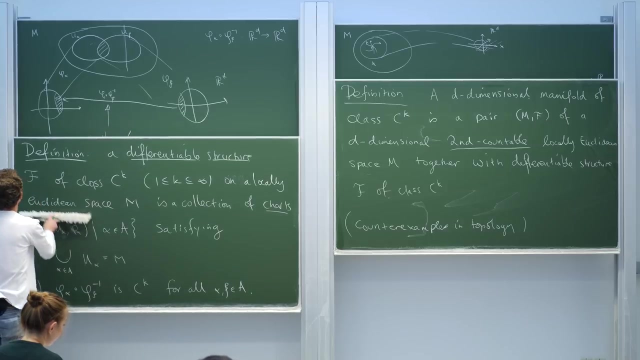 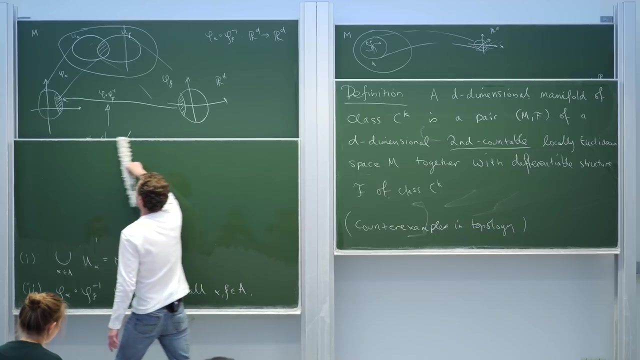 It's just absolutely mind-blowing what's in them. Thank you. So that's why it's second countable, because really bad things go wrong if it's not. But it doesn't matter, because for us, because, as I said, physics is about examples- 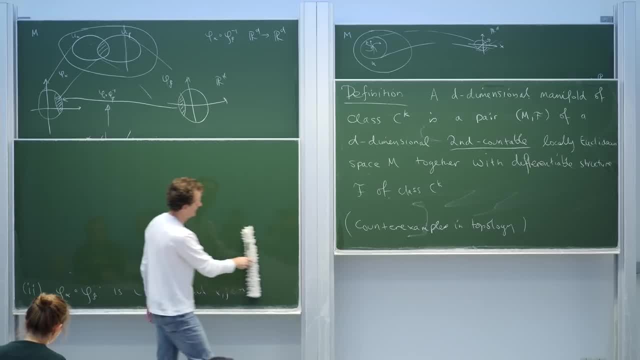 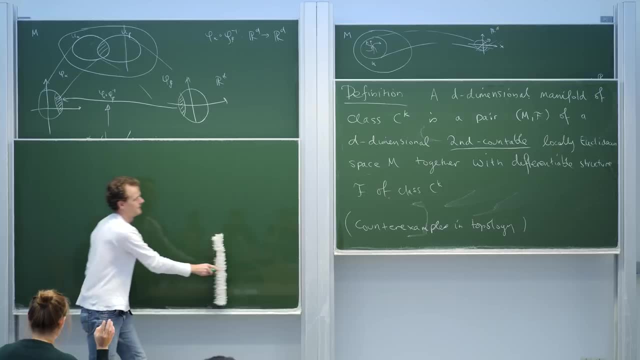 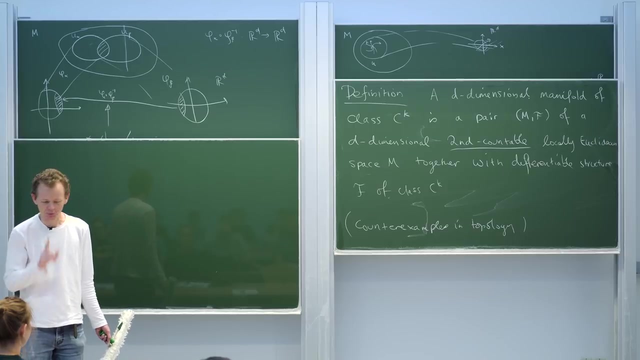 We know the Hamiltonian of the universe more or less. We don't need to consider all the different Hamiltonians, Yeah, Question: What does second countable mean? I don't remember is the short answer to that question. What does second countable mean was the question. 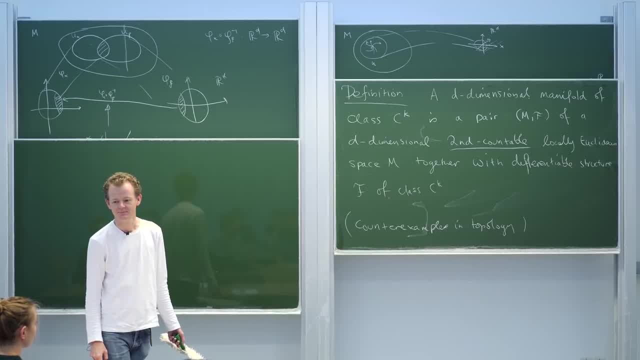 A finite. It's the one that says: 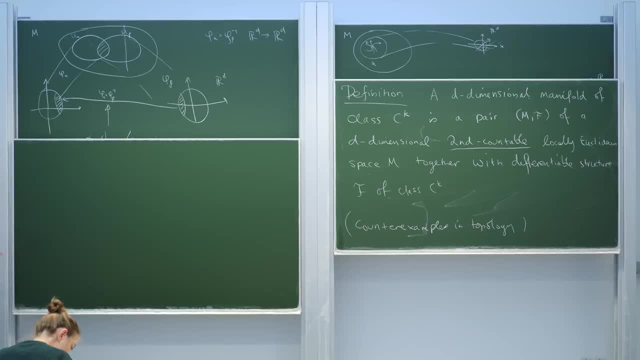 you put on them t0, t1, t2, t1 and a half and so on, and they're all additional constraints that you put on the definition of a topological space And I'm afraid I'd get lost somewhere. 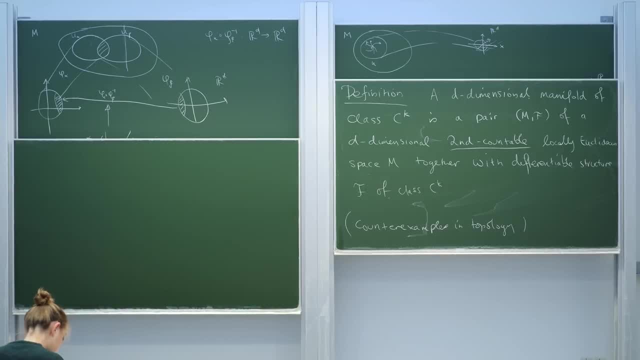 around the second countable point and have to look it up in the book. Now we can get to our examples. So, as I said, right, is it a good definition? Is it a bad definition? Well, it at least better capture that one example. 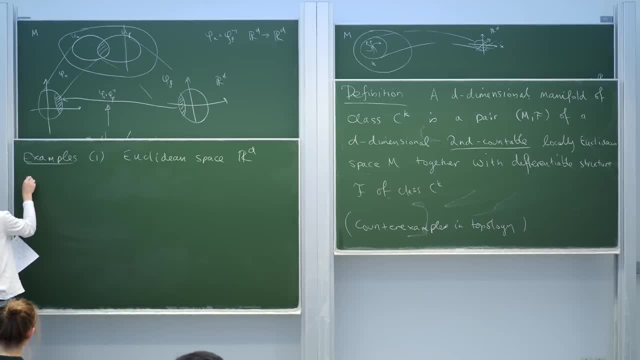 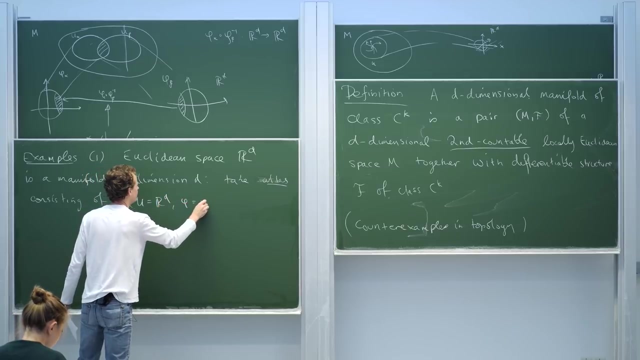 that we started off with, namely Euclidean space. Well, it is a manifold And it does actually have an atlas, a really simple atlas, the world's simplest atlas. Well, u equals r to the d and the map phi is the identity. 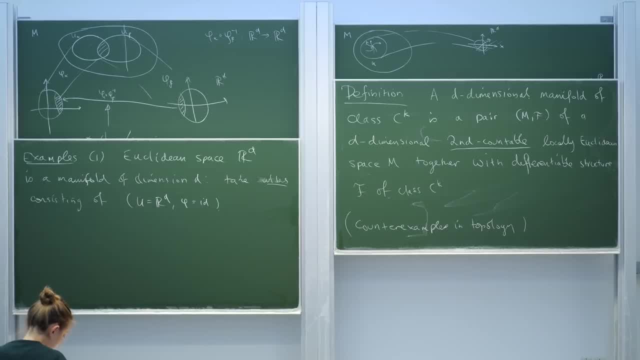 So that's a super good coordinate system for this space. Done, All right, it's a. And then you can add in all this stuff, The other charts, to make a differentiable structure. So good, This definition while a mouthful. 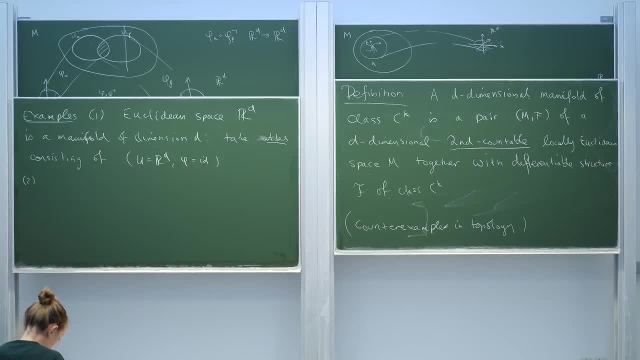 does capture the basic example of our course, Does it capture everyone's favorite second example, namely the Earth itself, the surface of the Earth, which is a sphere. Well, you can see, the whole terminology is adapted to this example. from this example, 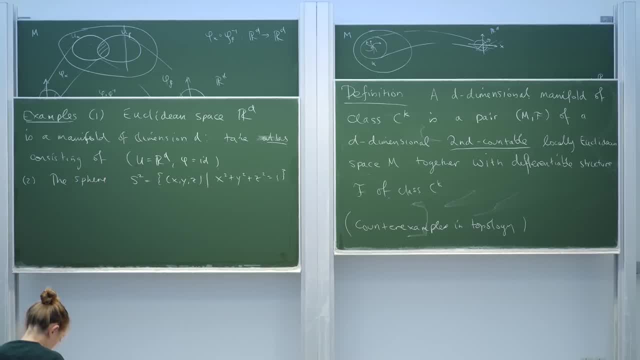 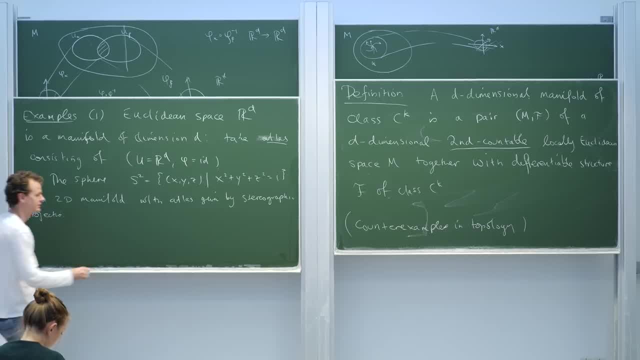 So there's an atlas given by stereographic projection. So you take the- This is r2 here- And Put the sphere underneath it And then you sit on the South Pole and then you draw a line through the sphere it intersects. 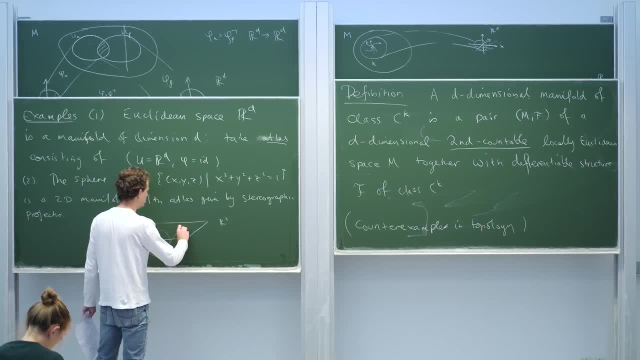 the surface of the sphere somewhere. and then you continue that line up to when it hits this R2, which is sitting on the North Pole, And so to every point except the South Pole has an image in R2 under this mapping. This is what we'll. 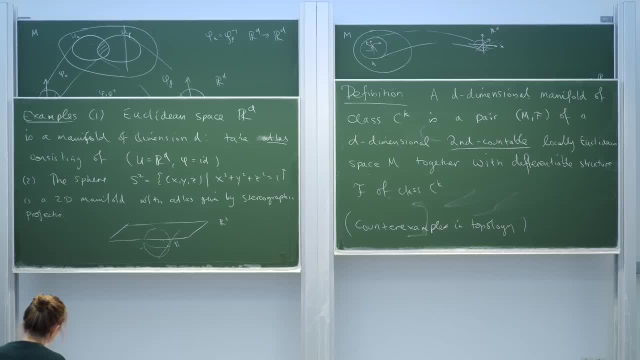 call Phi 1.. So that's a chart, right. You can check that it's infinitely differentiable, except at the South Pole. To make it an atlas, we need to be able to cover this sphere at least with one other chart and the second chart. 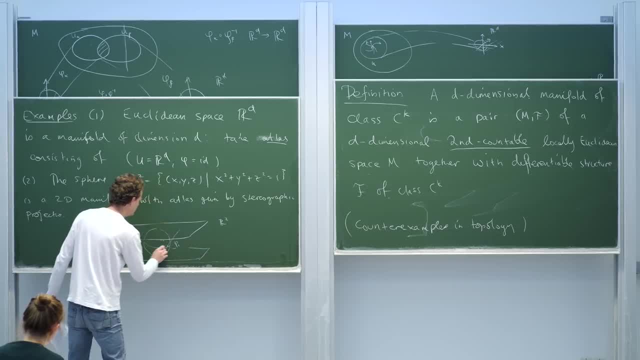 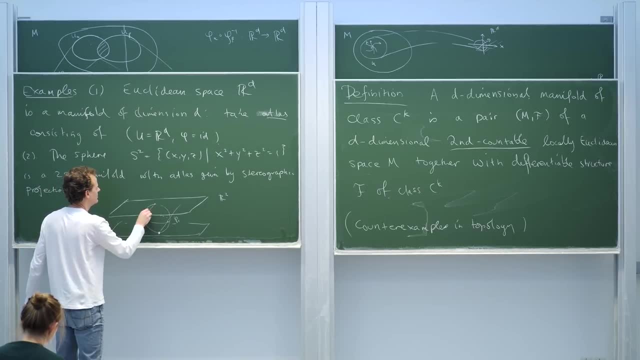 that we use is the same idea, but done from the North Pole. So I have a second chart, a mapping that goes: you stand on the North Pole, you draw a line through the sphere until it hits the surface and that point gets identified with where it. 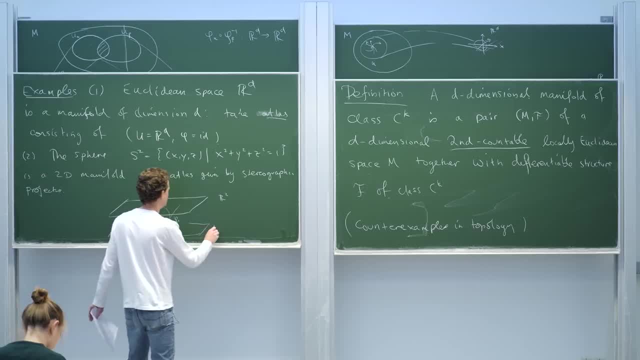 lands On the R2 on the bottom, And that's called Phi 2.. That's an infinitely differentiable map from the sphere to R2.. The sphere embedded in R3, as it happens, Because if I didn't say the word embedded then I would have said something. 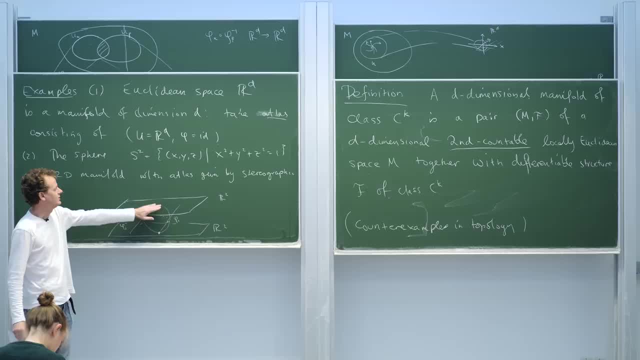 wrong, Because the only thing we need to check is that where these two maps have a common map and the other two maps have a common map and the other two maps have a common map, Because the only thing we need to check is that where these two maps have a common map. 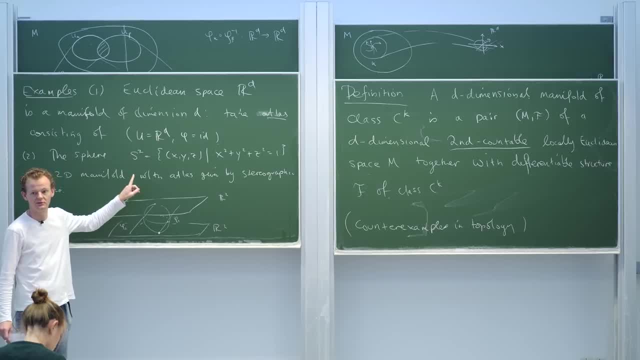 that the transition map is infinitely differentiable. The maps themselves need not be differentiable in any sense. In fact, to make sense of the word differentiability of such a map, we're gonna have to do a lot of extra work, But for this example, it's embedded in three-dimensional space. we can sort of 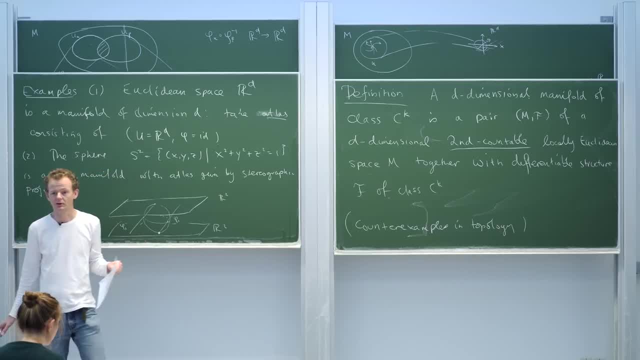 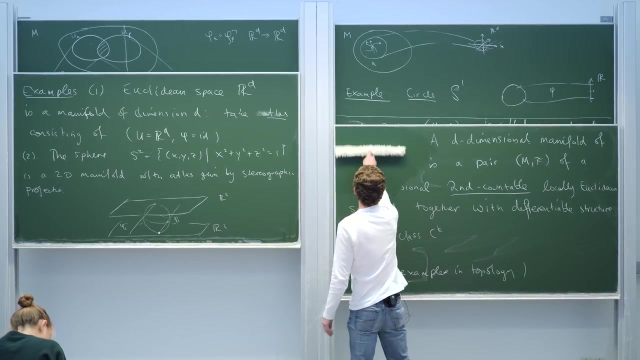 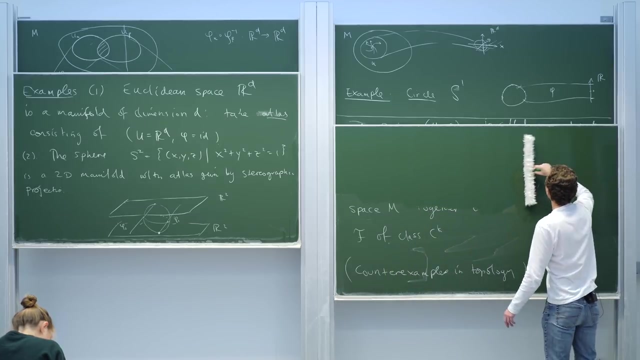 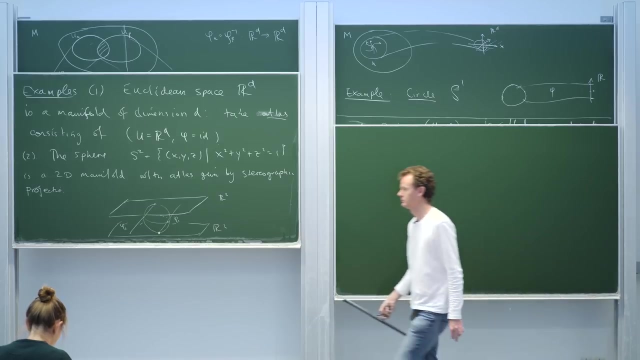 cheat, And this is an example. it's part of your exercise to work out that this is a manifold of class K is infinity. All right, Then in the last minutes I'll mention a couple of other examples. There we go. Let's choose some examples that apply more to mechanics. go through a couple now. 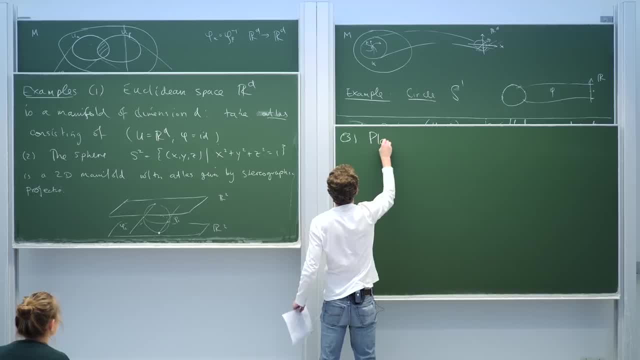 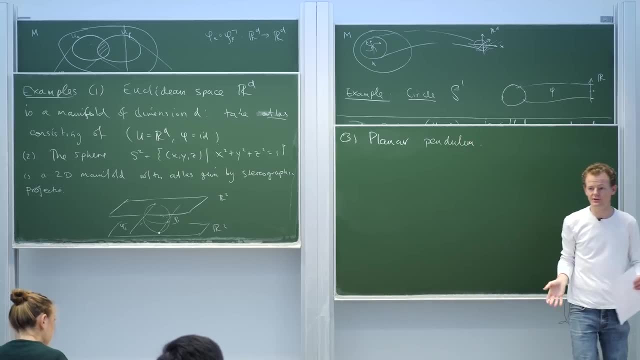 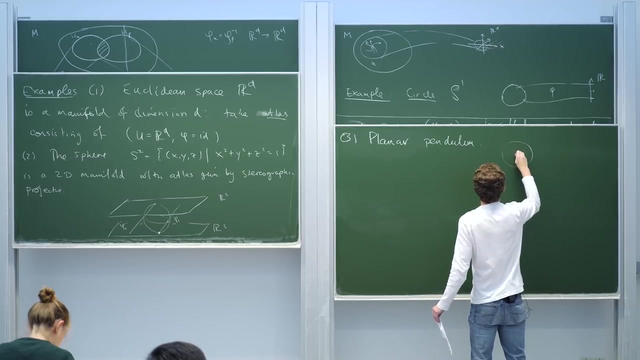 Planar pendulum. So the configuration space of a planar pendulum is a manifold. well, we've already done it actually. So if you have a planar pendulum, then it's with a perfectly a rigid, weightless rod and a mass, no friction. blah, blah, blah- all the conditions that you like. 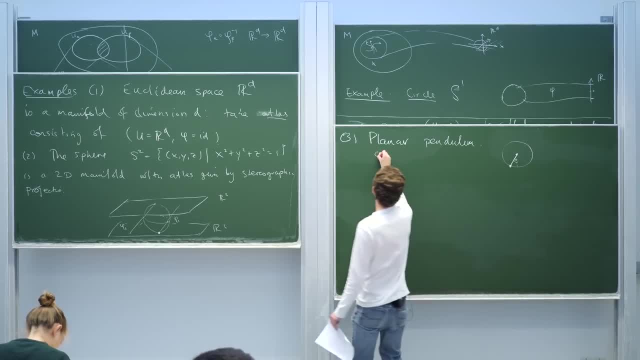 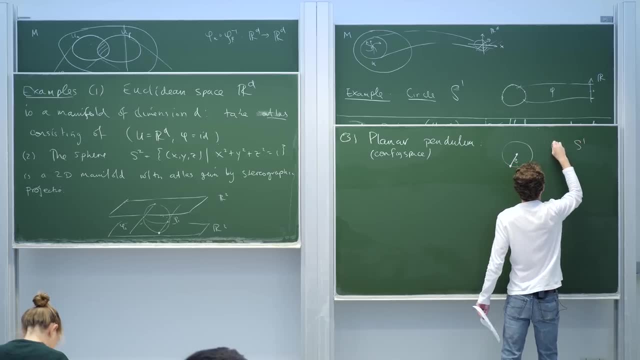 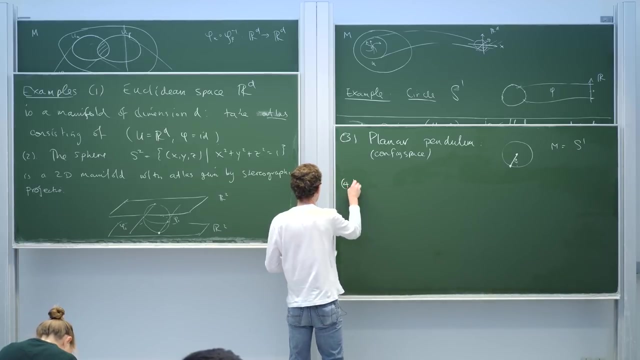 The configuration space of a planar pendulum is a manifold, and the manifold, of course, is just S1.. That wasn't too bad, Not too hard. Then the planar double pendulum. Its configuration space is well, not S1 but S2, S1, cross S1, the torus T2.. 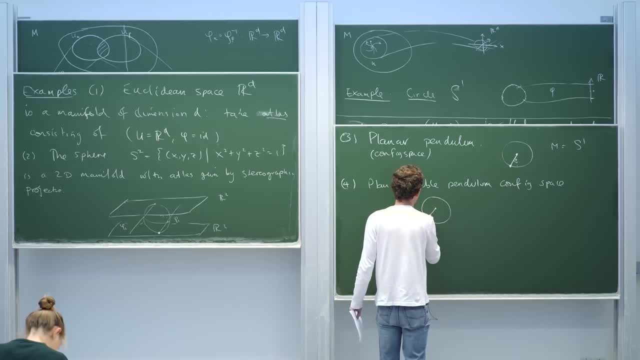 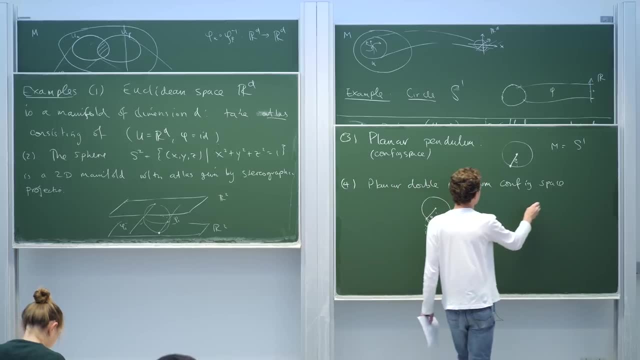 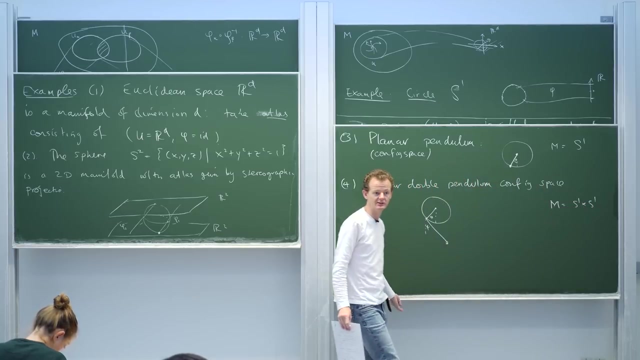 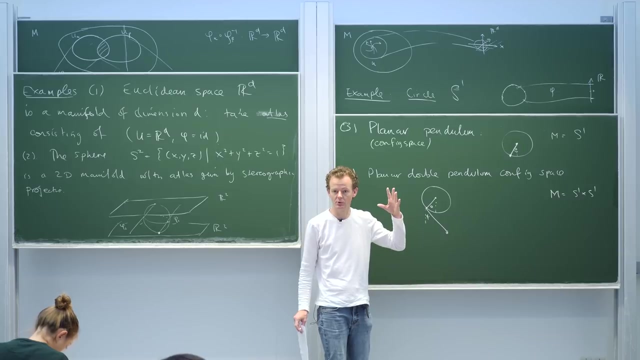 Okay, Okay. So I haven't proved that this is an infinitely differentiable manifold. That's your, that's an exercise for you, But once you see the sphere and the circle, then you can start to imagine, I hope, how those arguments work. 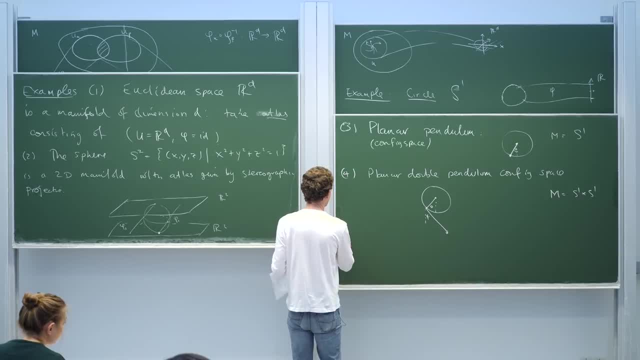 Okay, Ah, here's a sort of more interesting one. Imagine a dynamical system consisting of a rigid line segment that's stuck in the plane. So it's a little little piece of infinitely thin. it's an infinitely thin rod of some. 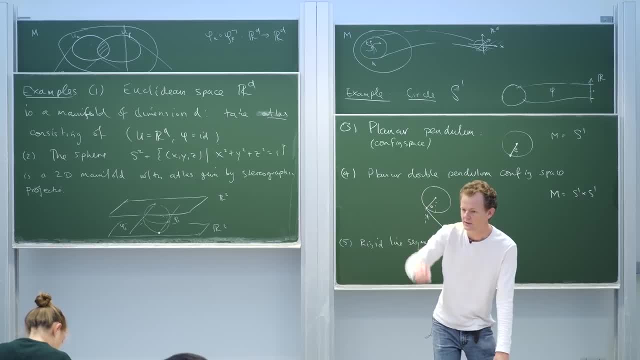 finite length in the plane, like this piece of chalk Right And then on the plane. how many coordinates do you need to specify the configuration of such a thing? Any takers? This looks like a coordinate. That looks like a coordinate. 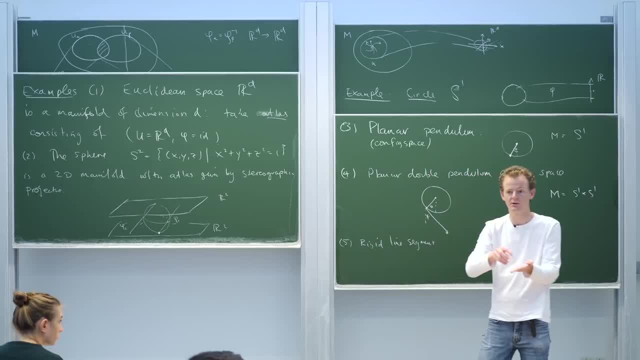 Is that enough? Two, Four, Four coordinates is one answer. Do we need four coordinates for the rigid line segment in the plane? Well, we definitely need everything, Okay. Okay, So we need x and y, It's two. We also need rotation. 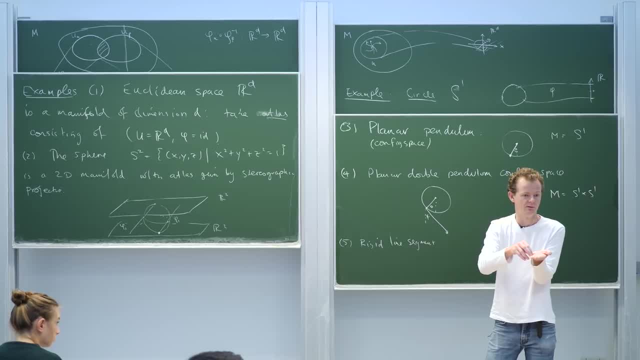 So that's a third one, But I think we don't need a fourth one, Because you're right in that to specify both endpoints would require four. Right, If you have a rigid line segment, you could specify it with four coordinates, namely the: 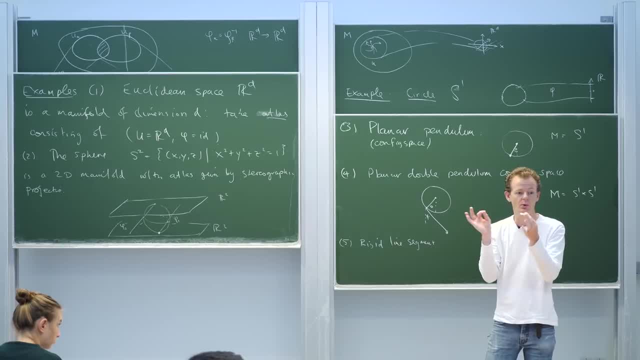 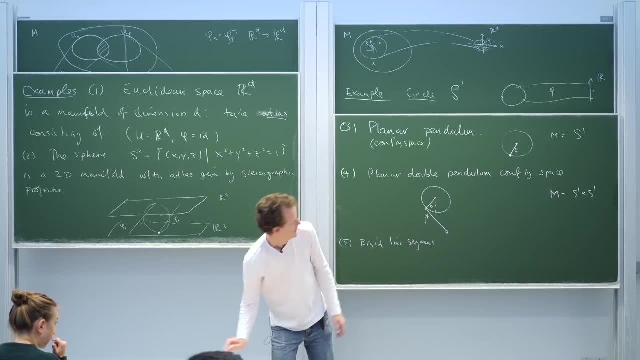 coordinate of this end and the coordinate of the other end. But there's an equation of constraint here that the points are always a certain distance apart, So that cuts it down to three. Okay, So the rigid line segment, the configuration space M is actually equal to R2, the plane: 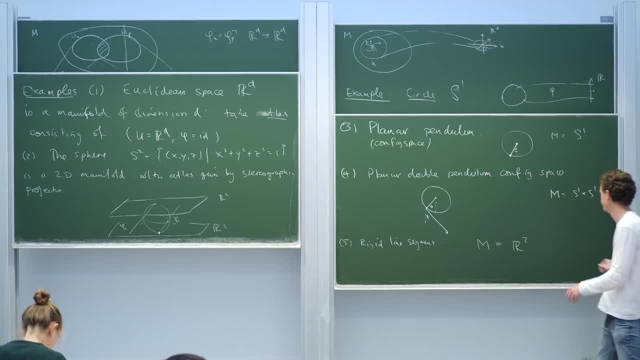 its coordinates of one endpoint in the plane plus a rotation. That's a manifold. Actually the quantum theory of that is not that far off the quantum theory of strings. So these kind of manifolds they look a bit trivial but they can get rapidly very, very. 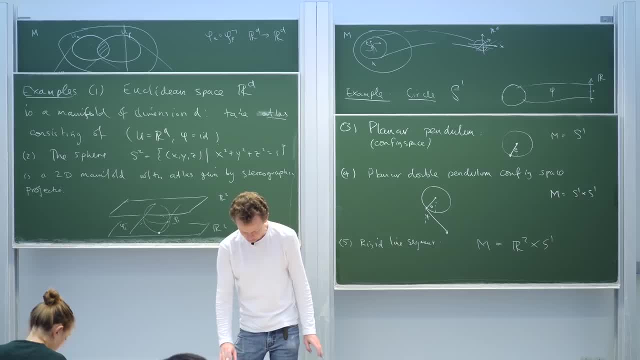 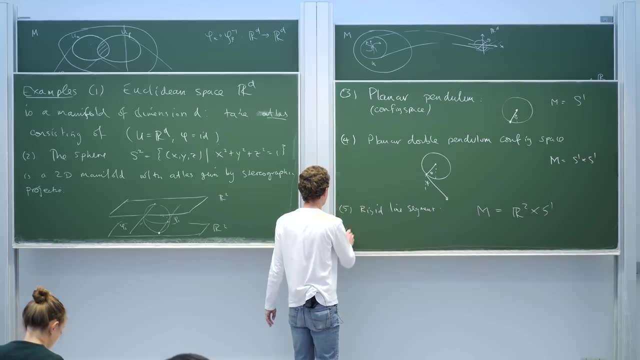 very complicated. Do I have any more examples for you today? No, Okay, Okay, All right, I'm going to give you a sixth one. Hilbert space is a manifold. It's a bit weird: You don't usually think of Hilbert space as a manifold, but it is. 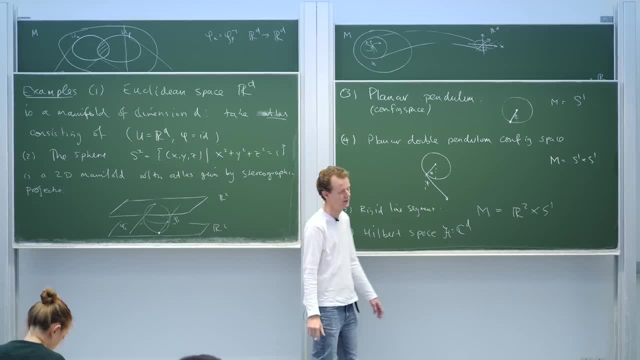 And actually it's a Kehler manifold. That's something that we may or may not see in this course. Okay, Which means that it's a symplectic manifold And that's why quantum mechanics. it's sort of an underappreciated fact. why quantum mechanics? 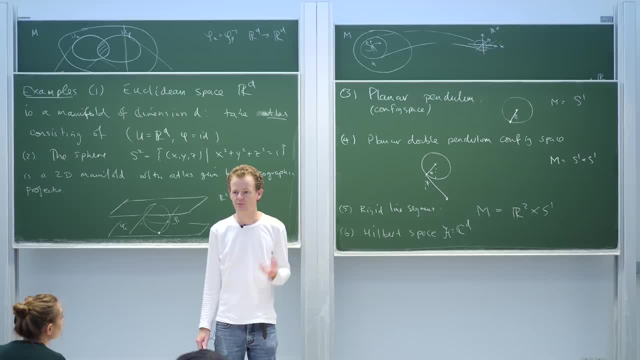 itself is symplectic, is covered by the formalism of symplectic geometry. so at least in finite dimensions. Hilbert, space of an infinite dimensional system, that is a manifold, but it's an infinite dimensional manifold And we're certainly going to stay away from those in this course. 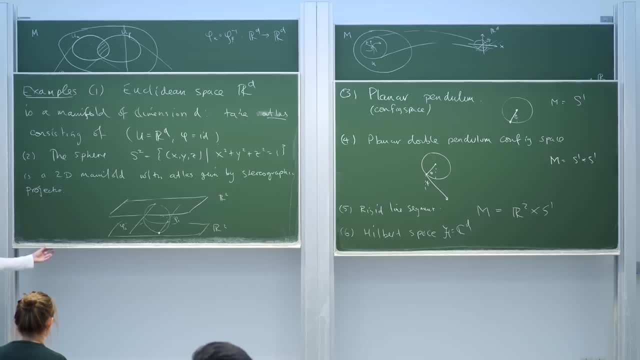 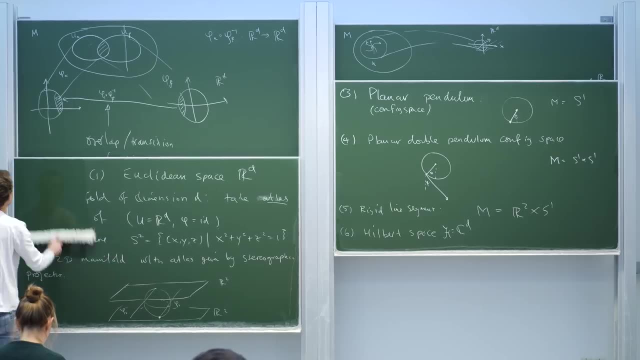 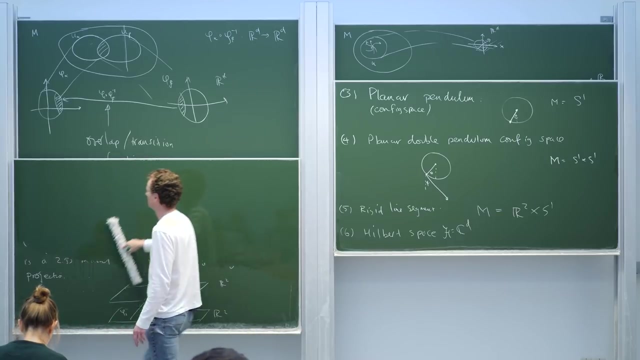 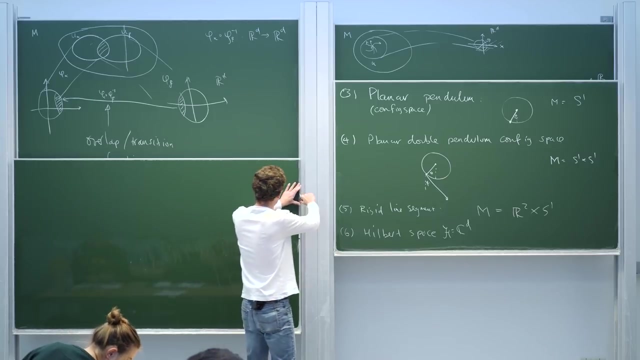 Although, to be fair, a lot of what we'll deduce will be just simply true for the infinite dimensional case. I want to end with a nice way to construct examples, And really this is the way I I. I think this is the way most people think about manifolds. 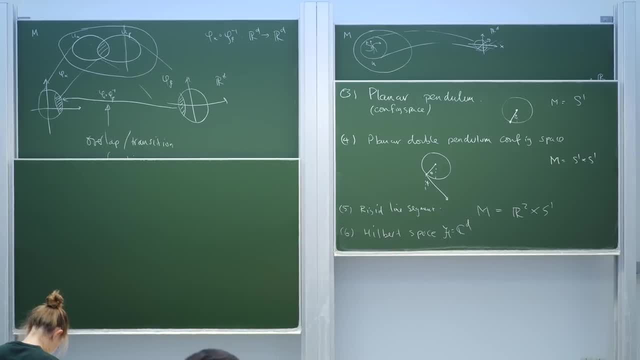 anyway, right. So this is a, this is aennenium manifold, It's a manifold manifolds anyway. So there's this lovely abstract definition here locally: Euclidean space, homeomorphisms, transition functions and so on. But really, you know, if we're 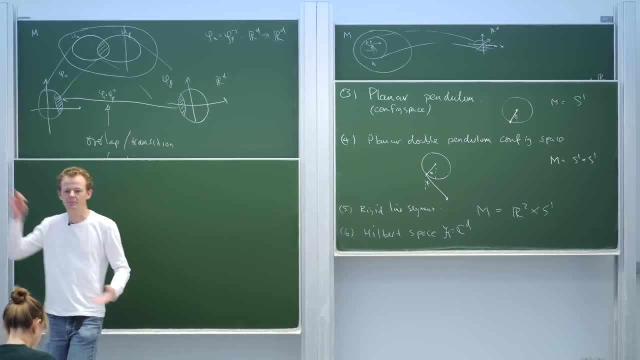 brutally honest, the way we work with manifolds is we usually find some bigger space which is clearly like Euclidean space, and then we realise our manifold is some surface, some embedded space, And then, like, all this abstract stuff isn't really. 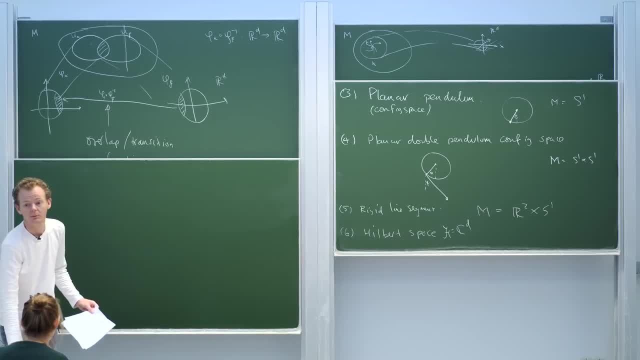 necessary. you just, you know, do your usual Euclidean thing, but with some constraints. You know, it's pretty rare that you have to worry about Klein bottles or Möbius strips- in physics- Pretty rare. It is possible these things come up occasionally. 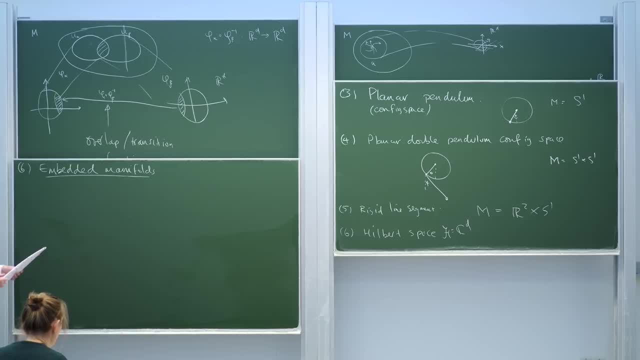 But usually the manifolds in physics we care about are actually embedded, actually live inside something else. So you know if you're going to do something like you know you're going to do something like you know you're going to. 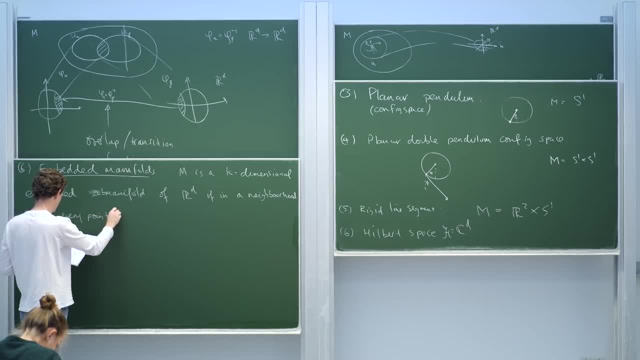 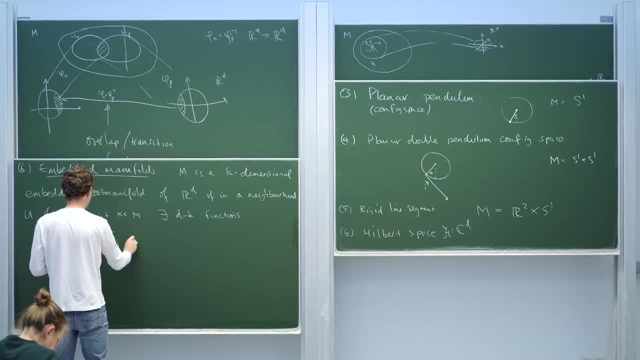 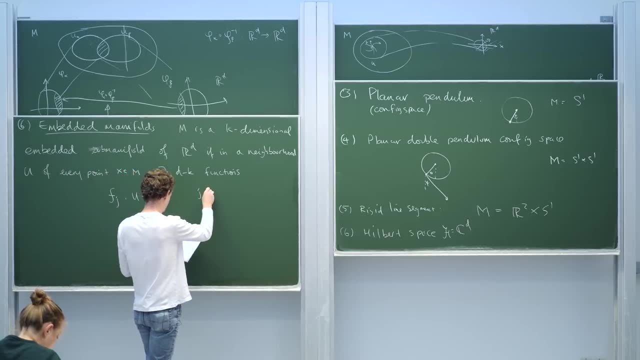 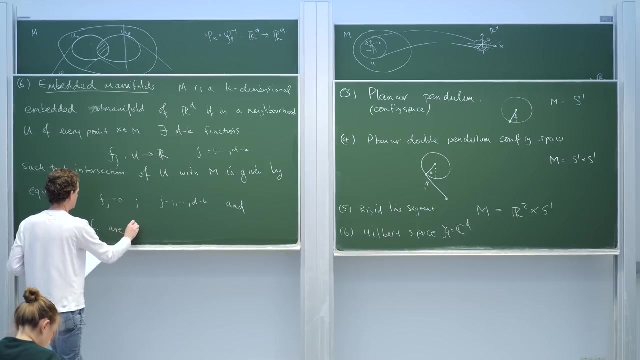 know you're going to do something like. you know you're going to do something like: Because there's that kind of constantка that's going to come up again and that constant thing still there in its Thank you. All right, this is a ready source of examples. 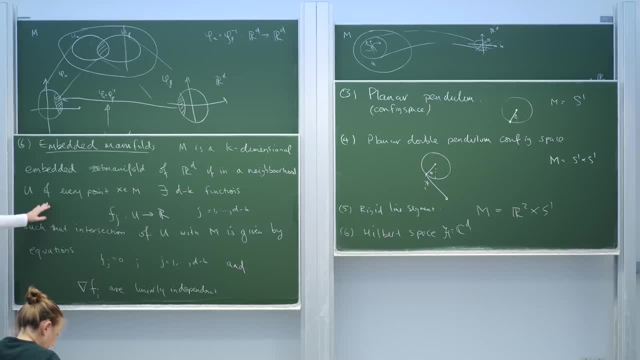 Pretty much all the examples we cover in this course will be really embedded manifolds. What are they? M is a k-dimensional embedded submanifold of Euclidean space. if in a neighborhood, in a small neighborhood, in a small region, around every point in your manifold, 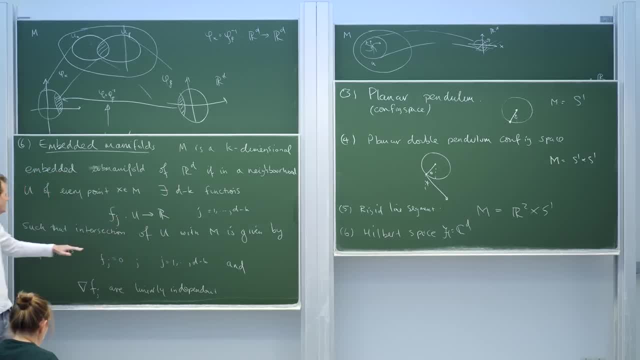 there's a bunch of functions which vanish on your manifold. That's not enough. You also need that the gradients of these functions are linearly independent. That stops some nasty counterexamples coming in. You'll see that as well in your assignment sheet. 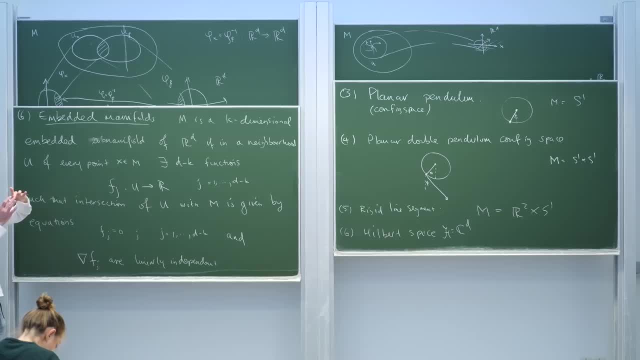 And what's a perfect example of an embedded manifold? Well, a circle. A circle's an embedded manifold in R2.. It satisfies this one equation, which is 0, namely x squared plus y squared minus 1.. 0 on the manifold. 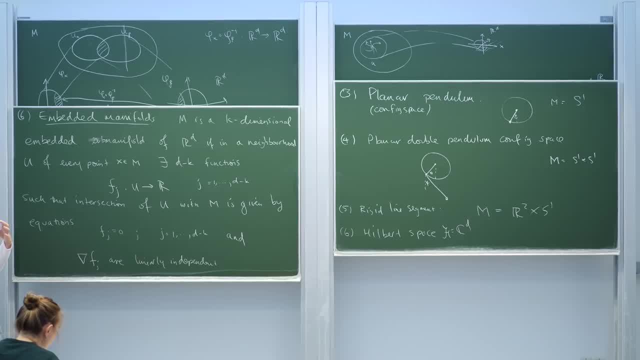 The sphere is an embedded manifold. It's what you get when you restrict in R3 to points which obey the constraint that x squared plus y squared plus z squared minus 1 is 0.. But you can come up with crazier examples. Take the intersection of: 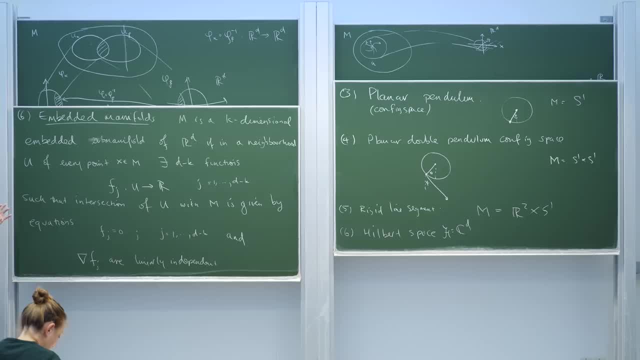 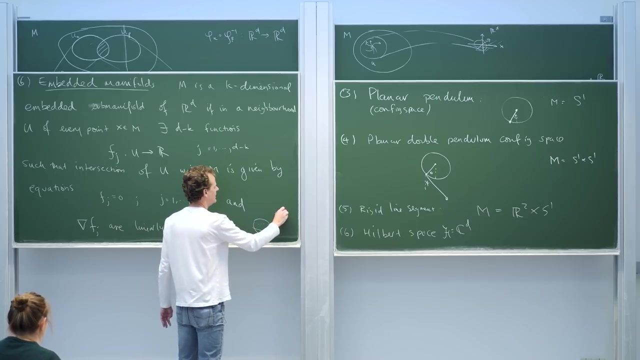 say the sphere with a paraboloid. There's two equations now that define that And it's some curvy circle. Try and draw that. That's one equation: f equals x squared plus y squared plus z squared minus 1.. 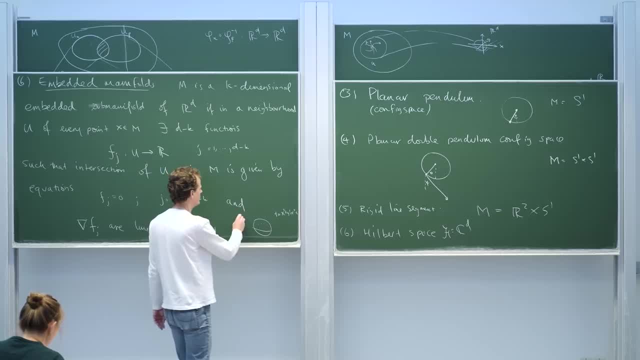 That's the equation that vanishes on the surface of the sphere And then you want to intersect it with a paraboloid. say: That's the second equation. Let's call that z minus x squared minus y squared. That's the second equation defining a paraboloid. 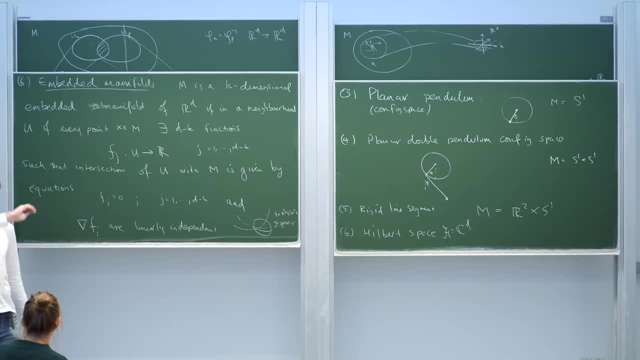 The intersection of these two things is some slightly curvy. No, in fact it's just a circle, isn't it? It's not even a curvy circle, It's just a circle. So that's an embedded manifold as well. 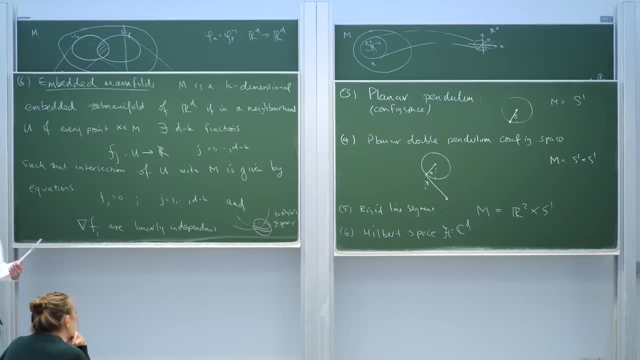 All right, I think that's all Yep I want to say today. Thank you very much.